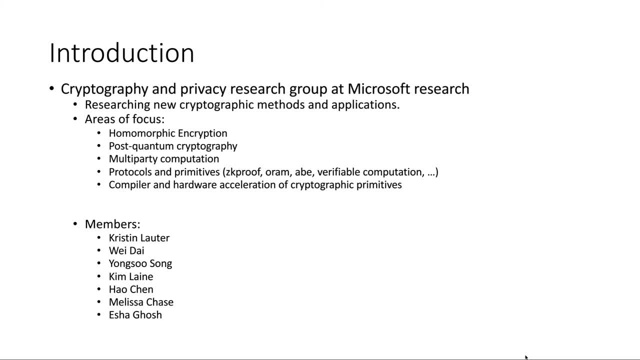 so that we get to learn more about each other and potentially in the future we can have some opportunities to collaborate. So we are the Cryptography and Privacy Research Group at Microsoft Research in Redmond and our task, the major goal, is to research on 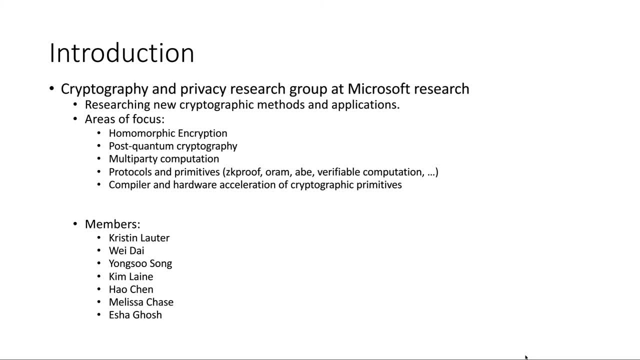 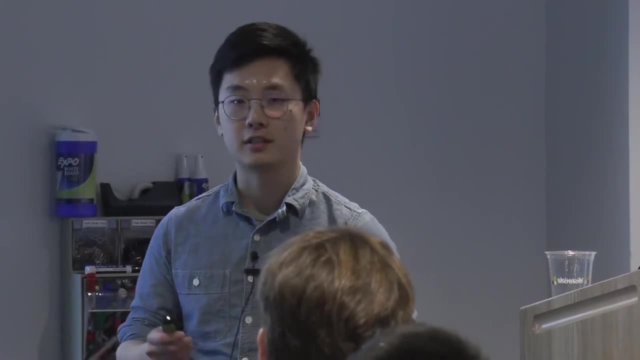 the new cryptographic methods and applications and we have developed several focuses along the years and right now we have these several areas of focus, which includes the homomorphic encryption, multi-party computation and some other protocols and primitives. we are interested in Zero-knowledge proofs, ORMs. 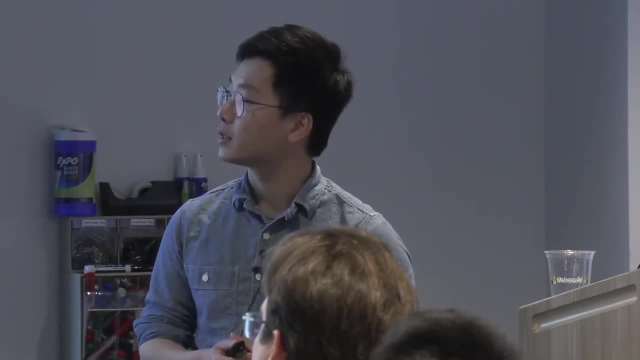 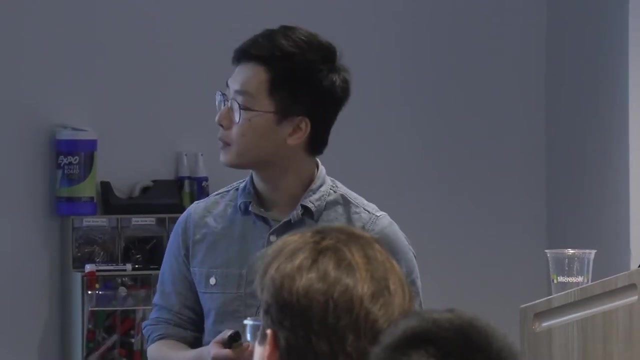 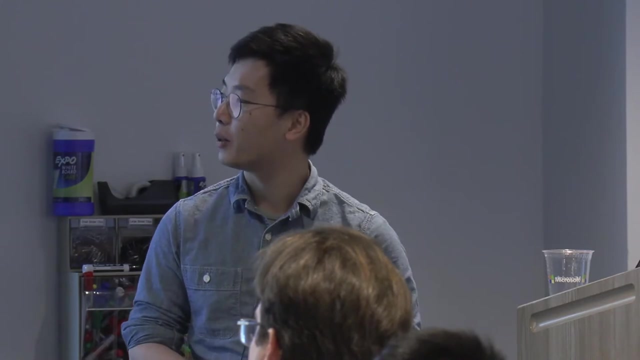 attribute-based encryption and et cetera. We also like to work on things like compiler and hardware accelerations for the cryptography primitives. Currently, our group consists of- I think it's- seven members. So Christine Wei Yongsu Kim. 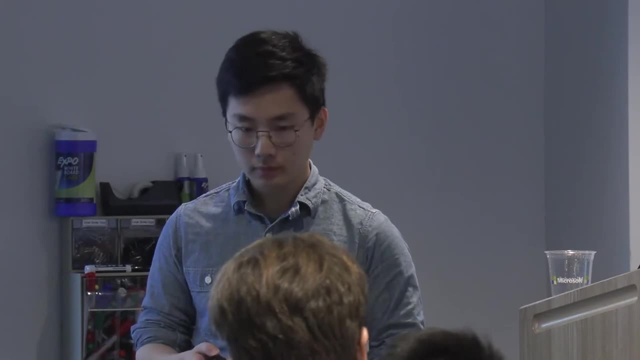 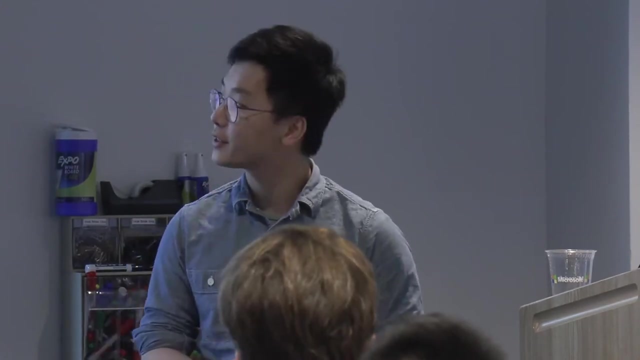 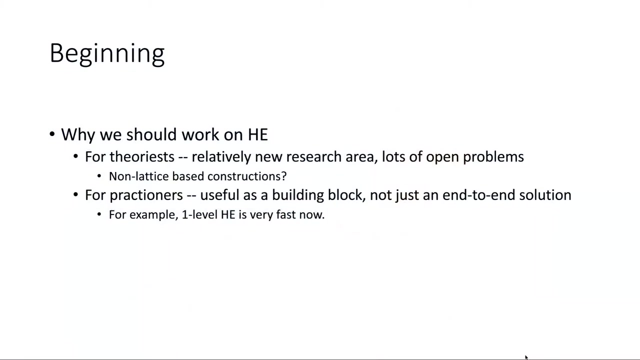 myself, Melissa and Asha. So you can learn more about our group on the MSR website and also feel free to chat with any of us. Okay, So, and also maybe just to motivate the talk, I wanted to talk a little bit about why. 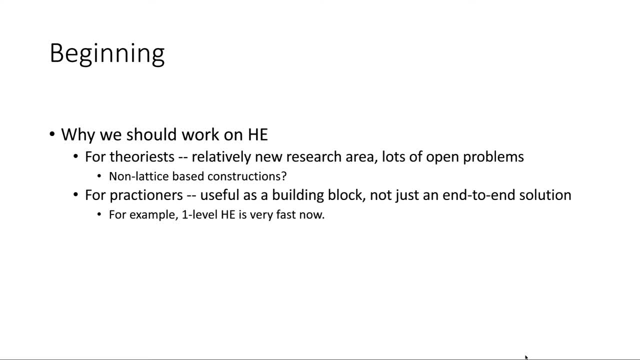 I think that we should work on HG. Well, I don't know if you need such a motivation because you're already here, But I guess for me. I think HG is interesting area to work on for various reasons, But just to highlight two of the possible reasons: 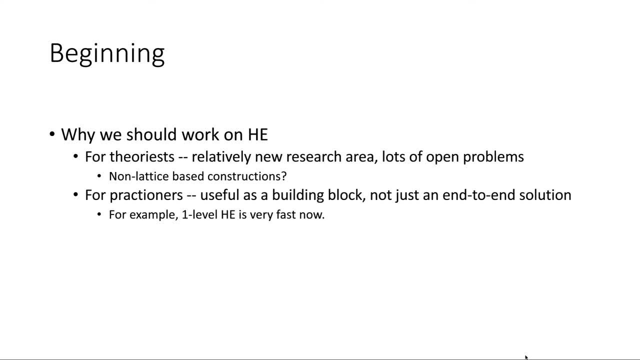 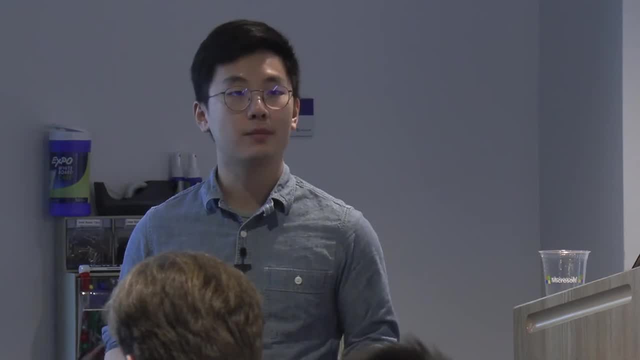 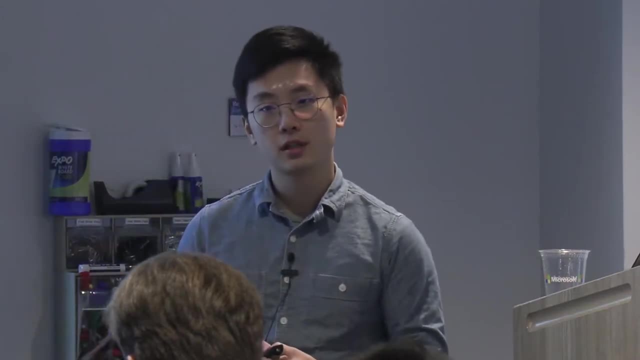 First of all, it is still a relatively new research area and there are many open problems that there are still to be solved. Just for example: right now, all the most efficient HG techniques are based on the lattice assumptions. Lattice assumptions, right now that people believe that. 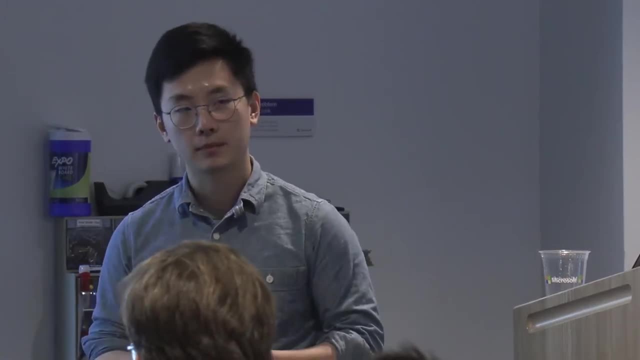 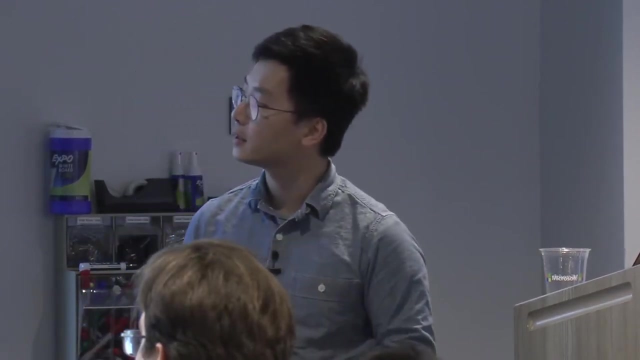 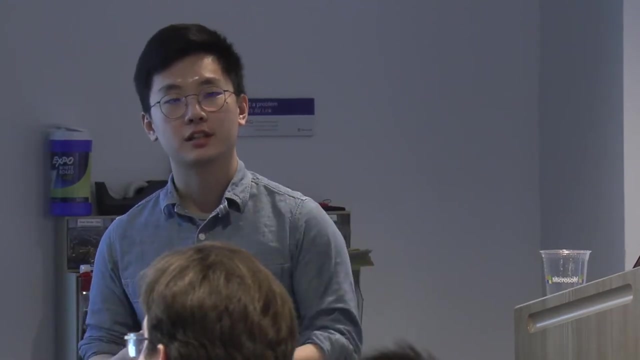 it's post-quantum, but we actually don't have any efficient constructions that's not based on lattice. I think that's something interesting question to think about, Also for the practitioners in the audience. I think HG has this reputation of being inefficient. 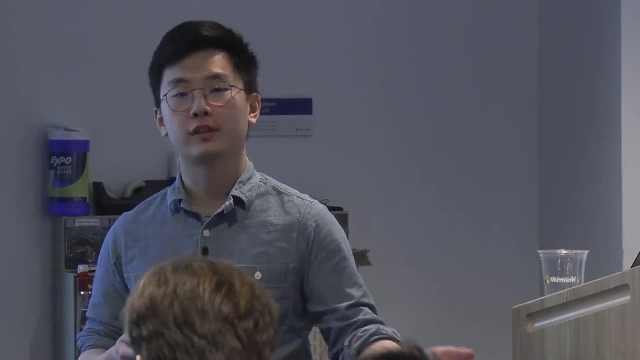 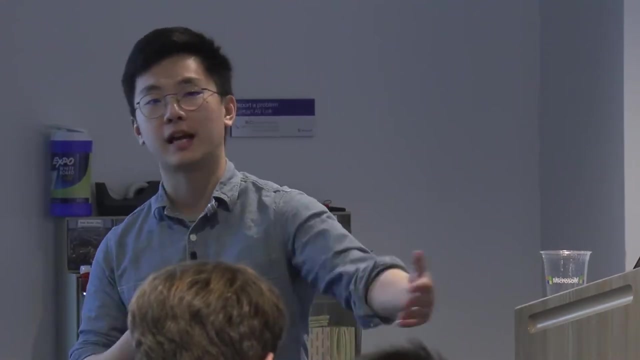 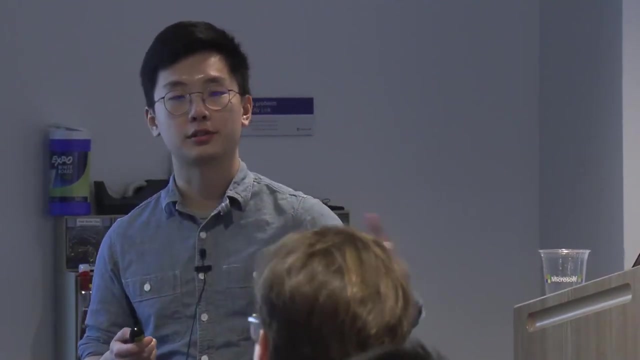 But actually I think over the years people have proved that at least it can be efficient for certain computations. So even though maybe you're thinking of building an end-to-end solution which has some privacy guarantees, HG might not be the sole solution to this problem. 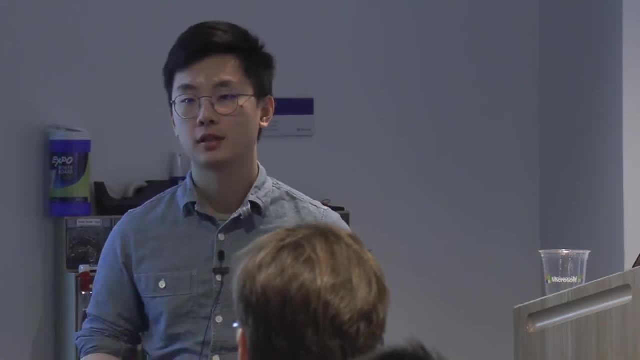 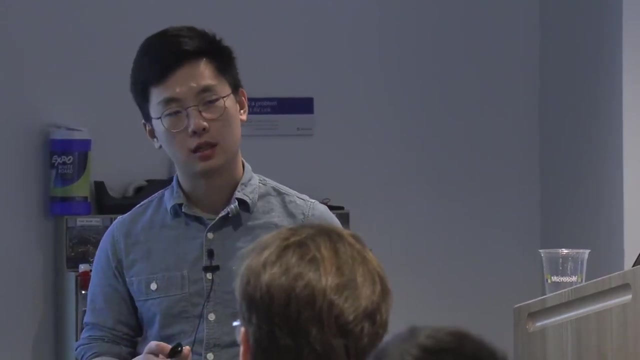 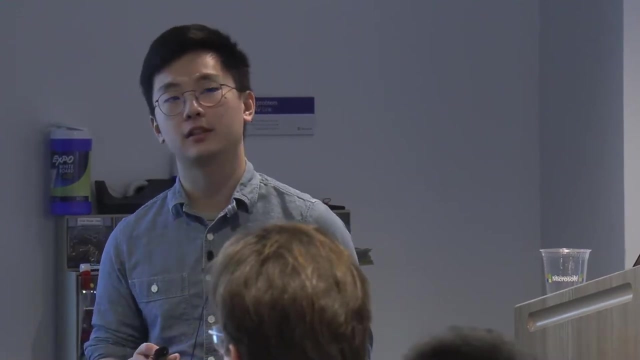 but you can somehow use it as part of the solution. So, for example, if we use this currently best lattice-based HG technique for the linear operations as a substitute to the classical additive homomorphic encryption systems, then it is already very fast and overhead is low. 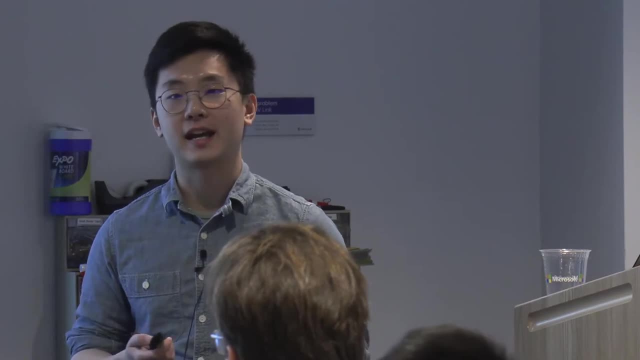 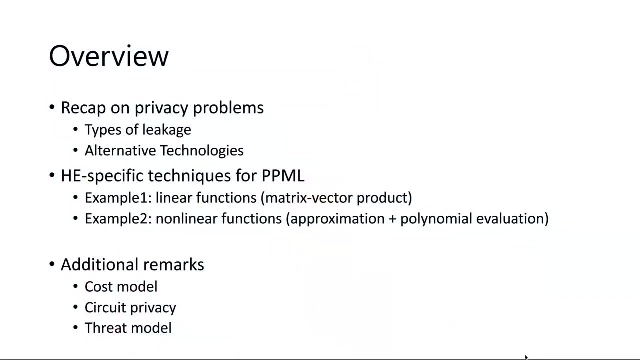 So actually it can be used today as an efficient solution. So I do have an overview of the talk. So I will talk very briefly about some of the different techniques of doing the PPML. but I will just pass through that very quickly because I'm not an expert in those fields. 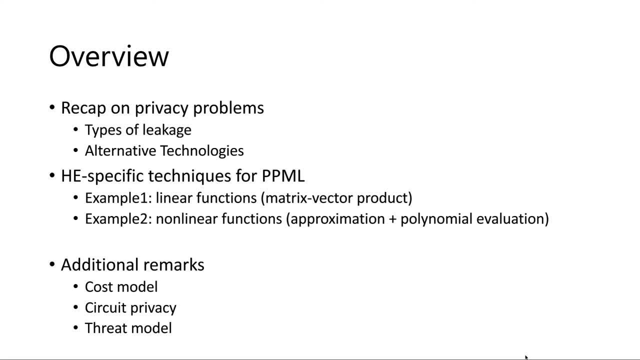 Then I'll go to the HG specifics, maybe just go through some examples of how we would go about building some applications which does some machine learning over encrypted data, and what are the challenges and what are some of the algorithms or improvements that we made. 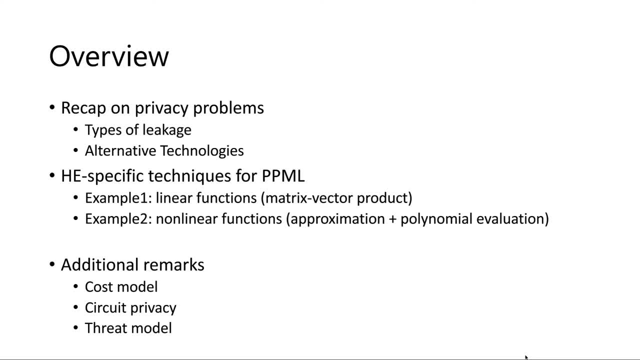 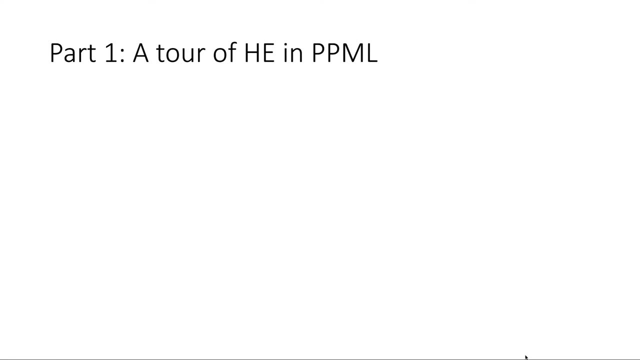 Then, in between these topics, I'll try to make some additional remarks or like short tips about what we should think about when we are building these solutions. Okay, So I thought a little bit about. when we talk about leakage in the machine learning, what are we talking about? 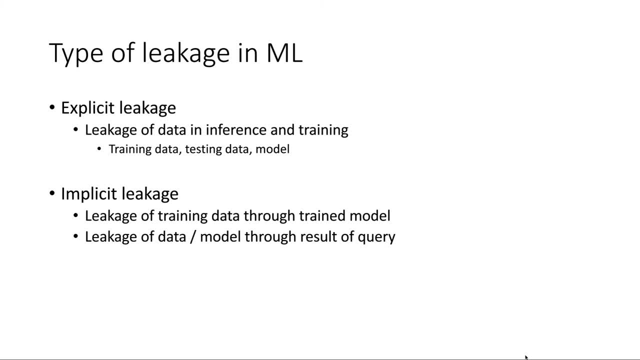 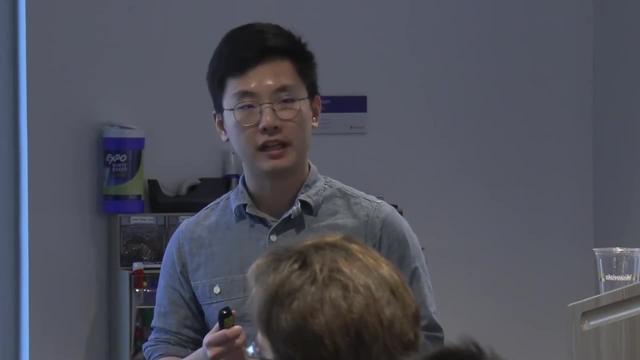 And roughly I think we can classify these leakages in two categories, But if you have some other opinions, let me know. So there's this explicit leakage in the machine learning where, for example, if some company is collecting all its users data to train certain machine learning model, 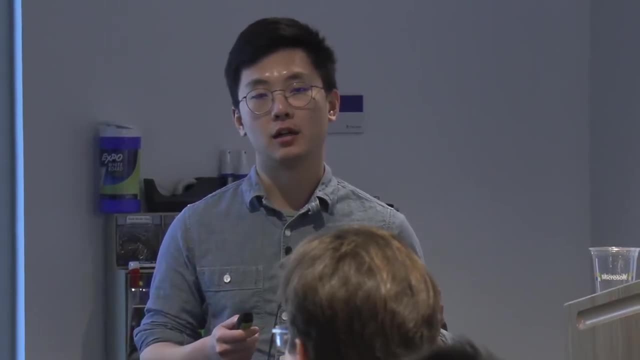 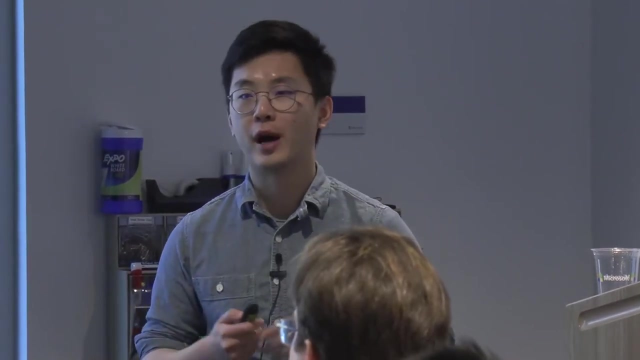 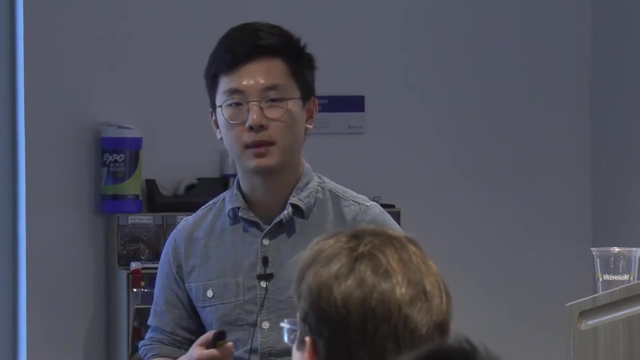 then this data is supposed to be known to this company. So you're in some sense, just directly contributing your plain text data to whoever is running the machine learning algorithm. When you're doing inferencing, for example, if I'm submitting my whatever kind of data, 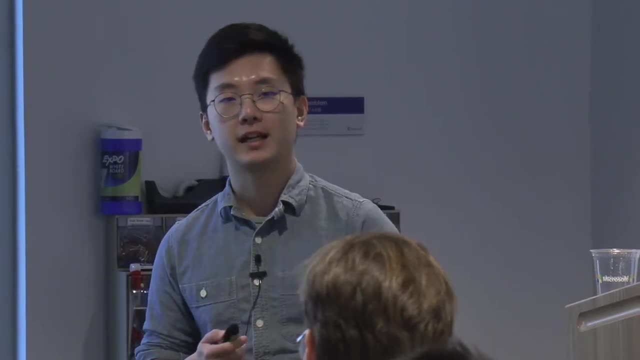 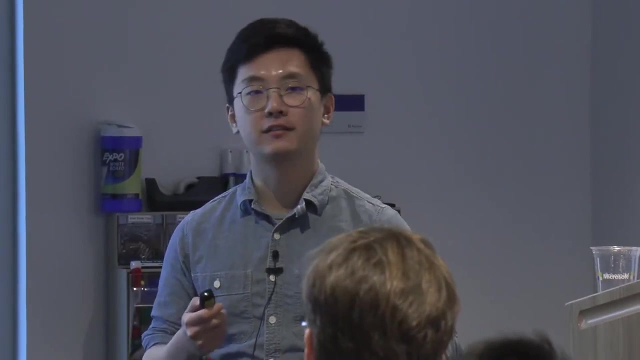 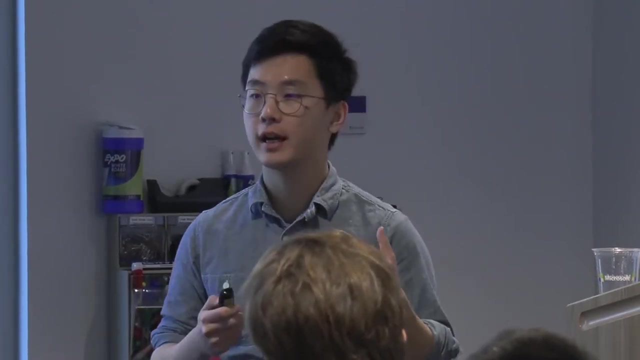 for example, it could be medical data, it could be genomic data or it could be something like what kind of movies or books I like. That kind of data for inferencing is also directly learned by the service provider. There's also the model leakage where, for example, 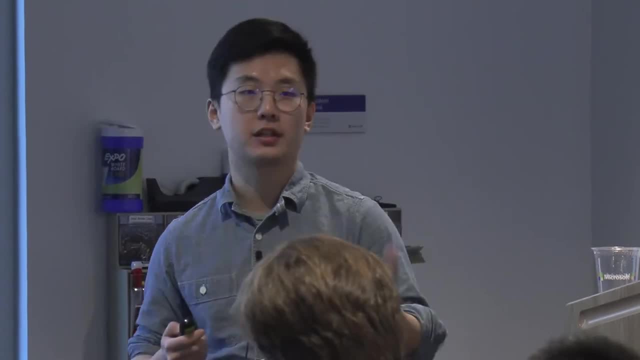 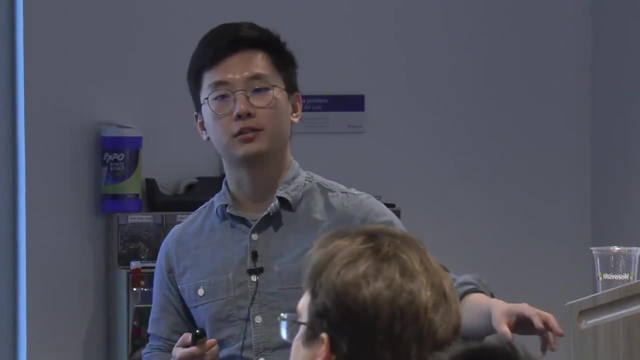 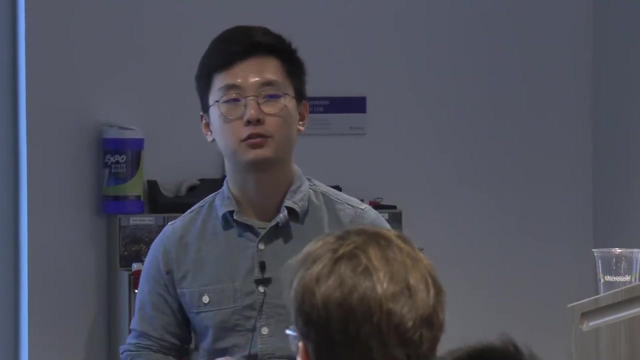 in some of the scenarios for machine learning, for example federated learning, you might have heard that the service provider actually deploys a model to the user's device, So in this case you must ensure that the model itself is not leaking too much information about the training data, for example. 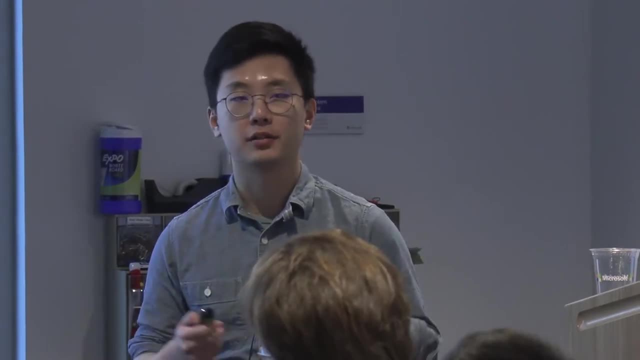 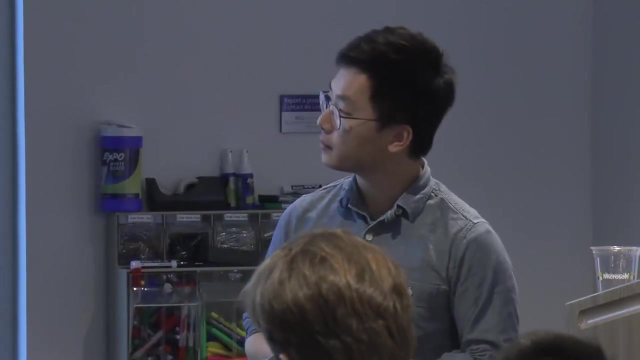 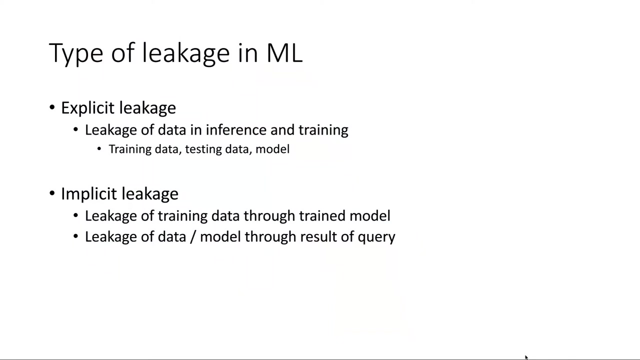 In a lot of the cases also, the model is considered valuable asset, so you may not want to leak it to anyone else. There's also implicit leakage in the machine learning, where I can give two examples. First of all is that I think many of 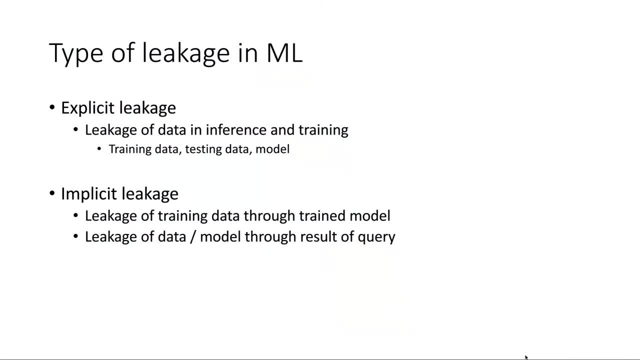 you also have worked on or heard about adversarial machine learning, So in those cases it's possible that the final model leaks some information about the training data. So this is not explicit in the sense that the model doesn't just directly output part of the data. 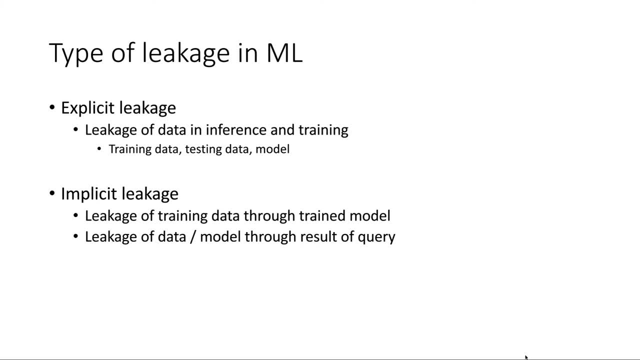 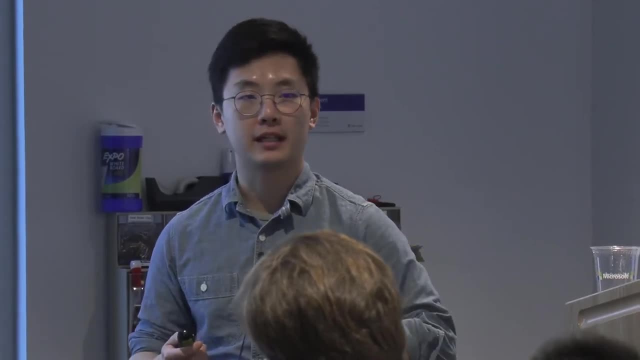 but you can often infer some information about which data is used in a training process. Another kind of implicit leakage is when you think of inferencing and someone is making a lot of queries to a certain machine learning models. You know that if the model is simple enough, 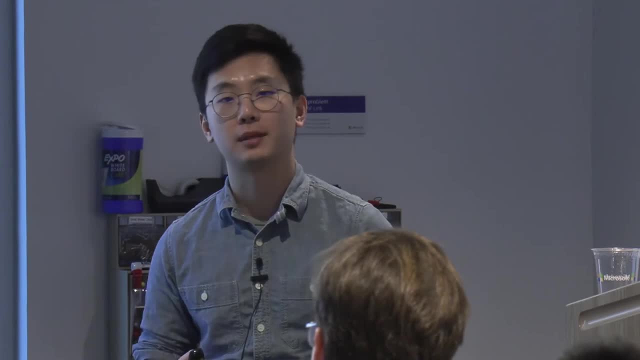 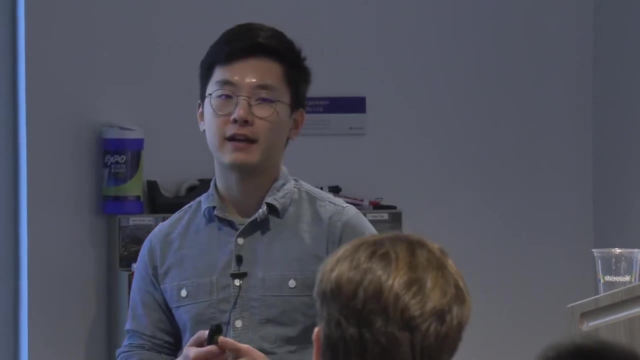 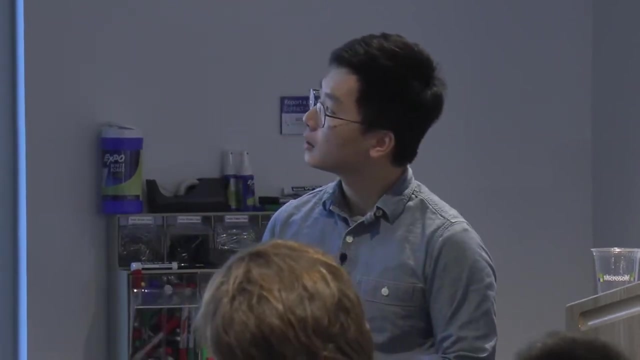 then, by making enough queries, you can actually just reconstruct the model. So this kind of leakage is not explicit, but it's implicit in the sense that every time you make such a request you are learning some function of the sensitive data With these types of leakage in mind, 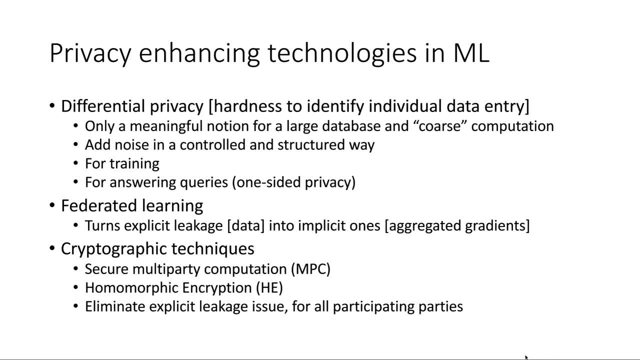 we can talk about the different kind of protection mechanisms. So I have listed differential privacy, federated learning and some cryptography techniques. So for the differential privacy, we can think of it as a meaningful notion of privacy for large databases and for coerced type of computation. 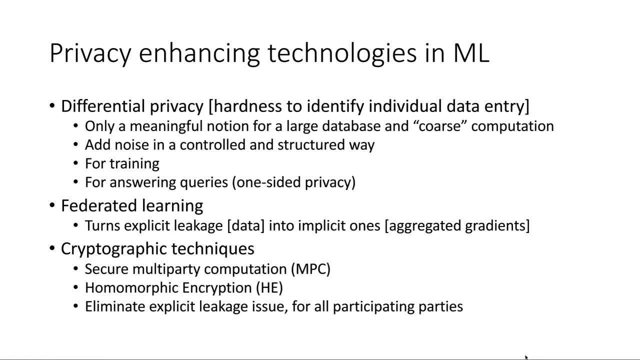 For example, it could be that the database is a long list of numbers and we're trying to get some kind of histogram or the top 10 of all the numbers. So in this case, the technique is to add some noise in a structured way, so that the final result of 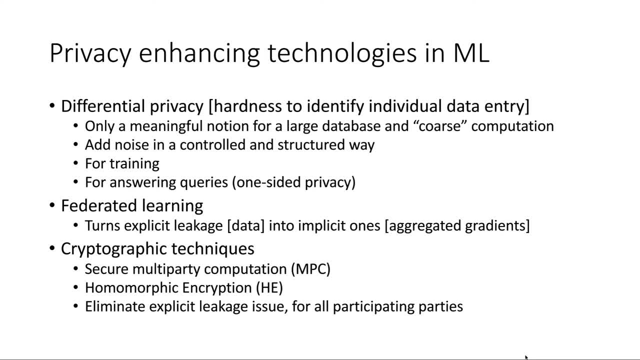 the computation doesn't let you identify whether a given individual is in this dataset or not. So this can happen in training, For example, I can deploy differential privacy, which makes the guarantee that just from the trained model nobody can identify whether a certain person's data is used in the training. 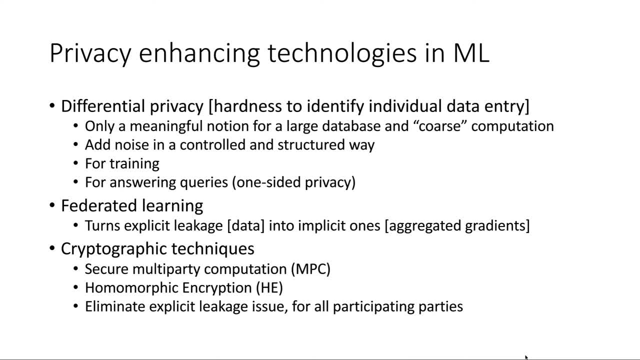 Also for answering some simple queries, where the guarantee now is that from the answers to the query I cannot learn too much about the underlying database. There's also federated learning, which turns this explicit leakage of a user's data into some implicit leakage where, if you think about how the data 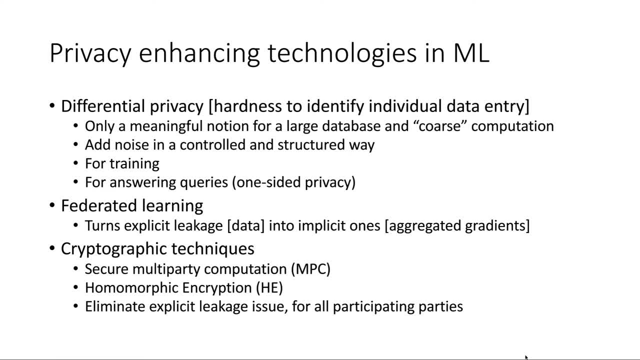 contributes to a machine learning model. in the training you actually use this data to compute some functions on them and then you use these- maybe gradients- to update your models. So for the federated learning you take a lot of users and then you average. 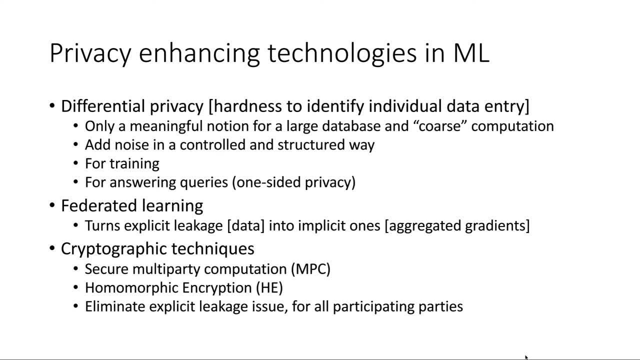 their gradients in some way so that only the service provider only sees this aggregated gradient, which supposedly doesn't leak a lot about each individual user's data. But put it in another way, it turns this explicit leakage into an implicit one, but it doesn't close the door of 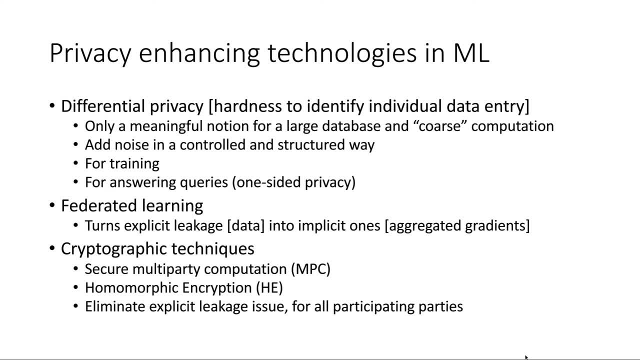 all the possible inferencing attacks, Then the techniques that I'll be focusing on today will be the cryptography techniques, So this includes the multi-party computation and homomorphic encryption. So these ones will eliminate the explicit leakage where, when you're doing training or inferencing, 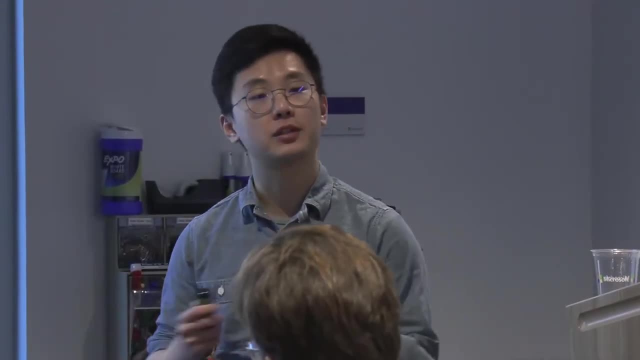 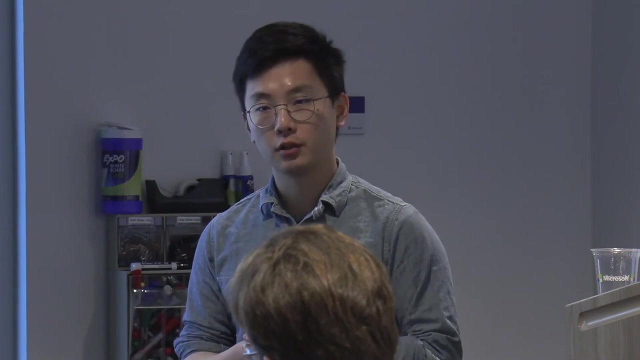 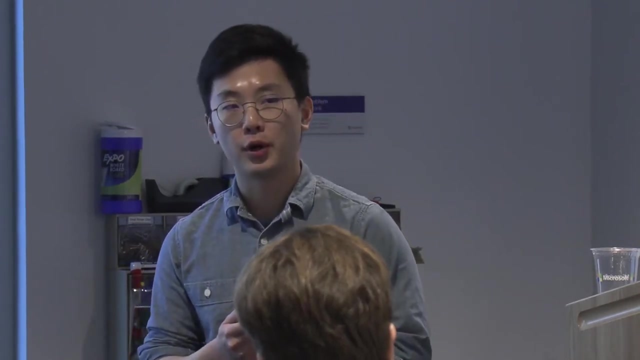 you can encrypt your data or you can do this secure multi-party computation so that the data is never leaked to each party barring the output. So notice that this doesn't solve all the problems, because you could still have some poisonous training algorithm where you can still ask a bunch of queries. 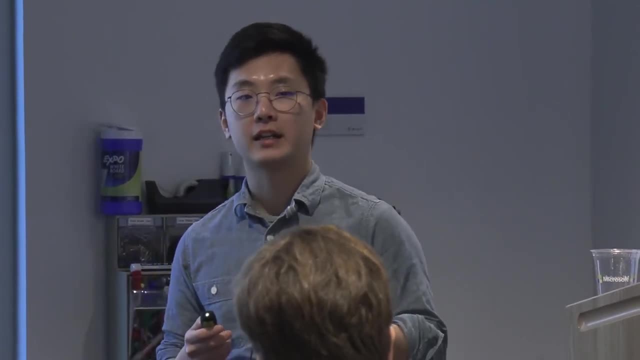 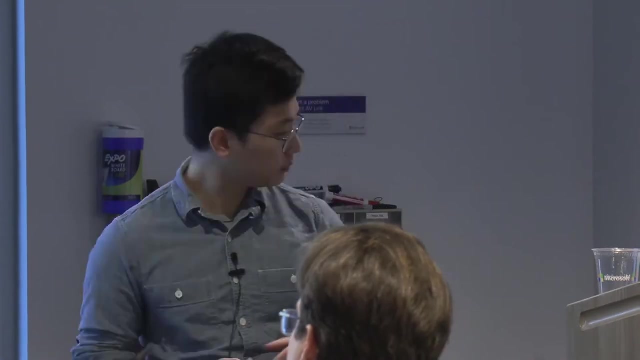 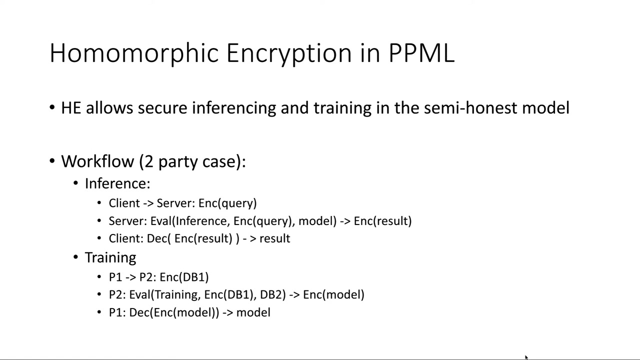 But it's a way of ensuring that, other than the leakage of the what's supposed to happen, you don't have any extra leakage. Okay, So with that, I'll talk about homomorphic encryption, specifically in a PPML. So homomorphic encryption can allow. 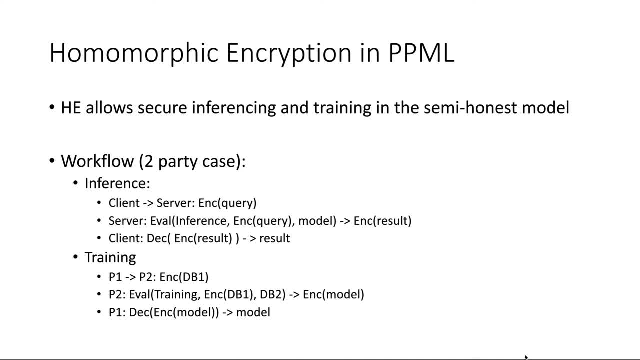 secure inferencing and secure training in a semi-honest model. Here the semi-honest just means the parties are supposed to follow the protocol, but they're trying to learn more about your private data. So a simple workflow in the two-party case goes by having 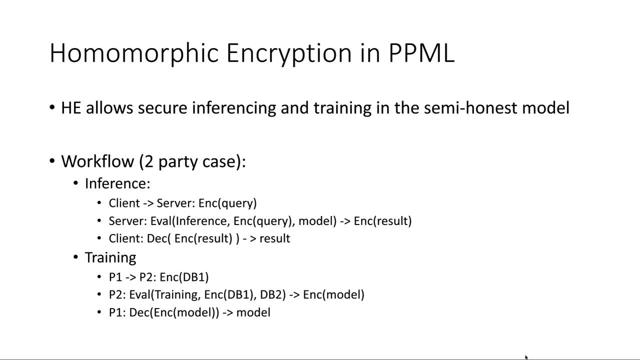 the client encrypt its query and send it to the server. Server, which is holding a model, will evaluate this machine learning inferencing function and generate an encrypted result. Finally, this encrypted result is sent back to the client, who can decrypt and get the final inferencing output. 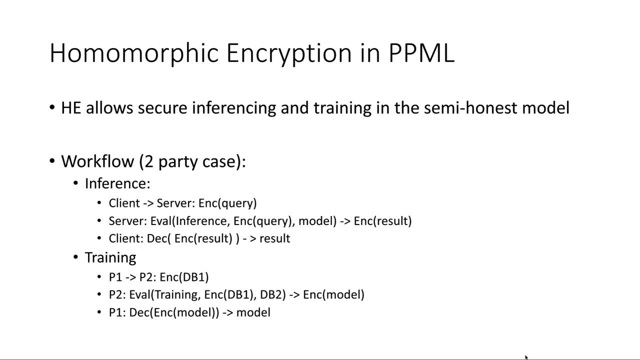 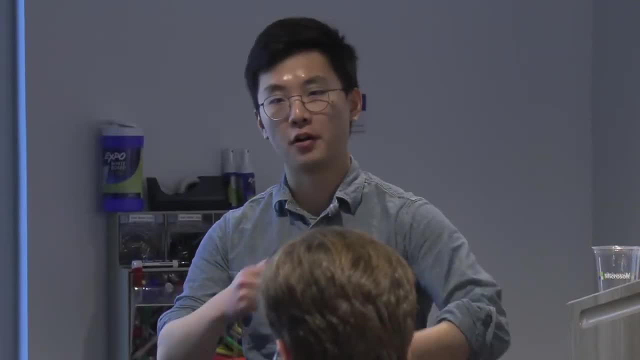 For the training. let's suppose that you have two parties each holding a part of the training dataset. It could be split either horizontally or vertically, but you can have any arbitrary party encrypt its dataset and send to the other, and the other party does all the training on the encrypted data. 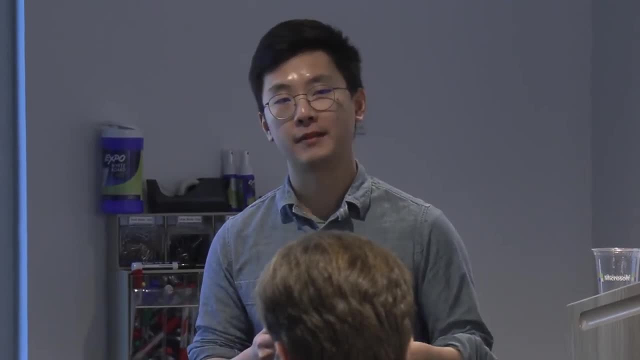 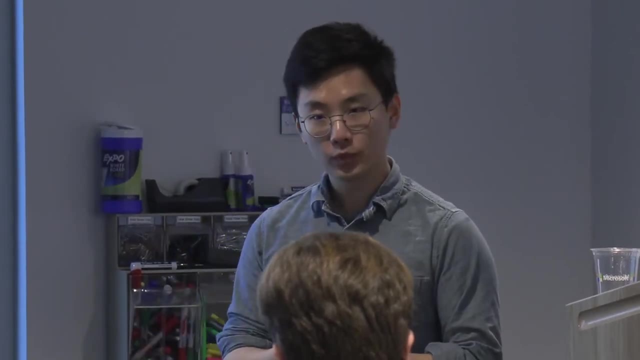 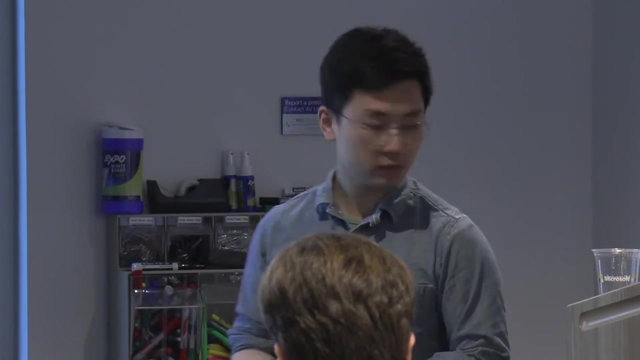 maybe just throwing in its own plaintext training data and generate a final model, and then we have some mechanism of sharing the model between the two parties. So this is roughly like how HG has been used in this PPML domain. So I'll talk a little bit about the literature. 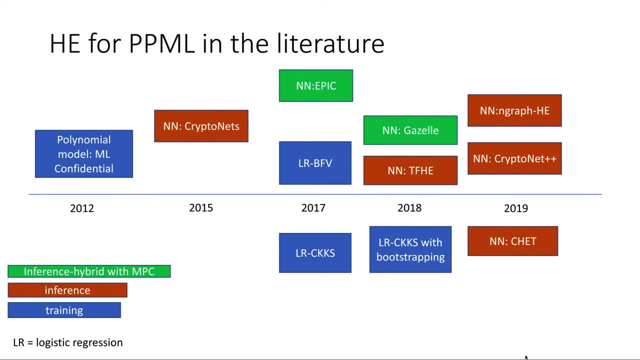 So it actually starts in 2012,, just three years after the fully homomorphic encryption invention, where there was a training algorithm for simple polynomial model- and this is done, work done inside our group- and also in 2015, we have used homomorphic encryption. 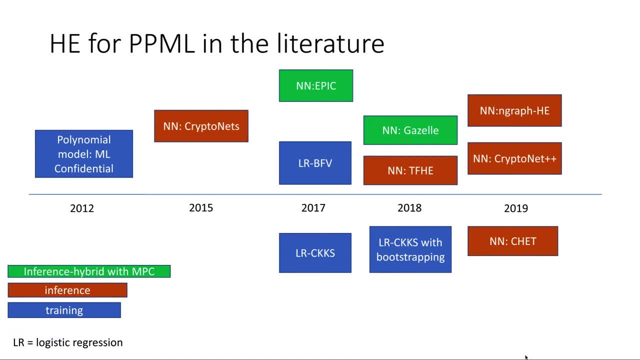 to do secure inferencing for specific neural networks. So here, the color coding is that the blue ones are for training and the red ones are inferencing and the green ones are inferencing with hybrid solutions. So in 2017, there's some work about using 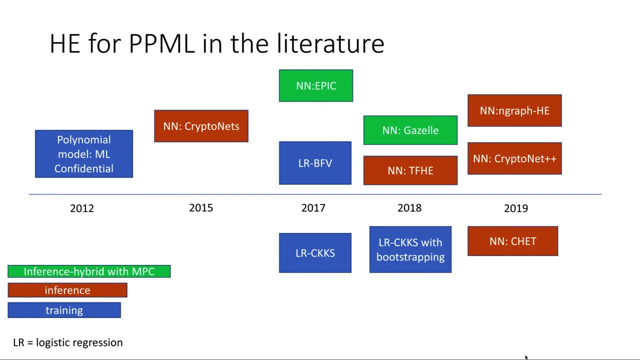 homomorphic encryption to train logistic regression models, and there's also more and more efficient ways of doing inferencing on neural networks, And the 2019 sees like even some incorporation of this: automatic compilers which takes input in neural network and output a program. 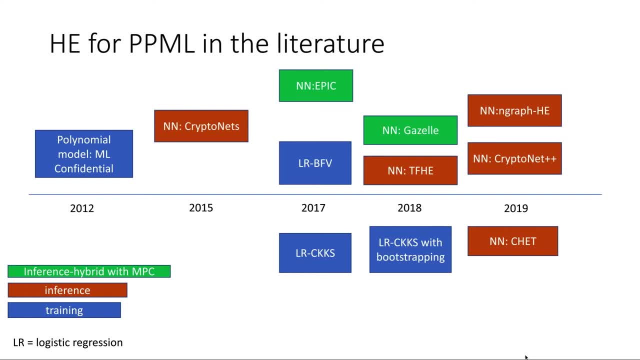 which you can just directly evaluate using, for example, seal or any other homomorphic encryption library. So and obviously I think there's a lot of room for going forward improving this kind of work. for example, if we look at the training, and there isn't a lot. 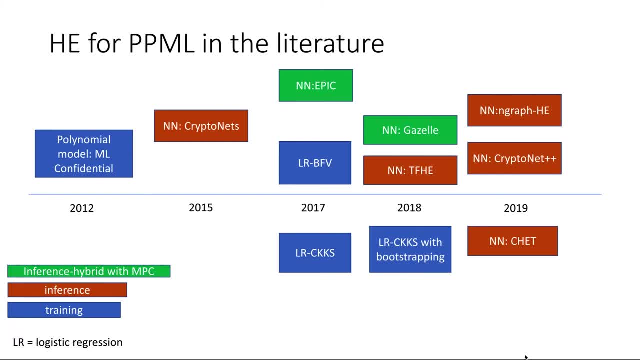 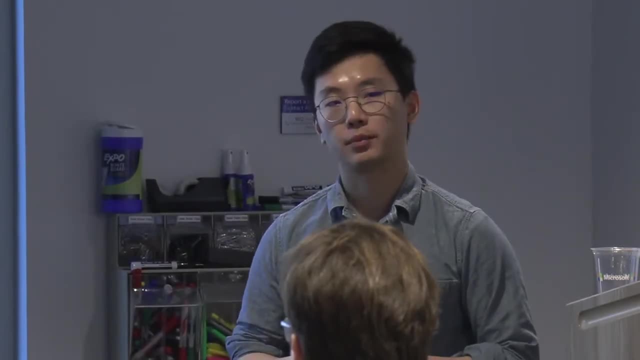 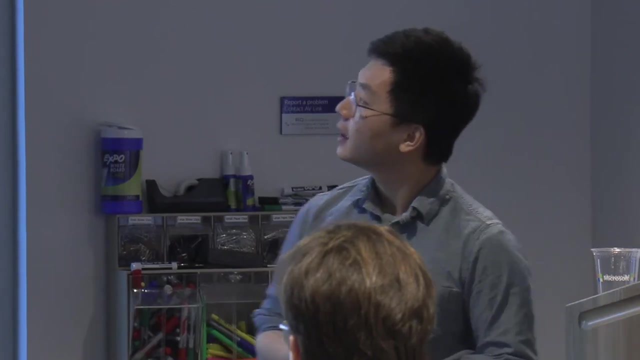 of efficient solutions going beyond the logistic regression. So for the neural networks, I think these current state of the art results still doesn't evaluate kind of very deep neural network with perhaps more than 50 layers. So those are things that I think it's interesting for the future work. 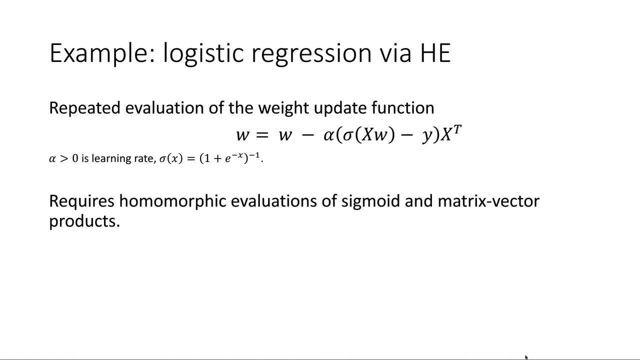 Okay, So I'm just going to take a logistic regression, for example. So if we really simplify all the machine learning training process into a single gradient descent step, then it looks somehow like this equation, where we have this weight vector W, which is encrypted, and we will evaluate this update function. 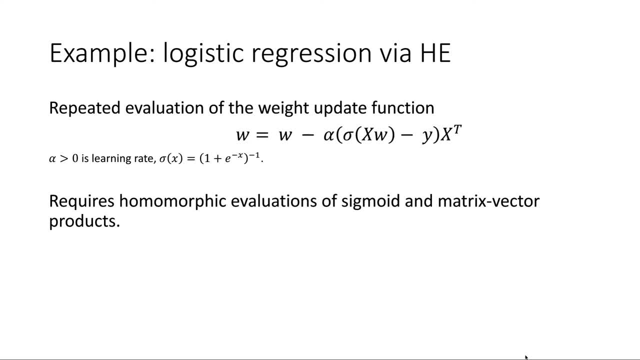 which consists of a bunch of linear operations. So here we're multiplying W as a matrix and some subtraction and some evaluation of this sigmoid function. So in particular we will need this matrix vector product and we will need a homomorphic evaluation of sigmoid. 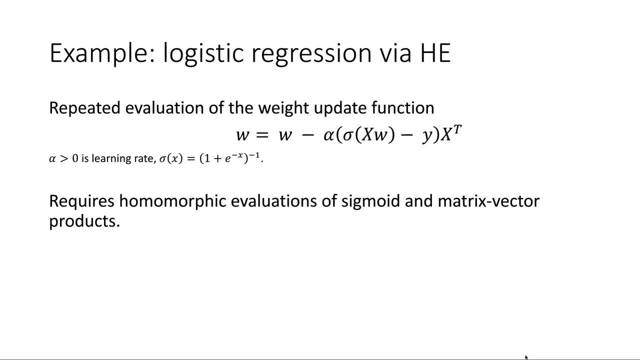 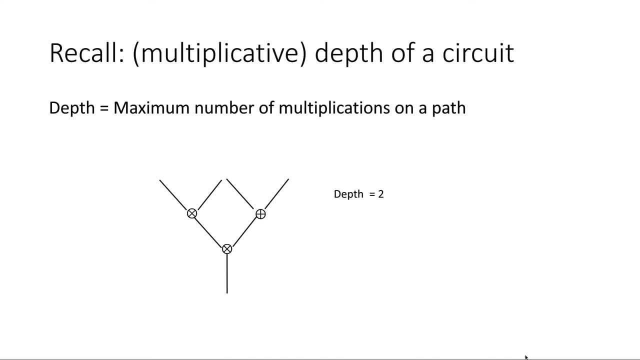 So these two doesn't seem immediately obvious how to do them efficiently. So we'll come back to these operations later in the talk. but let me go forward. So you may have heard of this notion of multiplicative depth of a circuit, So I'm just going to quickly recall the definition of that. 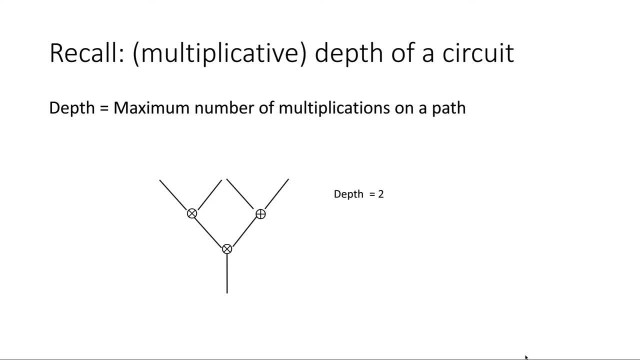 since that it is crucial to the later discussions of efficiencies in HGN and in SEAL. So the depth of a circuit is the maximum number of multiplication depth patients on the path. So in this case we have a path which has two multiplication gates. 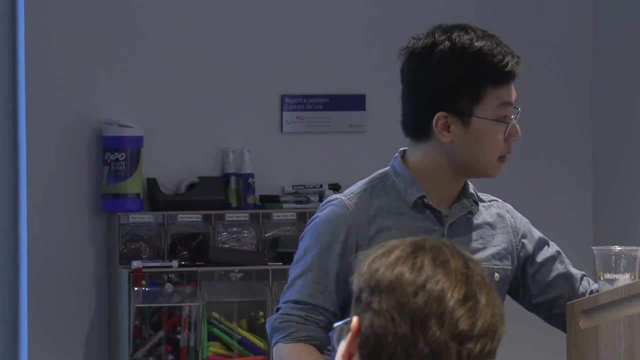 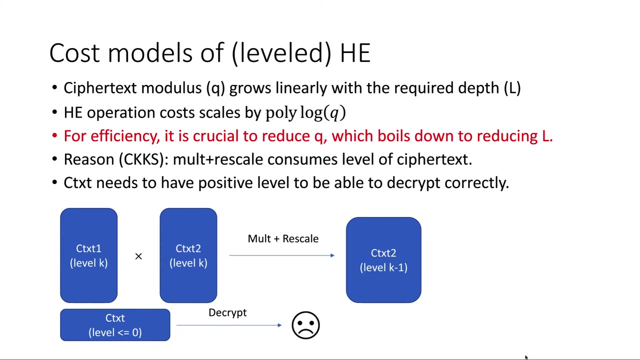 and the depth is two, And so, with that in mind, we can talk a little bit about the cost models of using this leveled version of homomorphic encryption. So I'm just going to fix on discussing the CKKS schemes from now And in the CKKS scheme. 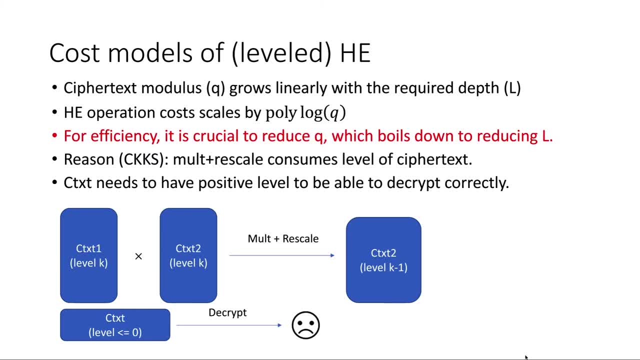 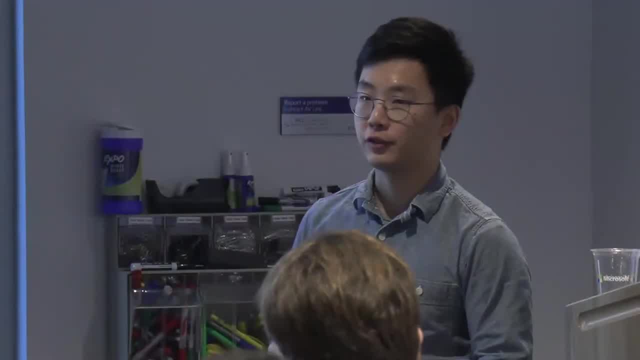 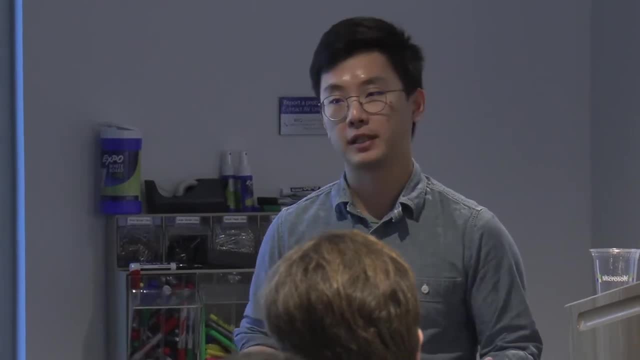 you need to set this modulus, as you have seen in the previous talks, And this modulus grows linearly with the required depth of the circuit. So if you need more depth, you need to set this modulus to be higher And that will will increase the overhead of HG, because when you do the homomorphic evaluations, 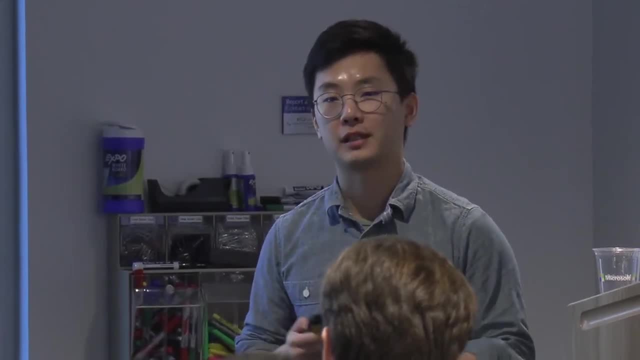 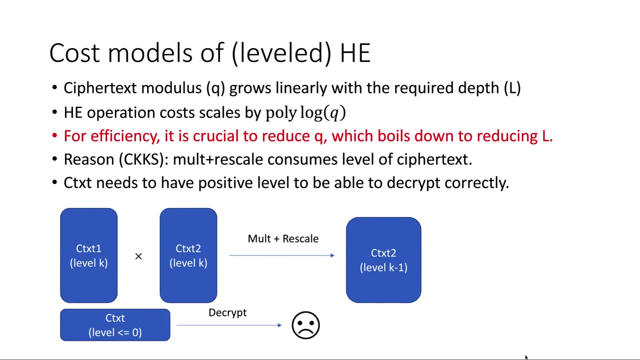 the complexity actually grows with this modulus because you're dealing with larger and larger numbers, And so, for efficiency reasons, it's very natural to reduce, or try to reduce, this modulus. And reducing this modulus comes down to reducing the depth that's required for evaluating your function. 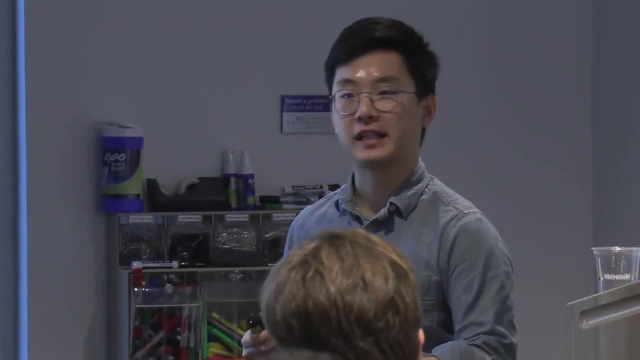 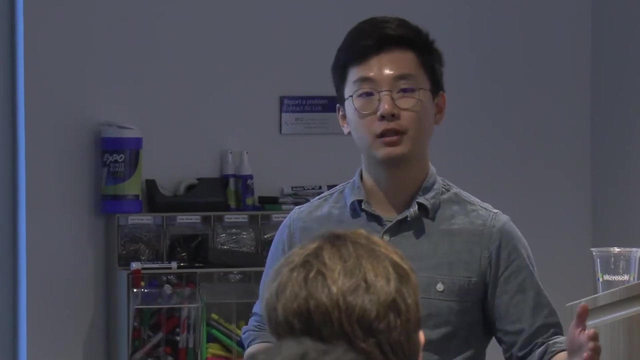 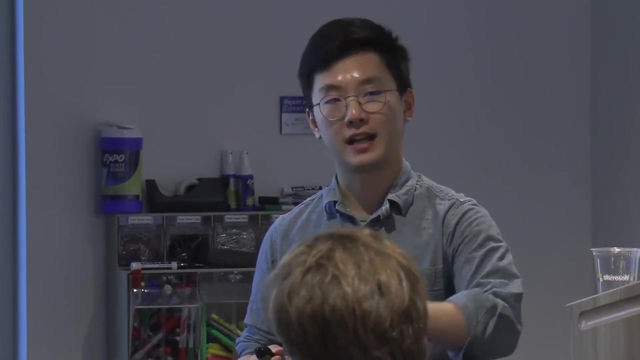 So the reason for this, at least for CKKS, is that we need to do this, rescaling operations kind of like a bookkeeping operation after every multiplication, And rescale is a simple operation but it will consume your ciphertext modulus, So it will go down by a level after each multiplication. 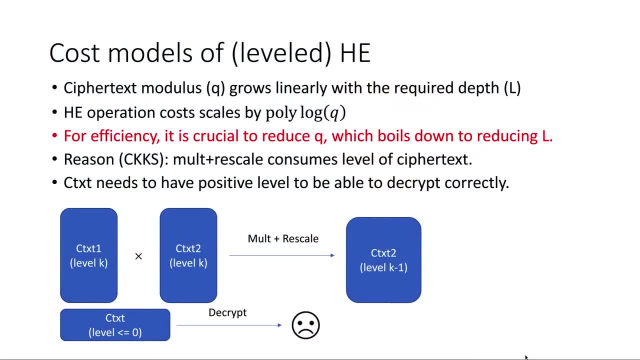 And when you achieve level less than or equal to zero, the decryption is not correct. So what we need to do is that we need to set the initial ciphertext to a high enough level so that, after all the evaluations, you will still end up with some positive level. 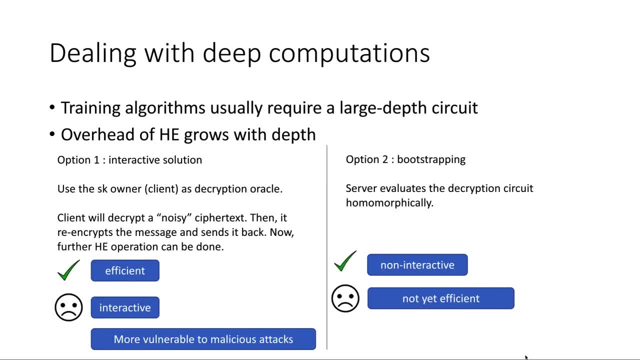 So. so then, a natural question to ask is that this, this approach, works, but it's not going to scale very well, Like, for example, if I have a very large depth circuit, if I want to train a neural network which has a 100 layers. 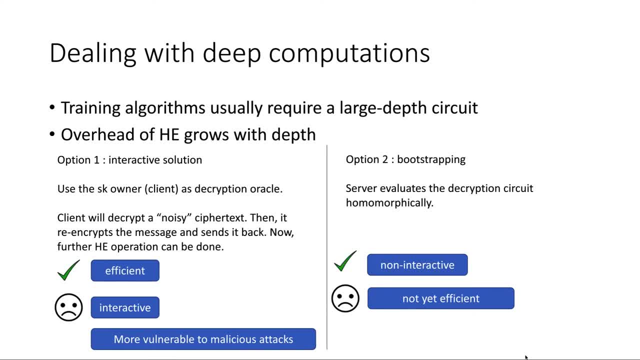 and who knows how many epochs I will be running my training algorithm. So then we can't just increase this modulus indefinitely, I think. well, theoretically you can, but it's going to be inefficient. So the question is that, once you have this deep computation, what can you do? 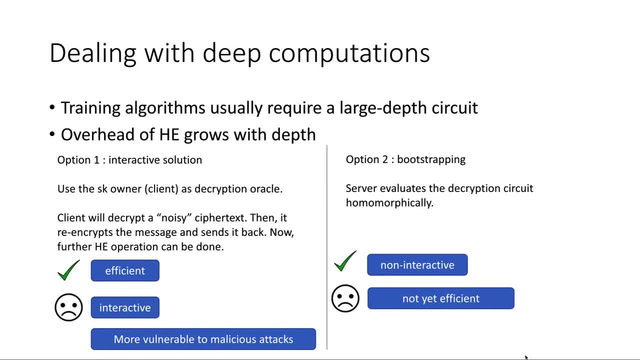 So we already covered that the overhead of homomorphic encryption grows with this depth. So we have kind of two different options. One option is to have an interactive solution where you can think of it as, once your ciphertext reaches the level where you can't do any operation anymore. 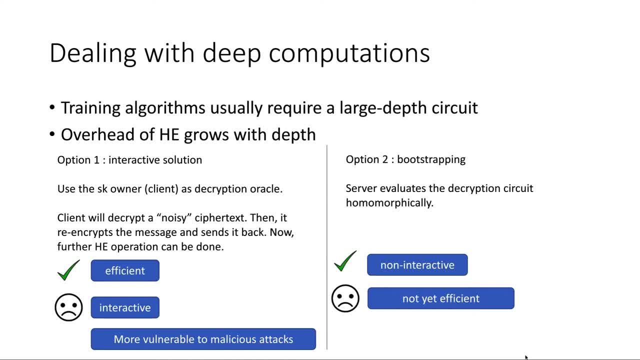 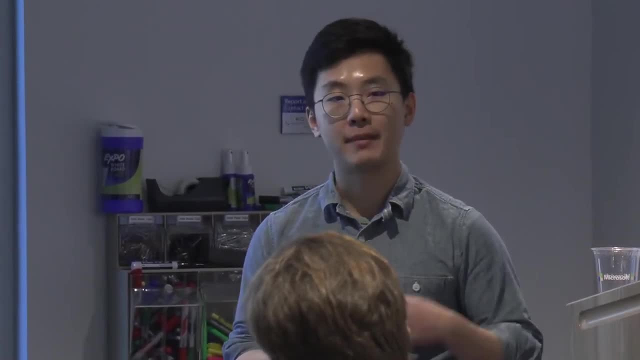 then you can send it back to the secret key owner who can decrypt it and encrypt a fresh one for you. So this often works with the additional kind of complexity of having to interact with the party who's data owner and that party needs to execute some decryption circuit. 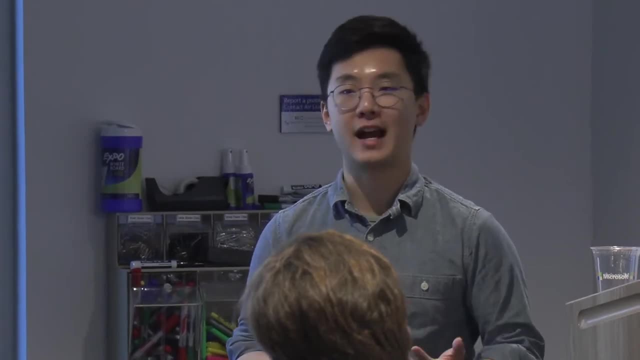 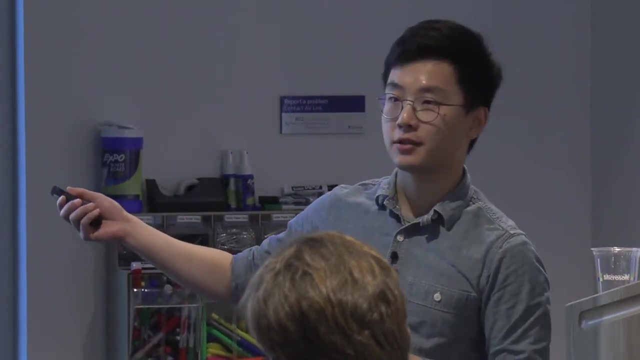 Then that opens the door to some kind of malicious attacks. So we need to be a little careful, but this is actually a valid solution. Another option is to use the so-called bootstrapping procedure. In that procedure, you will just send the encryption of. 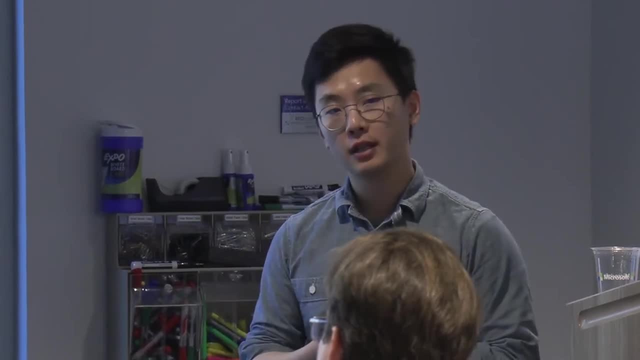 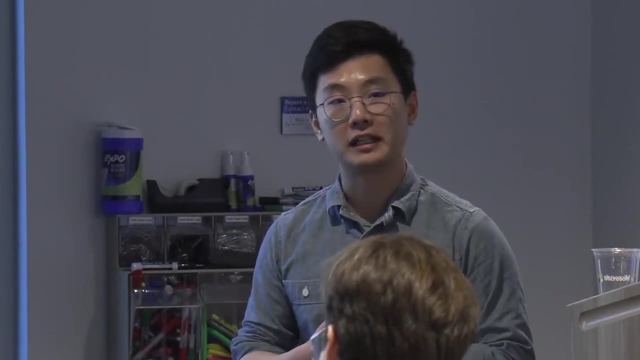 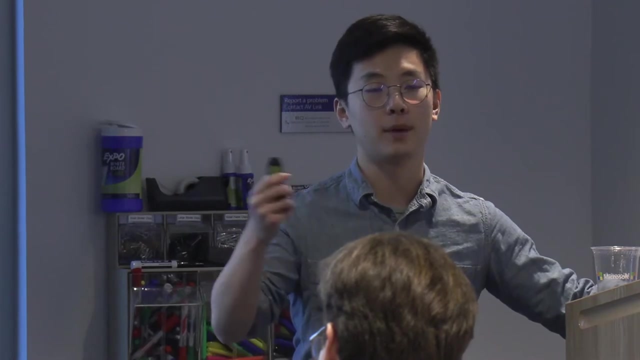 your secret key and the server will homomorphically do the decryption. So it sounds great. but after so many optimizations right now it's still a little bit inefficient. But the benefit is that now you don't have this interaction between the party who's doing. 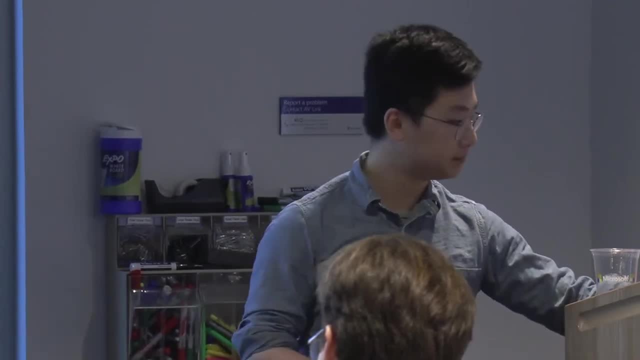 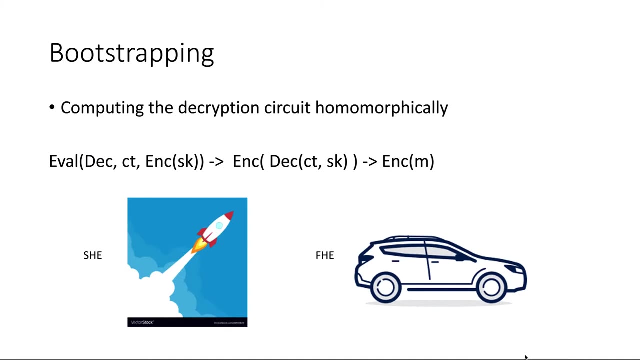 the computation and the party who's owning the data. So just one slide about bootstrapping and I'll go forward. So, as I said, bootstrapping is computing the decryption circuit homomorphically. So the workflow is that you start with a ciphertext and encryption of the secret key. 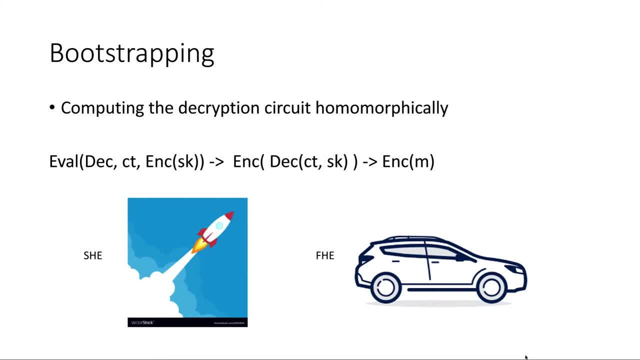 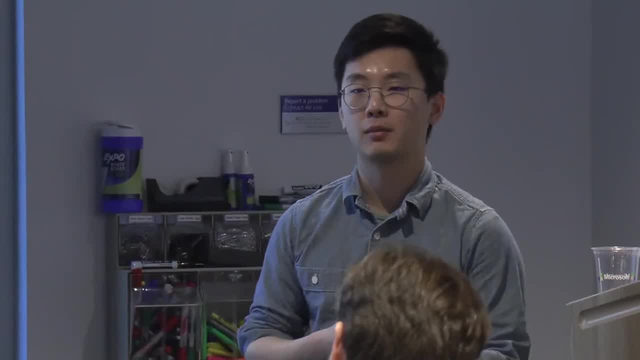 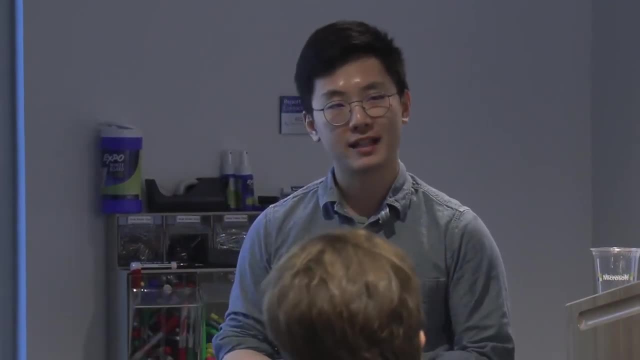 and then you perform this evaluation of the specific circuit, which is the decryption, and then you will end up with the encryption of the message, but possibly with more rooms for further computation. If you have just like one sentence comparison, I think the SHC, or leveled SHC, is like rockets. So if you want to reach further away, you need to build better rockets, but they probably also have more weights and it's more costly, which that corresponds to changing the parameters. FHE is like a car. I mean, our car is not as fancy as a rocket. 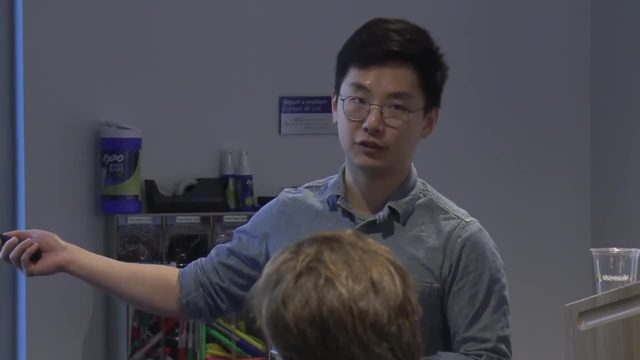 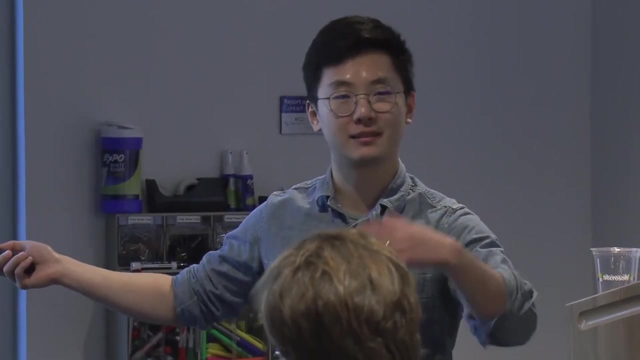 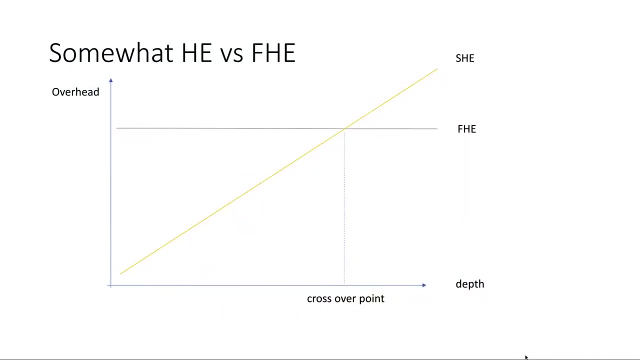 but the analogy is that if you remember to fill the gas before you run out of gas, then you can go indefinitely. like many, There's no limit of how far you can go. So this one just explains that if you have a simple computation, then using SHC is often much more efficient. 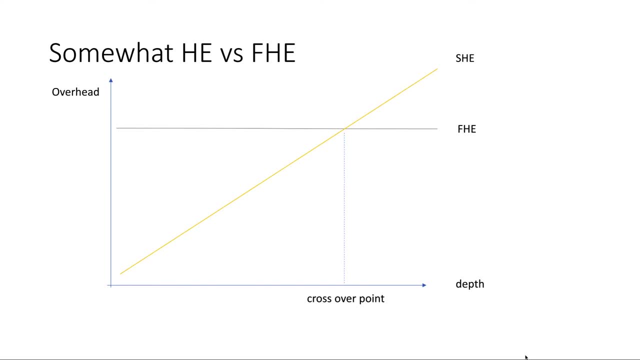 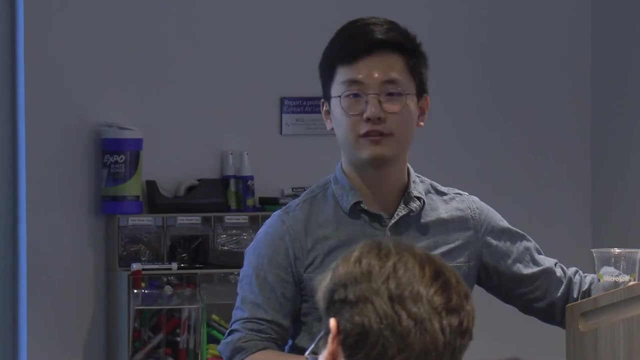 But if you are really considering a computation which can run off even like depth, thousands or hundreds of thousands, then there's a at some point, there is a crossover point where you may want to consider the FHE. But for this talk we'll just solely focus on the SHC. 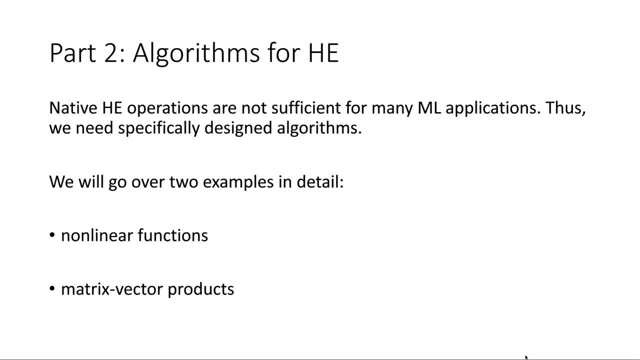 Now for the second part of the talk. I wanted to mention some algorithms that we want to build on top of the existing HE schemes. So the motivation for this is that we thought about- you have maybe seen from the previous talks that HE can be used in this SIMD fashion and it's very efficient. 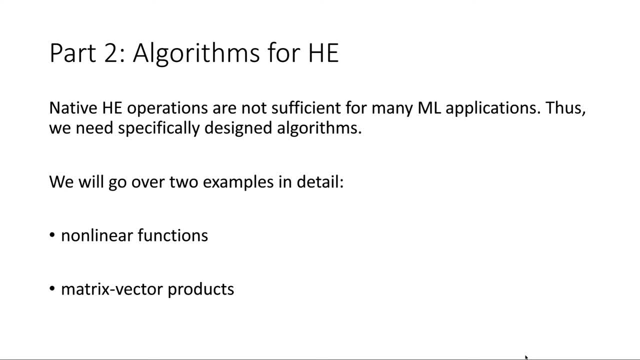 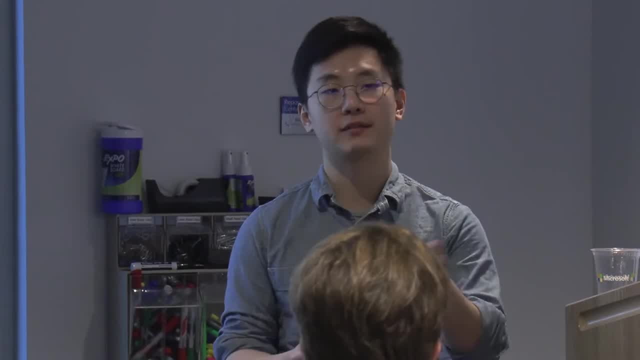 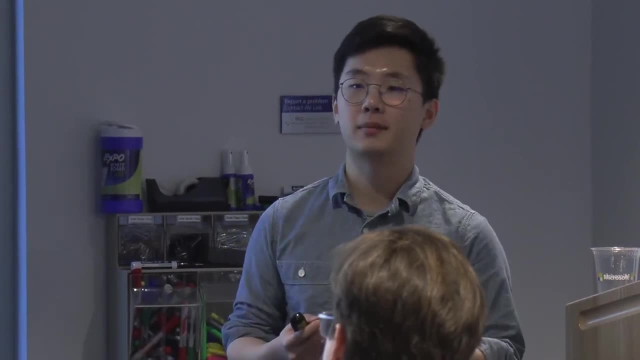 So what it supports is these operations where you can add two vectors, you can coefficient wise, multiply two vectors and you can rotate the vector. But a lot of the computation you want to do doesn't consist of these operations, So there needs to be some efficient translation of 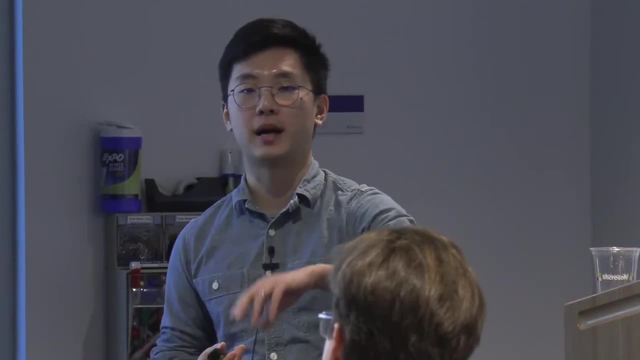 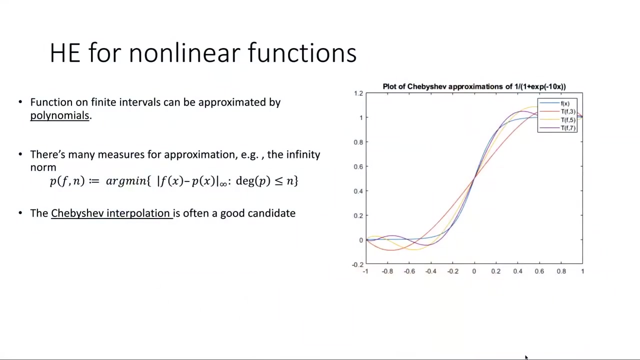 your computation into what's efficiently done by the HE schemes. So that's what I will talk about in detail. Okay, So first of all, what do we do for non-linear functions or, more narrowly, what do we do for the non-polynomial functions? 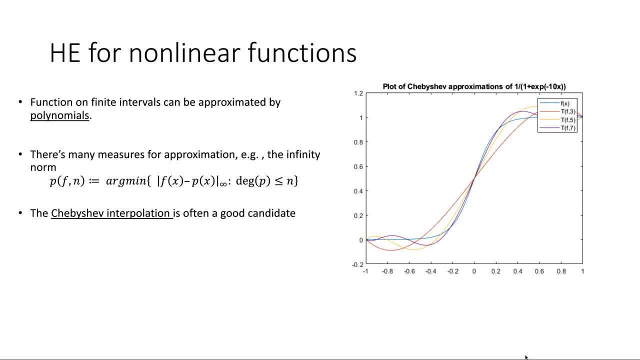 So here the example I'm taking is the sigmoid function, So it's scaled by 10 a little bit just for the picture to look nice, but it's basically the sigmoid that you use in the logistic regression. So, because this involves this exponential and divide, 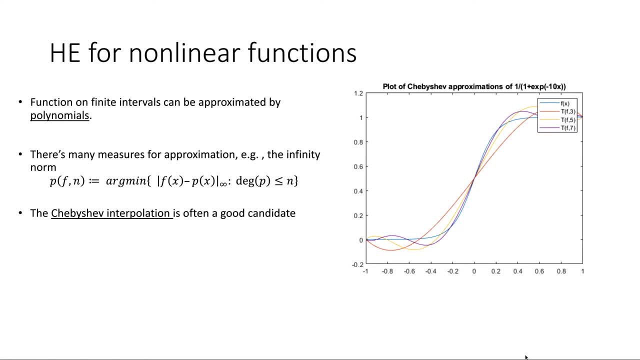 which is not amenable in HE. what we need to do is to approximate it with a polynomial. What we know is that for any given interval and any function, we can approximate this function pretty well as long as we have a polynomial of a high enough degree. 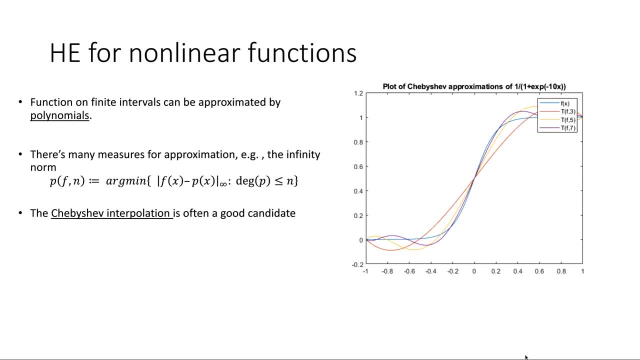 So this means two things. So first of all, we need to have this knowledge of what is the interval that will be approximating our functions. So let's say we always know that if we're evaluating this function, this input is going to be between minus one and one. 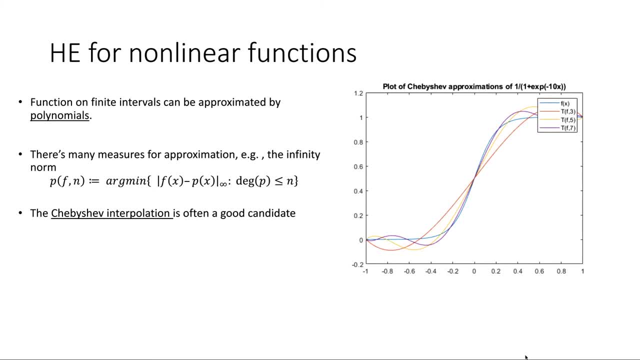 Once we know that, then we can design these approximations and computing this polynomial coefficients and then, once we set some threshold for tolerance of error, we can have a good polynomial approximation. So usually people take this measure of infinity norm to measure the goodness of approximation. 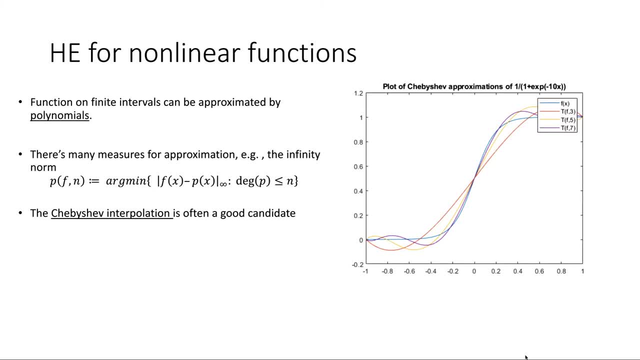 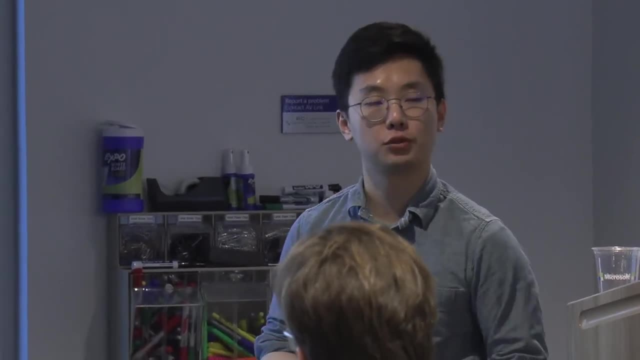 But oftentimes it's not necessary to output the best approximation, But I think at least a lot of times I use this Chebyshev interpolation to find a good polynomial approximation and it's usually sufficient. So here in this picture, 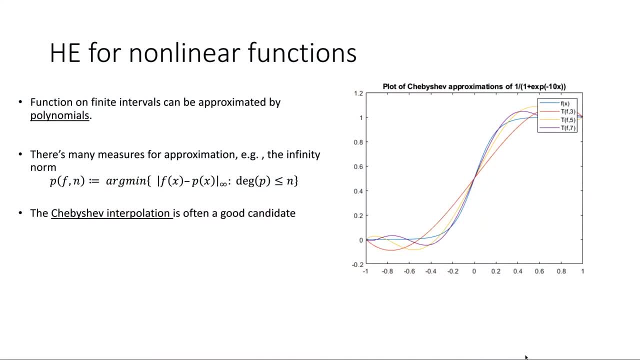 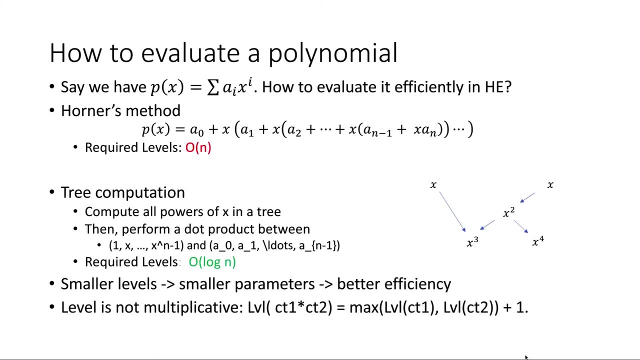 I have the function itself in blue, and the three different color curves are the Chebyshev interpolations of degree three, five and seven. Okay, That's the first step. Once that's done, we need to efficiently use He to evaluate a polynomial. 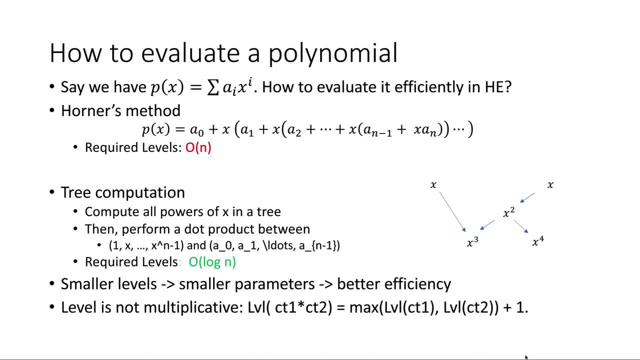 So suppose we already know these polynomial coefficients, these Ai's? There are multiple ways of evaluating the polynomial. if you think about it, So maybe like in the plain text, you can have many efficient ways, different ways of doing it. But in the He because the cost model is different. 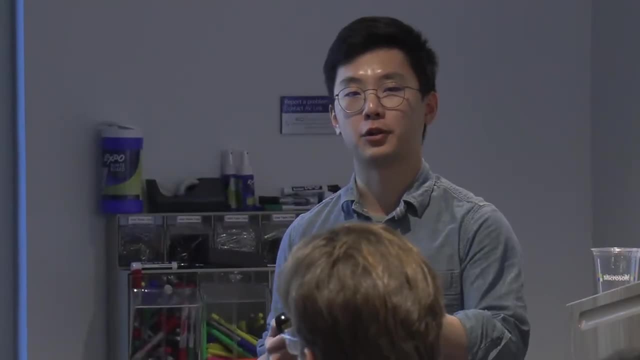 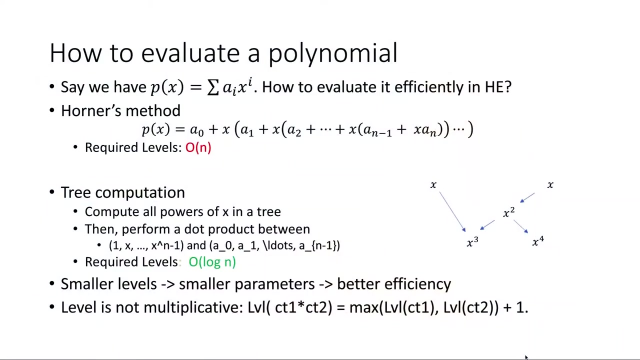 we should think of how we should evaluate this polynomial in order to make it the most efficient in He. So the first method is the classical Horner's method. So we can write this polynomial, this polynomial evaluation, as a bunch of additions and multiplication by X. 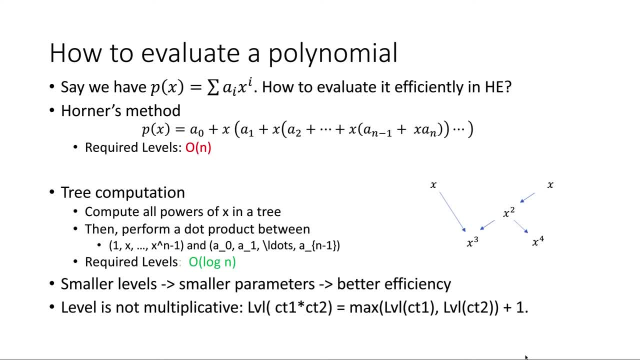 But this requires n levels, as every multiplication by X will consume one level. As we have seen, having a lot of levels is not good for the efficiency. The second idea is to use this tree-wise computation where we forget about these coefficients. Ai for now. 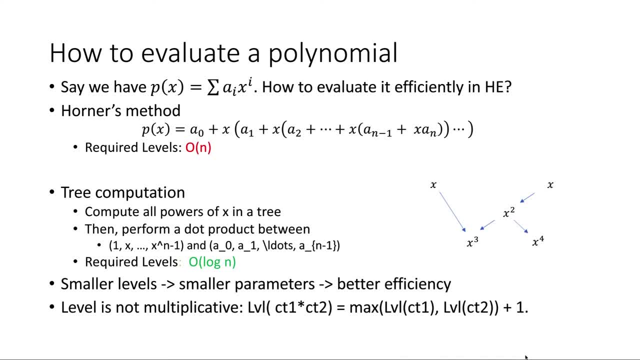 but just focus on computing all the powers of X. Remember that right now X is encrypted, So we can compute all the powers in a tree where the highest power of X can be computed using only log n levels. So this is good, because then, after we have all the powers, 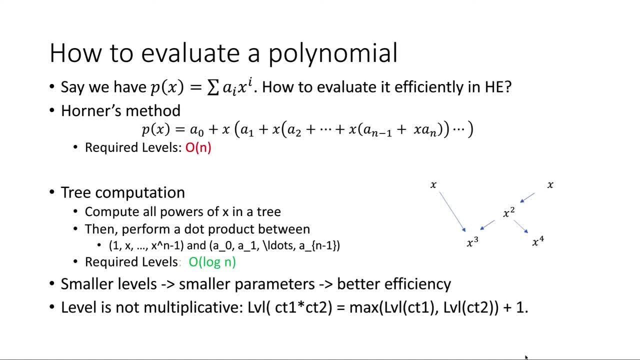 we can just do a dot product with all the coefficients, which is supposedly in plain text, and then we just need log n levels. This doesn't require much more computation, so it's good With the smaller level. sometimes they even allow us to go to. 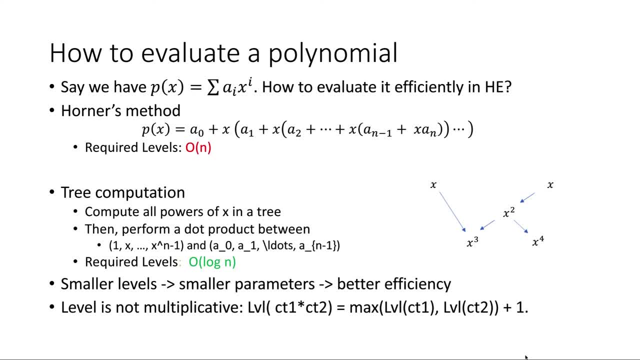 smaller HE parameters and it's much better efficiency. The reason that this works is because this level notion is not multiplicative, but rather it's like a max construction, where you have two ciphertexts and you want to multiply them. the resulting ciphertexts will have. 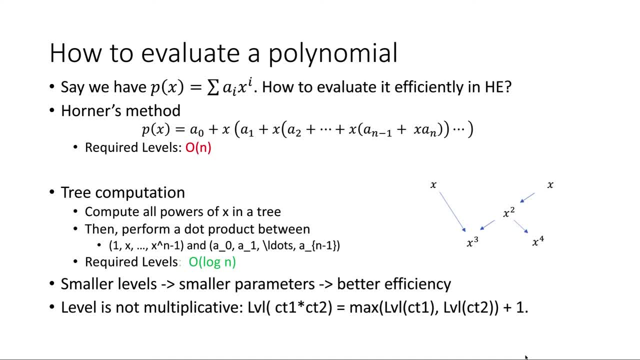 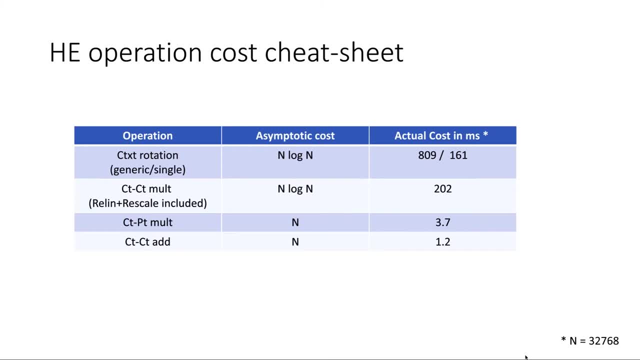 a level the maximum of the two input plus one. So before I go to the third method, let me talk a little bit about the operation costs. So in the HE I have a few of these operations which have very different cost structures. 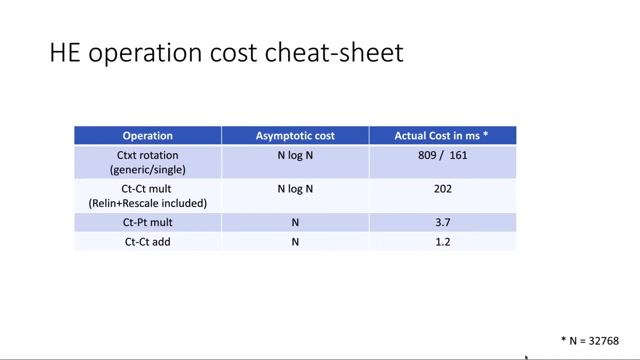 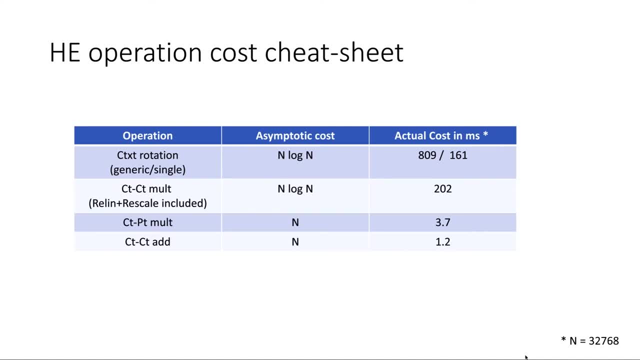 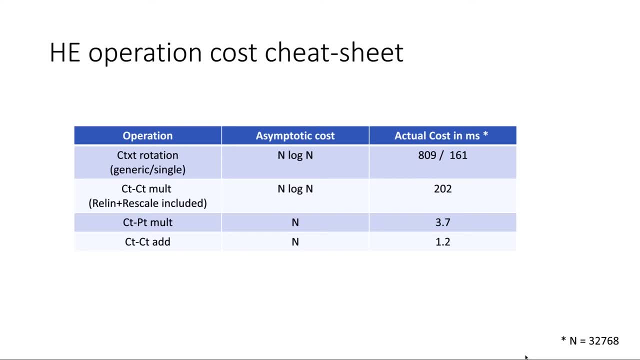 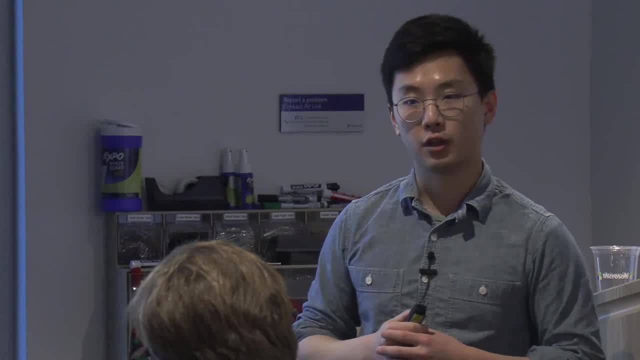 this huge vector. So if you want to compute the amortized costs, all these numbers should be divided by, for example, 16,000.. So efficiency is actually good. but we still want you to keep this in mind, because if you 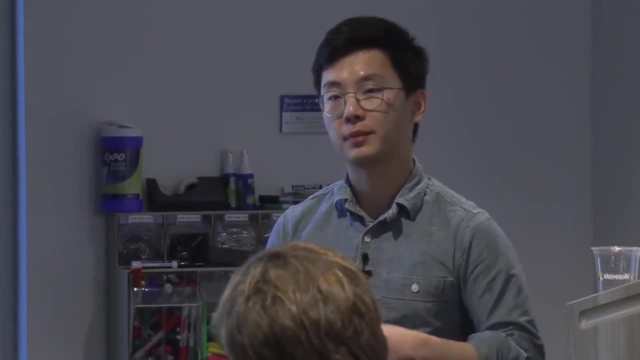 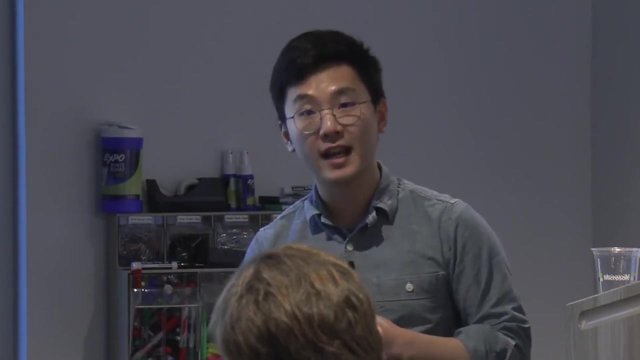 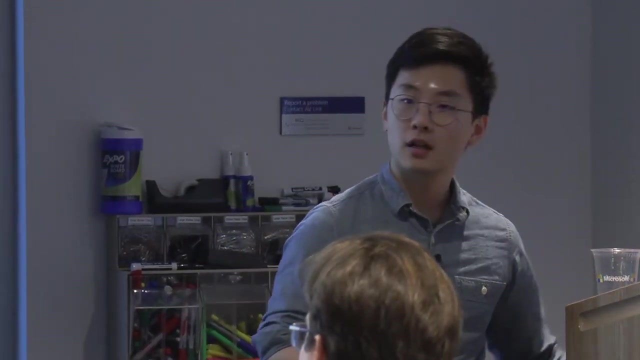 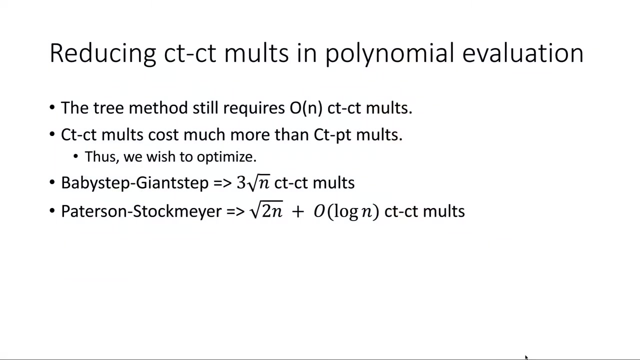 have a chance, for example, to swap or substitute the ciphertext modification with a ciphertext plaintext multiplication, then that's often a good idea. Okay, So with that in mind, I think we can talk a little bit about how to improve the polynomial evaluation method. 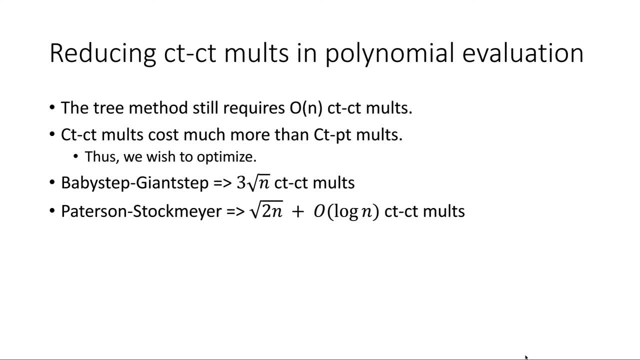 So remember that in the tree method for evaluating a polynomial, we still need to do n ciphertext multiplications for a polynomial of degree n, and this is because you need at least one multiplication to generate each power. As we see the ciphertext multiplications. 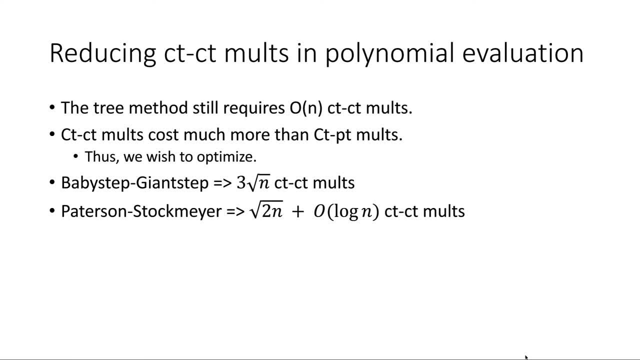 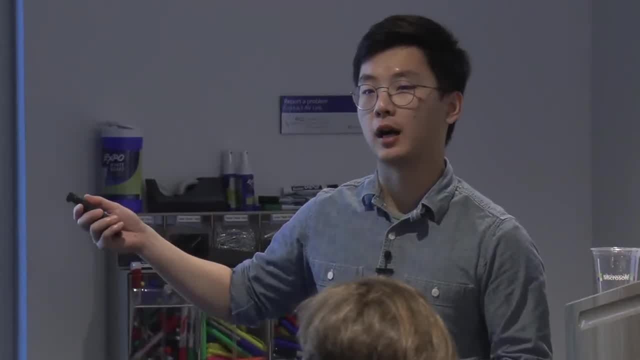 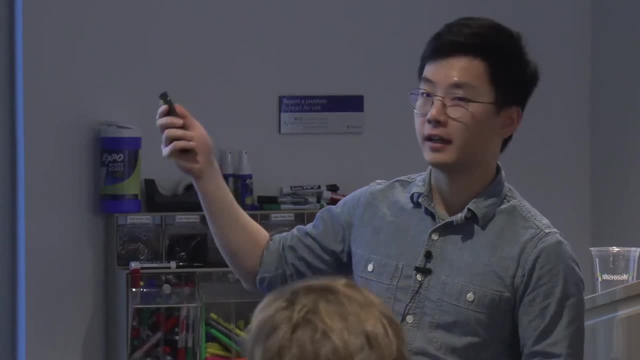 are much more costly. So it's natural to think about whether we can optimize this by using potentially more ciphertext, plaintext operations that evaluates the polynomial. So actually it's possible and in the next slide I will talk about this baby step, giant step method. 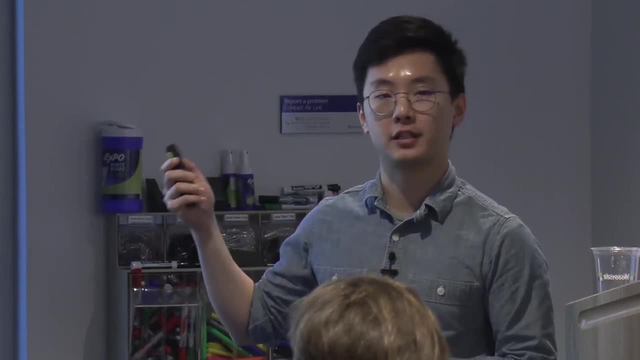 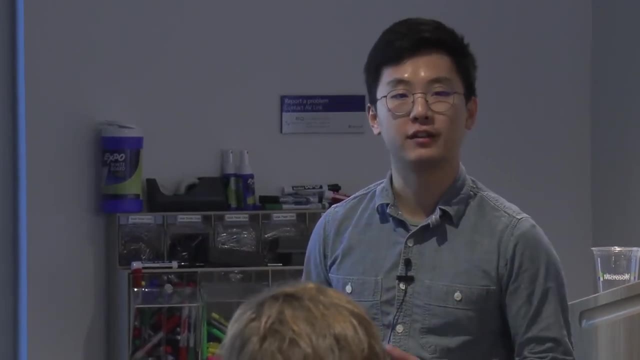 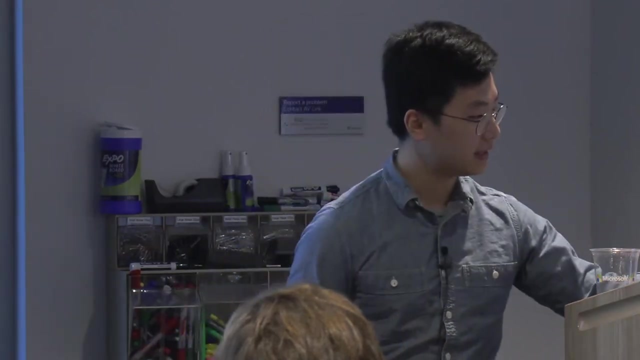 which reduces the number of ciphertext multiplications to bigger of square root of n. There's some more advanced method which gives you another save of constant factor, but it's too complicated and we can look it up, but it doesn't fit in the talk. 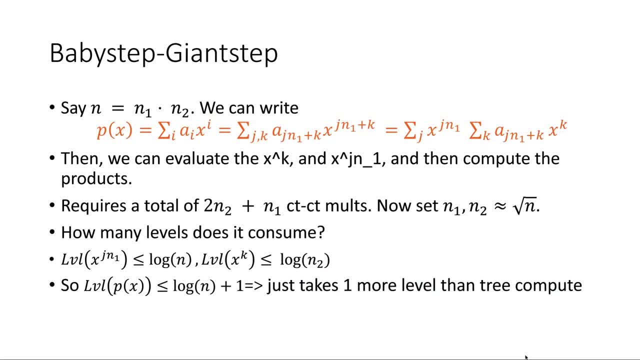 So in the baby step, giant step method, let's assume this degree is a perfect square and it can be written as n1 times n2, where the two might be similar or equal, and then this evaluation can be written as a double sum, where you: 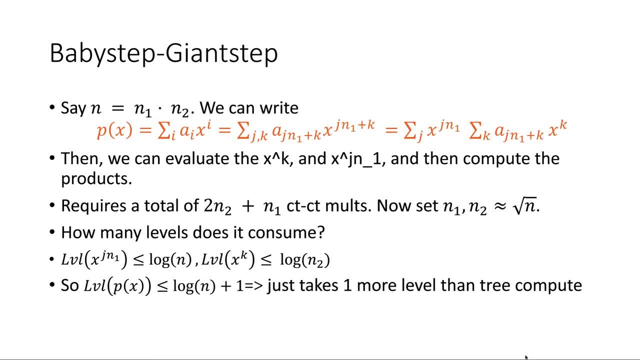 only have a sum in the inner summation with degree root n, and then this is multiplied to a big power of x. but if you count the number of multiplication it's small. So the reason is that, notice, we only need to compute the multiplication between the x to the j times n1 and all the sums. 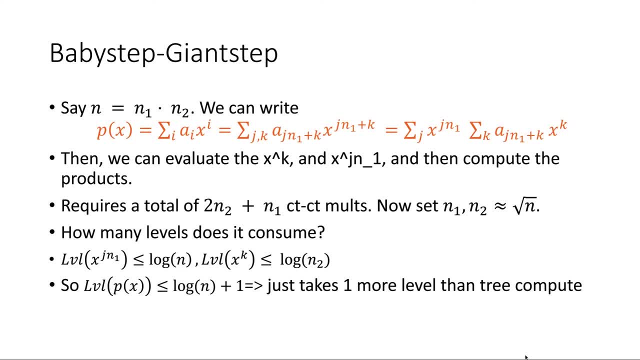 and we only need to compute all the powers of x to the k, also to a bigger of square root of n. So in this case we just need to make sure that the level it consumes is not much more than the tree method, which is log n. 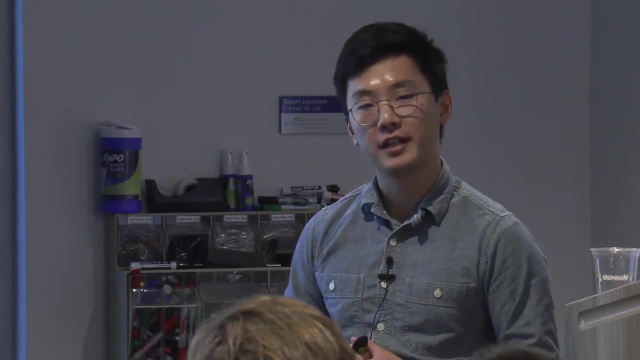 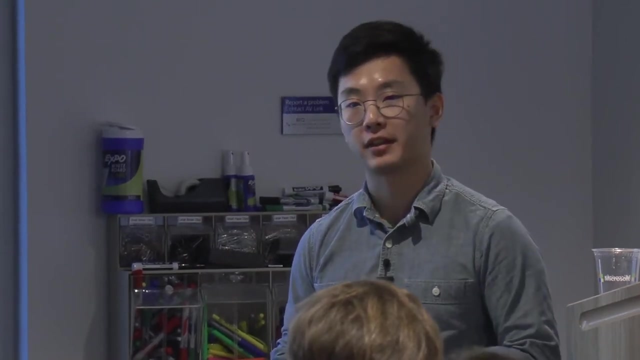 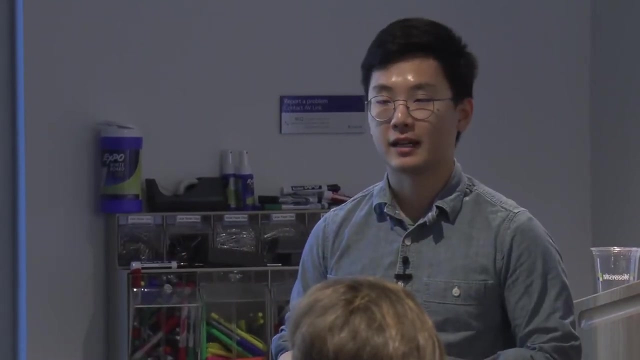 So there's a simple calculation, but we can actually show that in this case the level is just maybe one more than the tree method. So the baby step, giant step is a good method in the HG case for evaluating these polynomials, If you think about it. I don't know if it really makes. 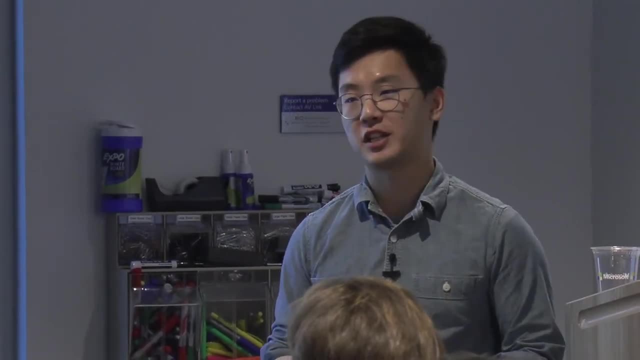 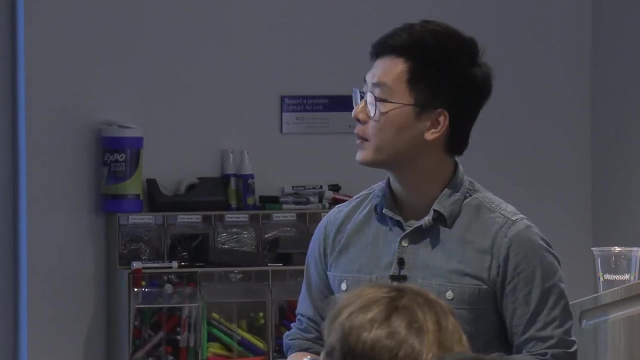 a big difference. in the plaintext case, where you don't have the HG, everything is on plaintext. Maybe you don't even want to worry about these evaluations, But in the HG, let me show you in some code examples that it actually could make a difference. 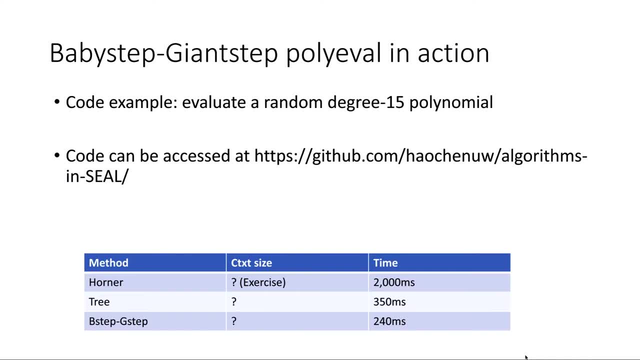 Okay, So I have some code examples and I think this repository is public, So if you go to that website you can download the code and maybe play with it and see what you get. But I'm also going to go over this code. 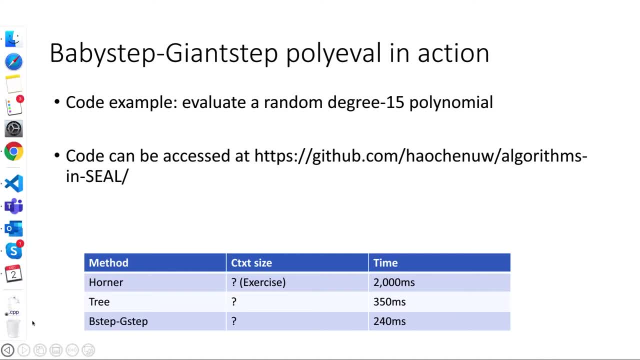 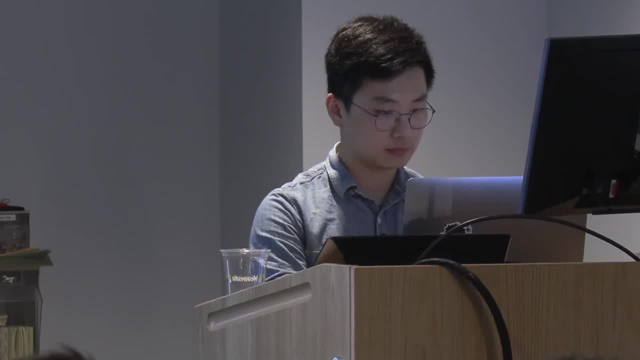 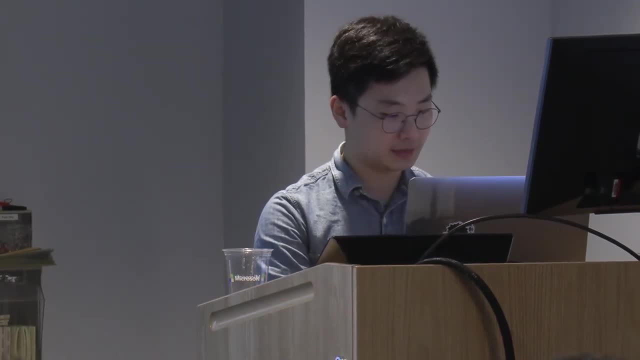 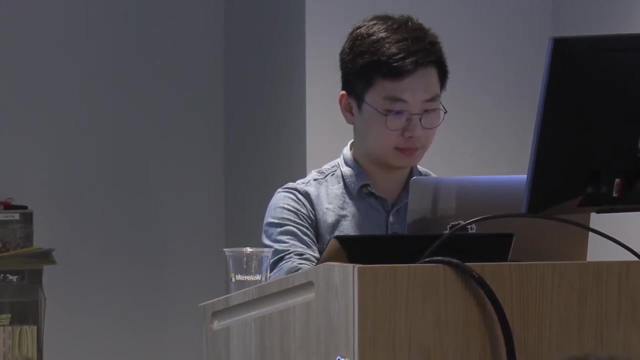 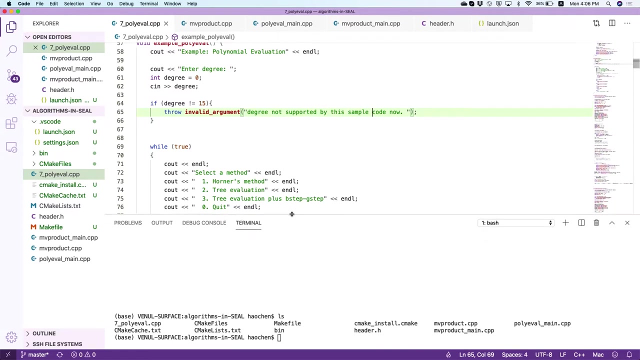 So I will show the link later. Okay, So now I already cloned the code. Let me just do a poll and make. So if you have cloned the code and I think you just need to do CMake and then make, it will generate two executables. 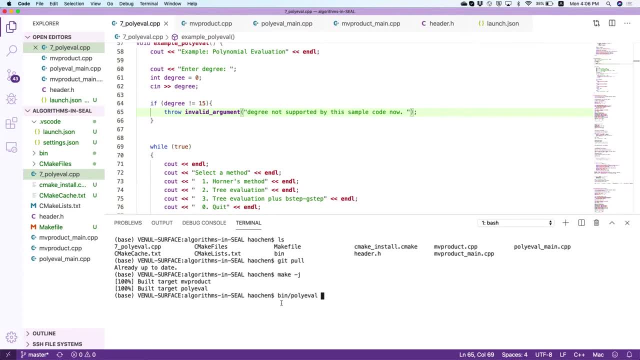 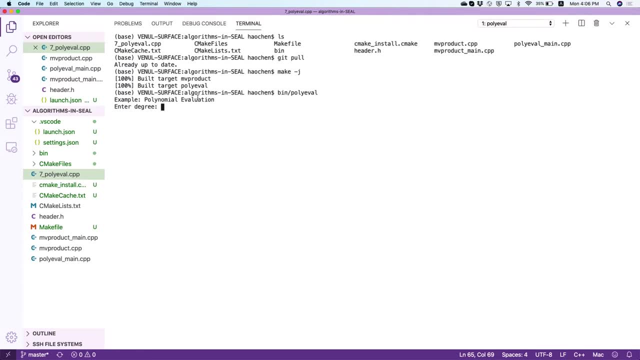 One of them is called polyeval in this bin directory. Let me just assume it's done, and then it will say that I want to do this example of polynomial evaluation and you should enter a degree. So I think if you enter anything that's other than 15,. 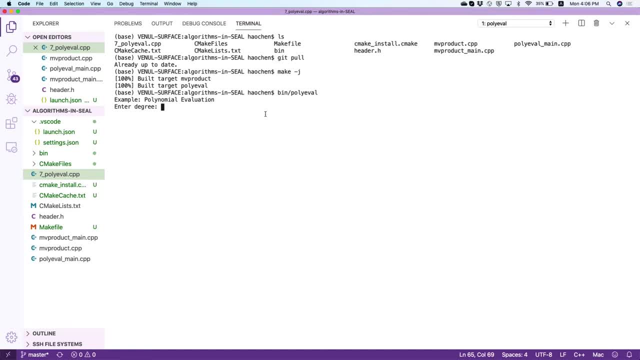 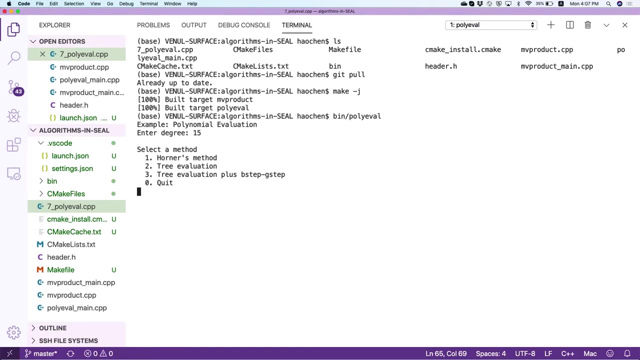 it will crash, But it's just because I only coded it for this degree. Once you enter this degree, it will let you select a method. So there are three choices: One is Horner and the second is the tree evaluation, and the third one is the tree evaluation. 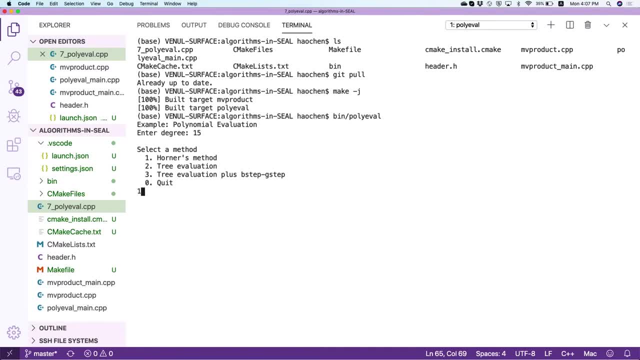 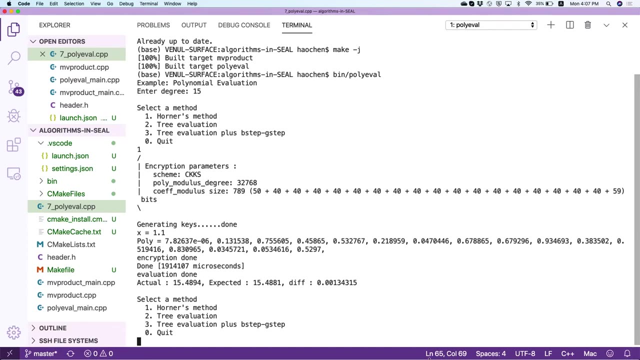 plus this baby step, giant step. We'll take a look, So I choose this Horner's method. It didn't freeze, I think it's just generating the parameters. Okay, It's done. So I will explain a little bit what this code is doing. 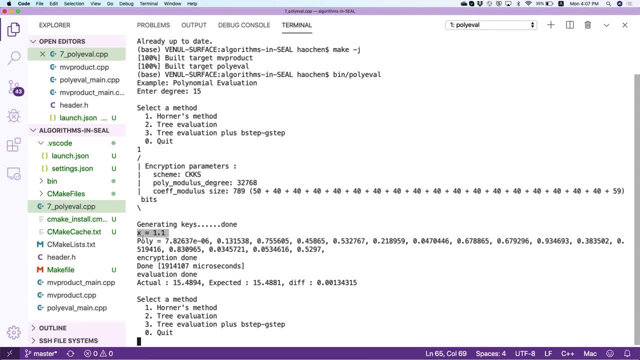 So it's selecting this input x, which is fixed to be 1.1, and it randomly generates a polynomial of degree 15 with these coefficients, and then it will use the Horner's method to encrypt x and evaluate this polynomial to generate. 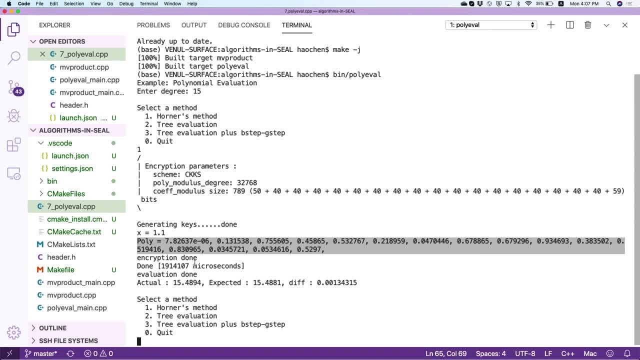 the encrypted version of the p of x, So it requires about two seconds, if I'm correct, and here I print it out, because this is using the CKKS scheme. We understand that there could be some error in the evaluation, and here I printed out the difference, which is about 0.001.. 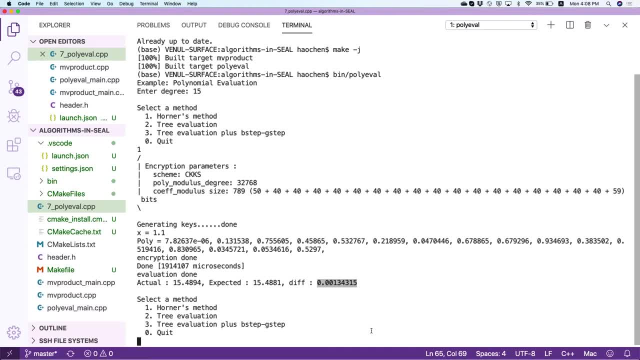 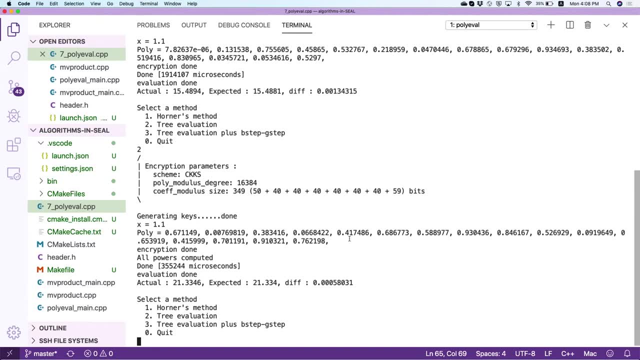 So the accuracy is okay. and now let's go to the second method, which is the tree evaluation. So it just finished and this is much faster- about six times faster than the previous. So notice that this is true because, due to this tree method, 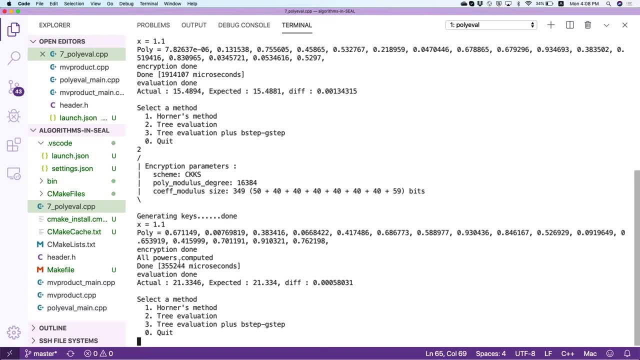 requires much less level. we can select parameters which are smaller, and smaller parameters means that usually you have much better performance. Now let's do the tree evaluation plus the baby step, giant step. So it's even a little bit faster than the previous technique. 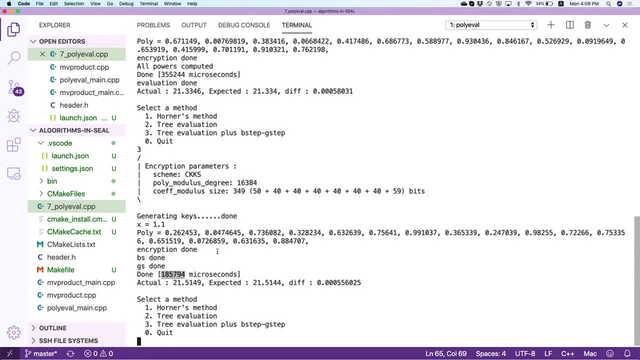 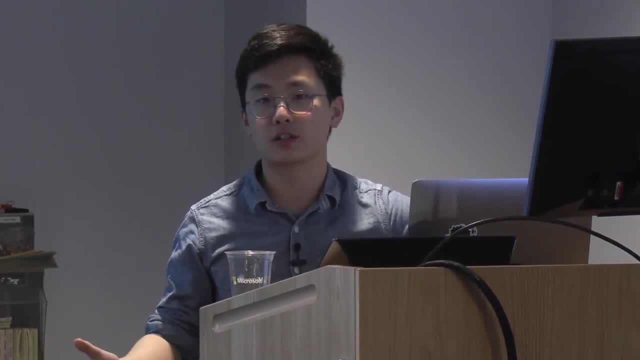 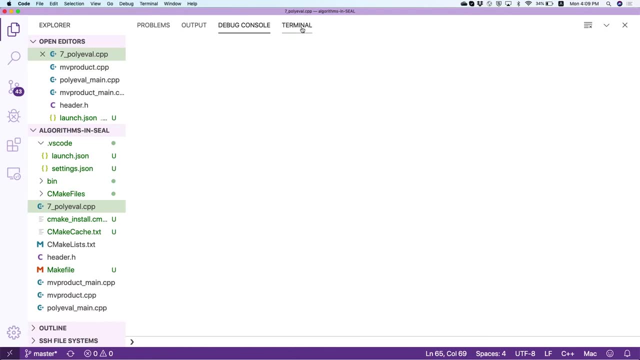 So remember that the degree is 15.. So if you work out the math, you roughly get like half of the required ciphertext multiplications, which is dominating the cost. So yeah, feel free to play with the code. but right now I will go into the code to show you some. 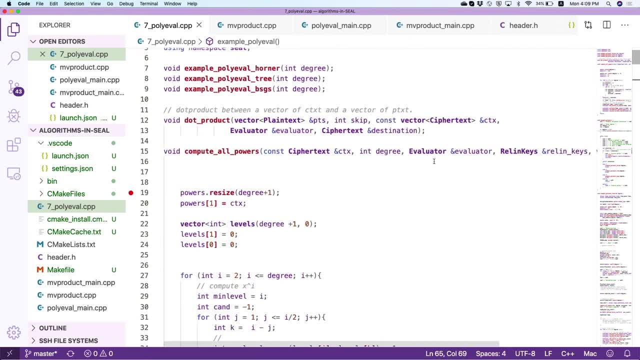 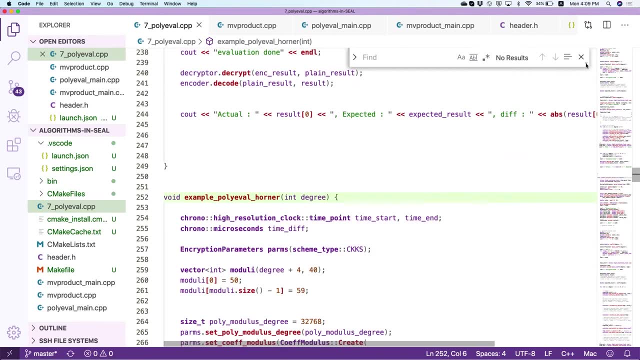 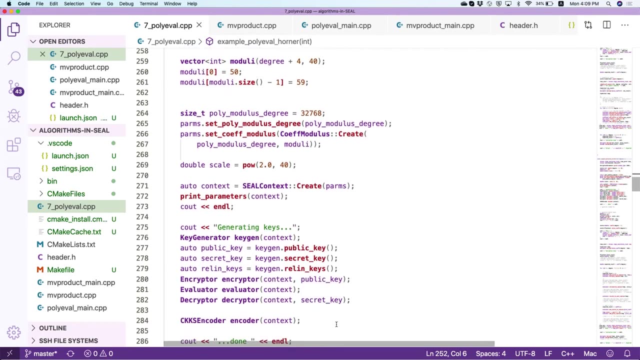 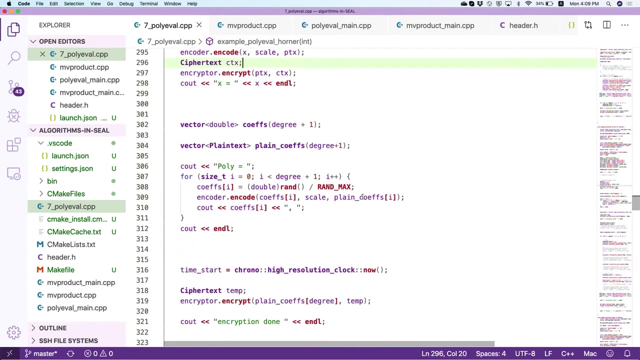 of the implementation details of how you do these things. Okay, So the first one is the Horner's method. So in this case I set the parameters and generate some keys and sample the polynomials, encrypt this input here. This is common to all the three methods. 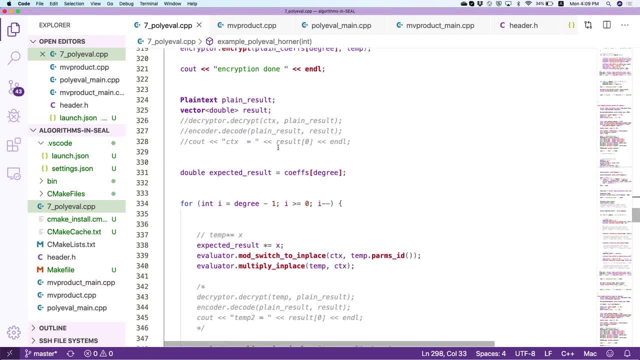 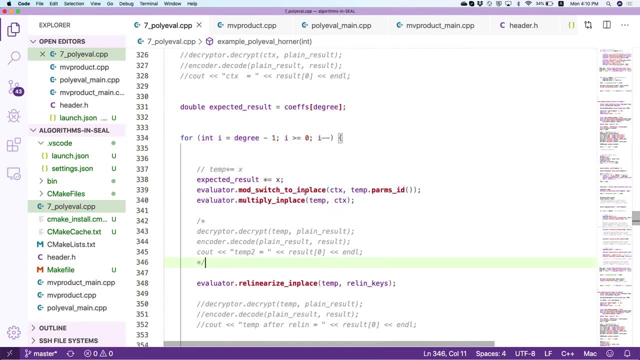 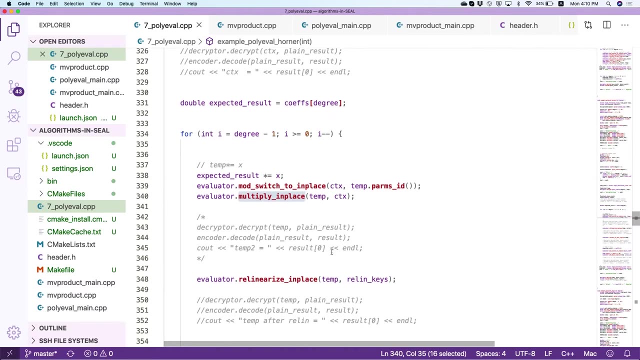 But then what I did was so remember that the Horner's method is a for loop. So in each iteration in the loop I do this multiply of the current evaluation with the encryption of x. And then there are some bookkeeping operations. 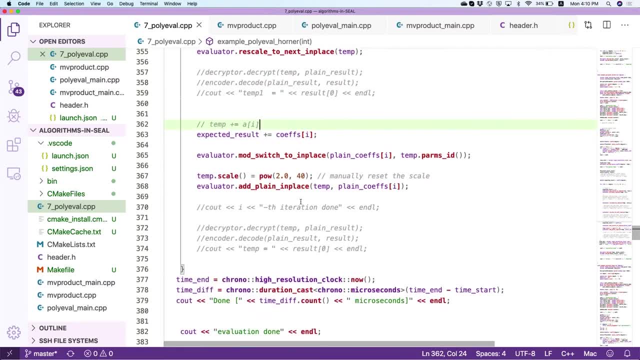 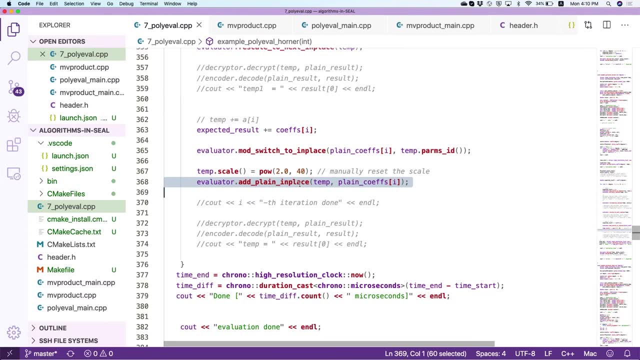 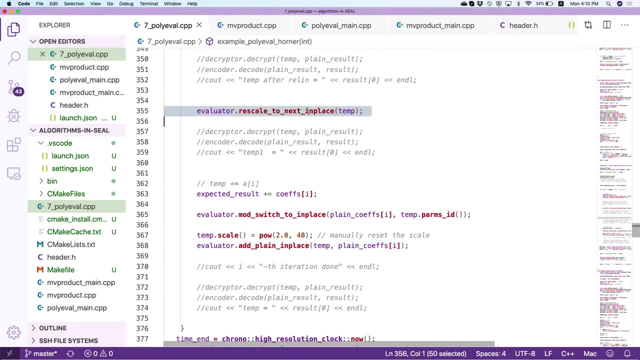 other bookkeeping operations. And then I have this addition which adds the plaintext coefficients to the temporary sum. So the reason that this is so costly is because every time I do this- iterations in the loop- I need to do the rescaling operation, and that requires one level. 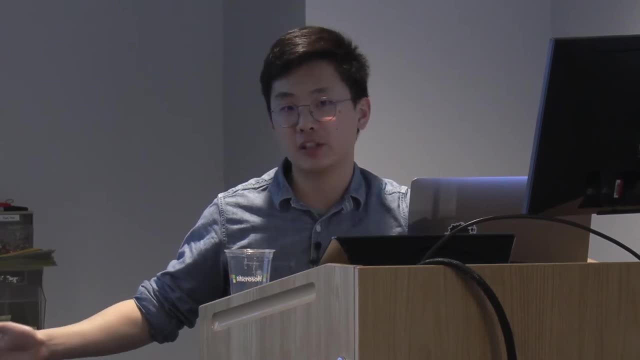 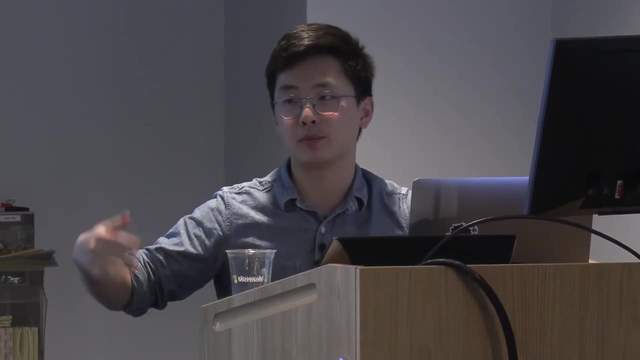 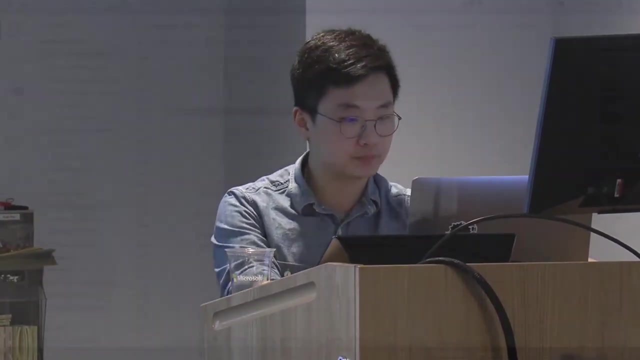 And this is the reason- Yeah reason- that I need to have at least 15 levels for the initial encryption. Although the levels kind of peels down when I'm doing this evaluation, you still start off with a quite large ciphertext and that contributes to the inefficiency. 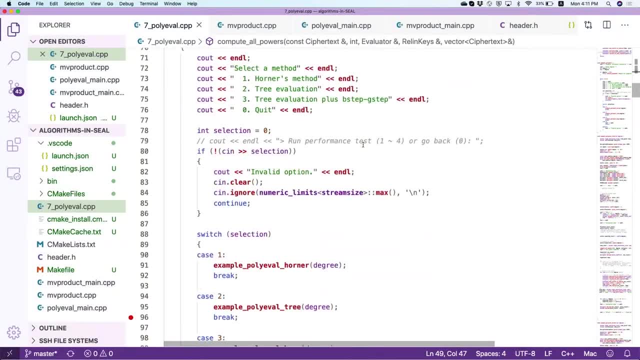 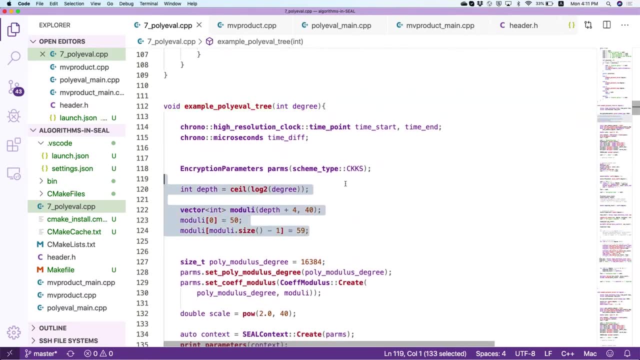 Now let's go to the second method. So the second method is kind of much better, and we can already see it here. So here we don't really have to select that many primes in a coefficient modulus where basically the level required is only logarithmic in a degree. 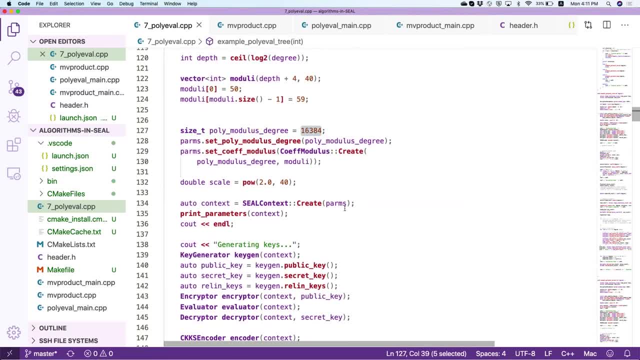 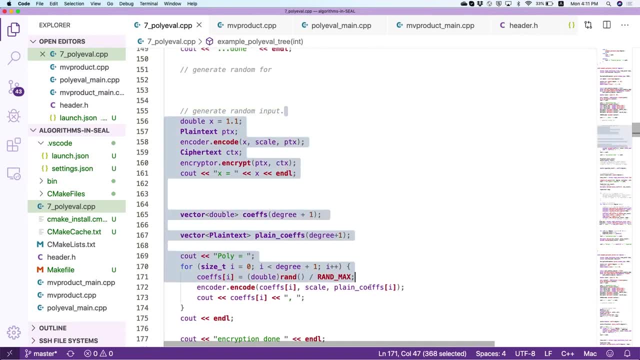 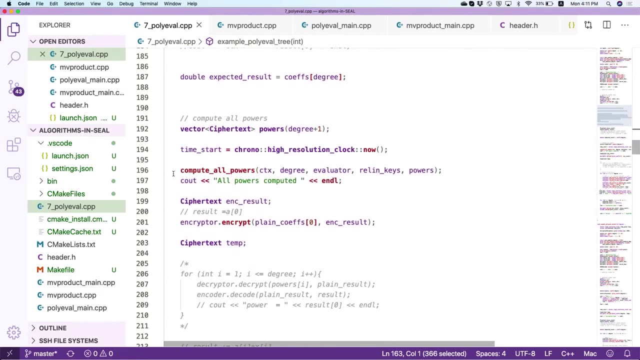 For this reason we can also select a smaller ring dimension, which is called polymodulus degree here. The rest is almost up to here. it's almost the same. We're just randomly selecting a polynomial. But the interesting happens where we compute all the powers first. 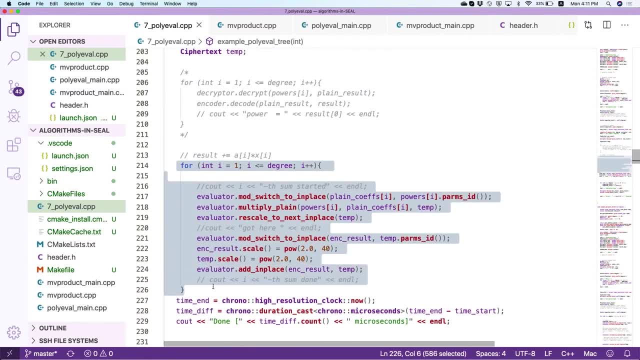 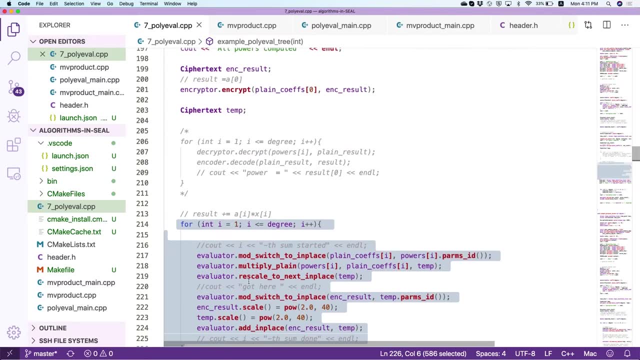 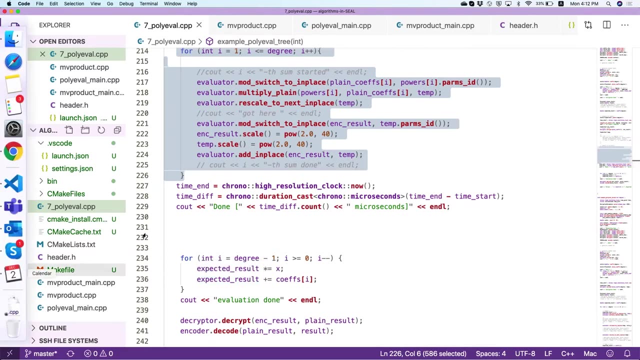 and then we do a summation which is kind of like a dot product, which is also present in Kim's talk. So the reason that this is much faster is because of the smaller parameter. So I think this is interesting For the interest of time. 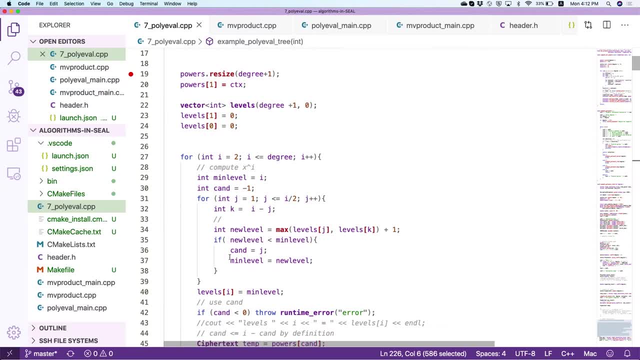 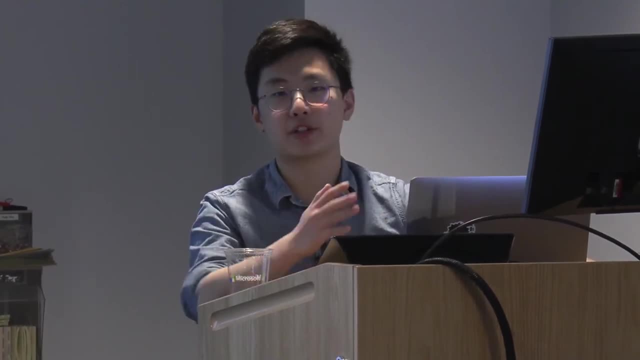 maybe I'll just leave it to you to check out the third method, which is the baby step, giant step. It actually kind of requires some effort to implement. It's not completely trivial, but I think it will be interesting to take a look and see what's going on there. 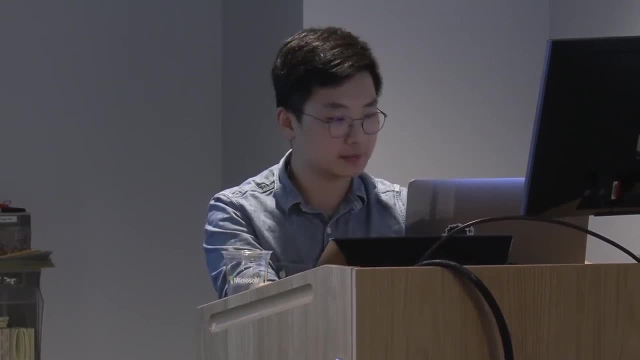 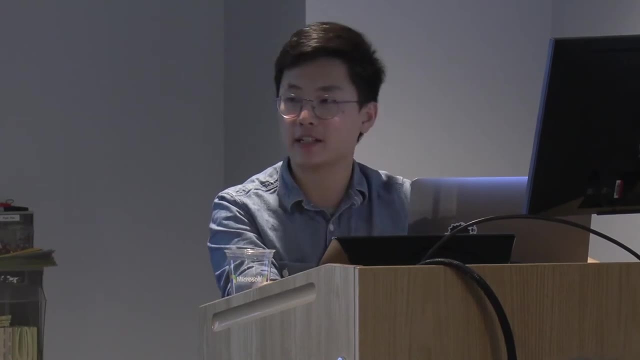 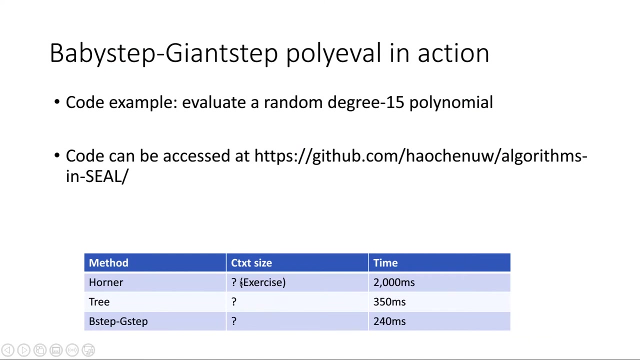 and how would you go about implementing it? Okay, So that's that, Thank you. Thank you, That's that. Another exercise I have for you is that the ciphertext sizes for these three different methods are also different. So you have learned. 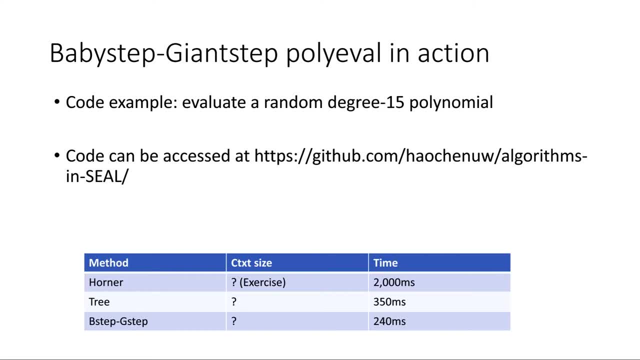 maybe from Kim, how to serialize and save a ciphertext to a file, and maybe you can just check out the size of these files for these three different methods, I think this one will be the biggest and these two will be similar. Basically, the size is proportional to how many levels is. 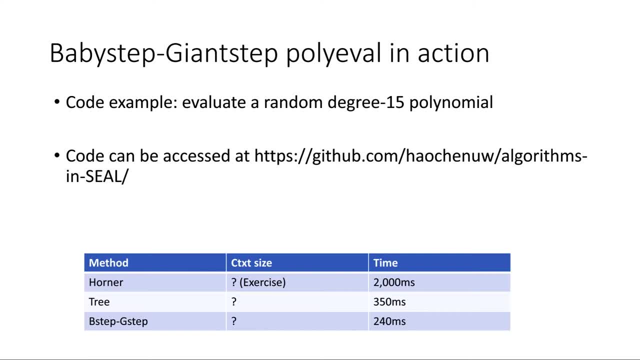 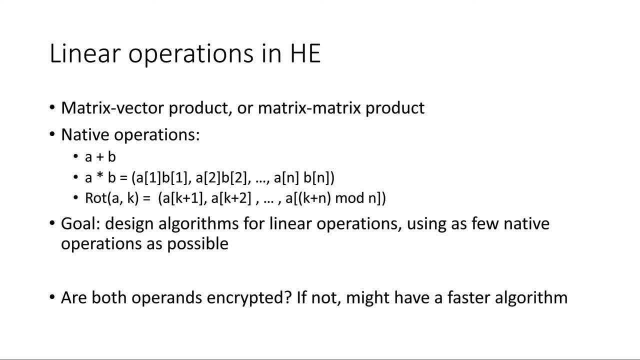 required for this application. Okay, For the last topic I will talk about is this: linear operations in homomorphic encryption. So, if we go back to this example of logistic regression, we're computing some sigmoid which we approximated, and we have some good algorithms. 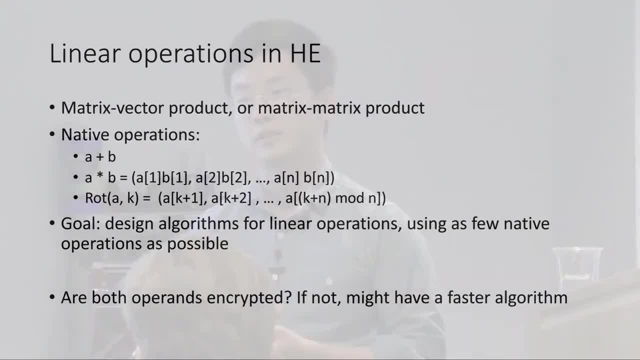 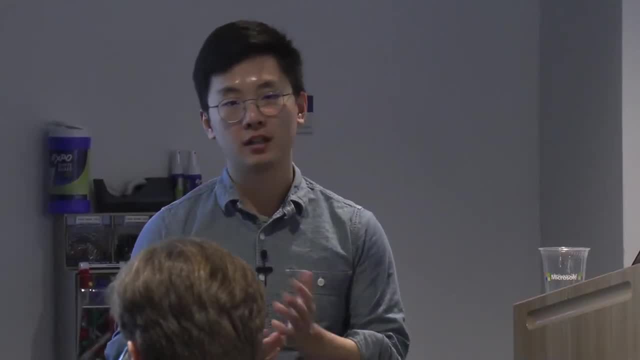 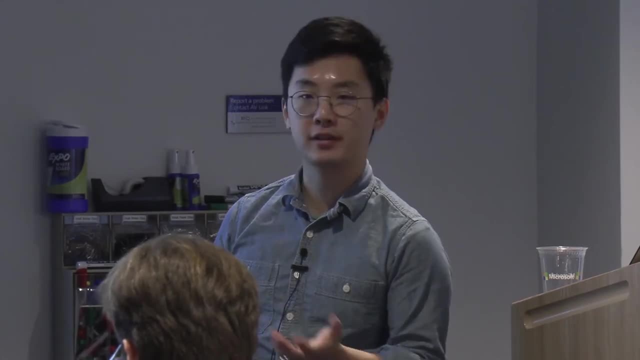 But what about this matrix vector product or even matrix-matrix product? So we only have these three types of operations, but none of them directly gives us matrix vector product, for example. So we need to have algorithms for these linear operations using as few native operations as possible. 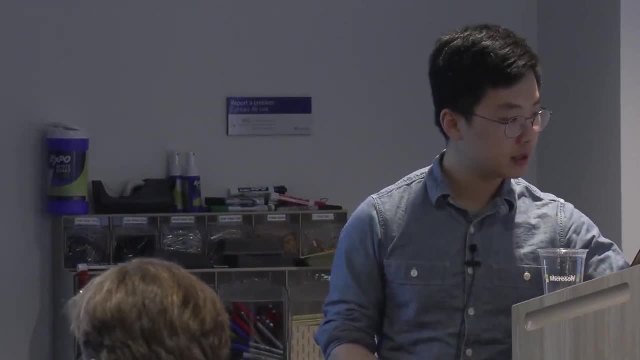 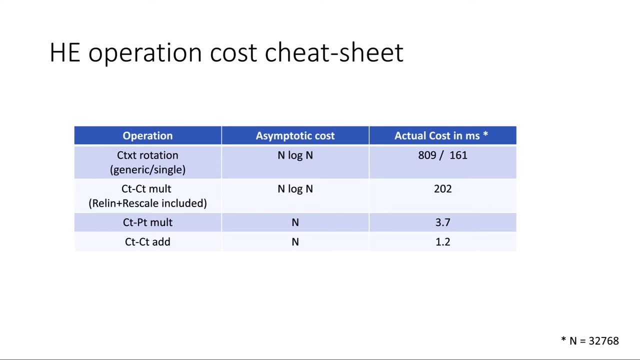 And let me go back just for a second to this cheat sheet where you can see that it's possible that if you can use this ciphertext rotations, then a lot of the functionalities can be achieved. But we need to keep in mind that this is like an expensive operation. 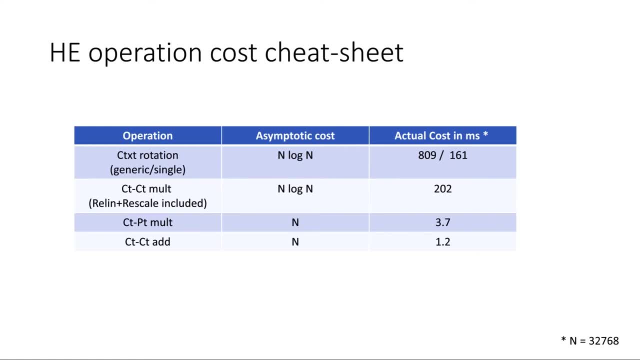 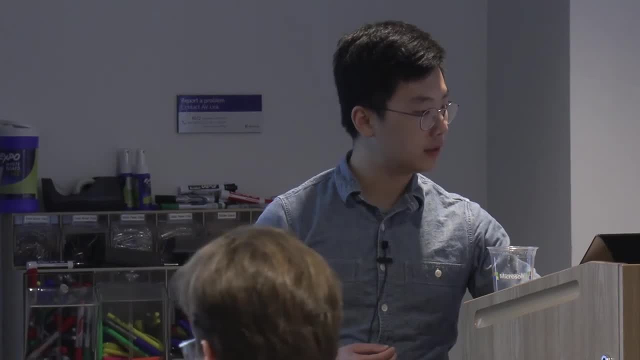 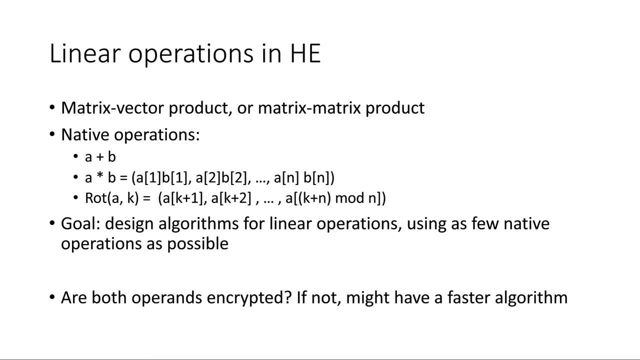 So what we want to do is to reduce the number of ciphertext rotations also as much as possible. So now let's go back to this question of doing this linear operations So oftentimes. also, observation that we made is that if you have encrypted, 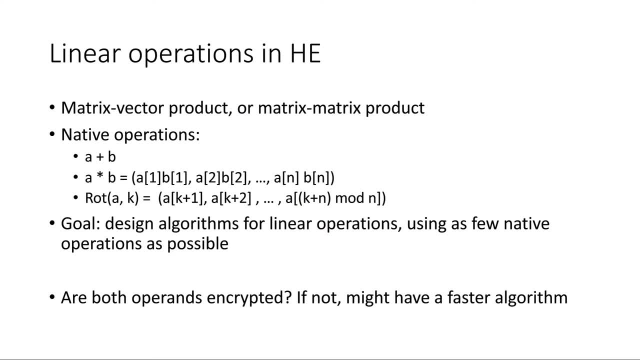 vector times encrypted matrix. that's often more costly than encrypted vector times plaintext matrix. In the latter case, you can somehow design your algorithms by just arranging the matrix in a good way so that the operation is even more efficient. So it might be good to think about whether you have that kind of ability. 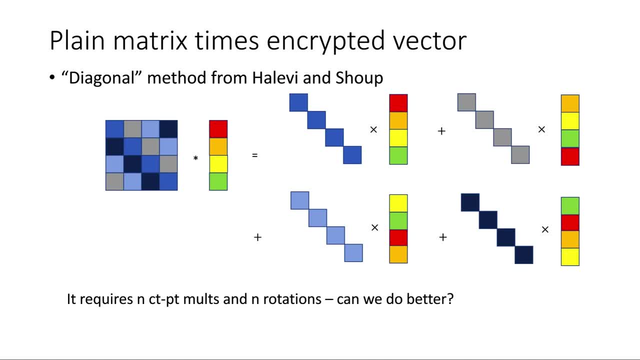 So let's talk about what we would do when there's a plaintext matrix multiplied to an encrypted vector. So, just for simplicity, we can think of the case where the matrix is square matrix. In that case there's this diagonal method which basically operates in this way. 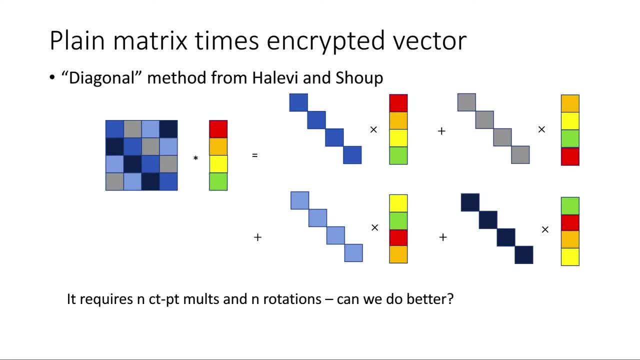 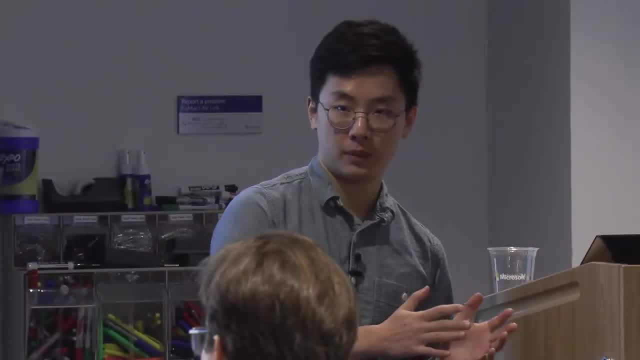 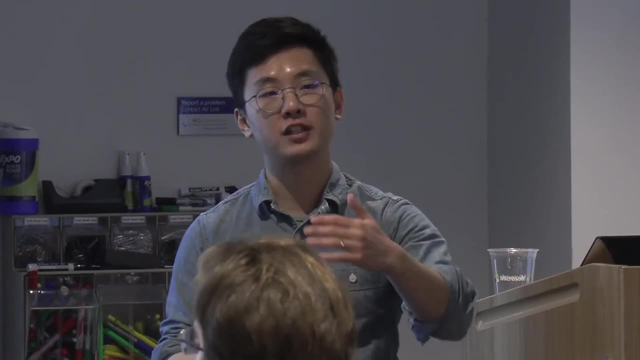 So you have a plaintext matrix and each of its diagonal is encoded into a vector. The reason of this procedure is because later we will try to multiply this vector to an encrypted vector in a coefficient-wise multiplication way. Notice that if you consider the main diagonal, 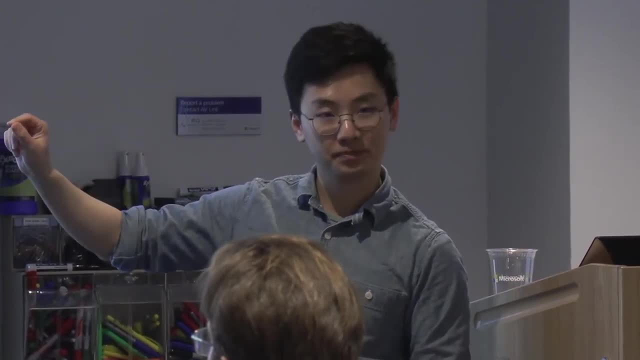 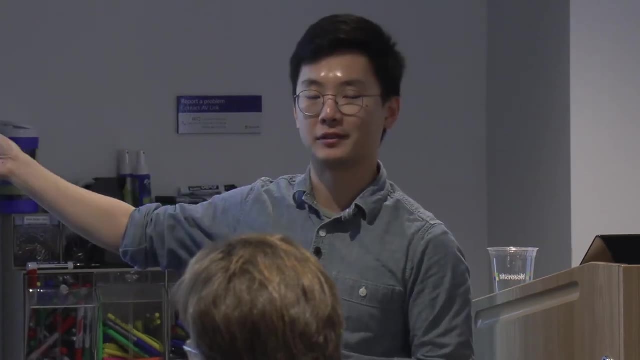 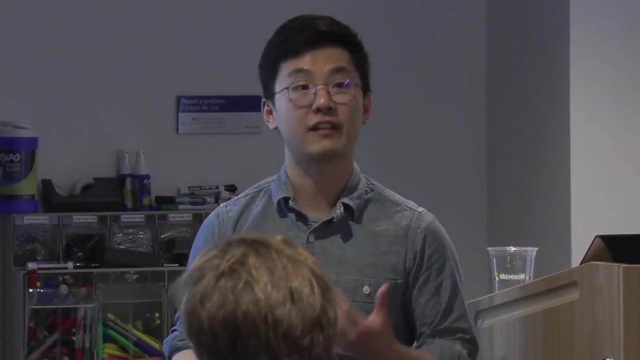 then actually the first element of that main diagonal is going to multiply by the first entry of the vector, and the second one will be multiplied to the second entry of the vector. So then you keep the structure of the multiplication by not wasting any effort in this coefficient. 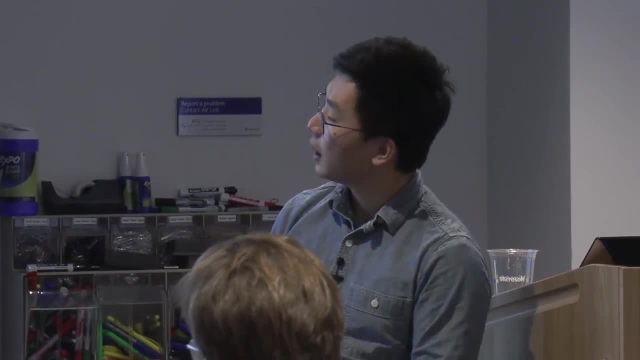 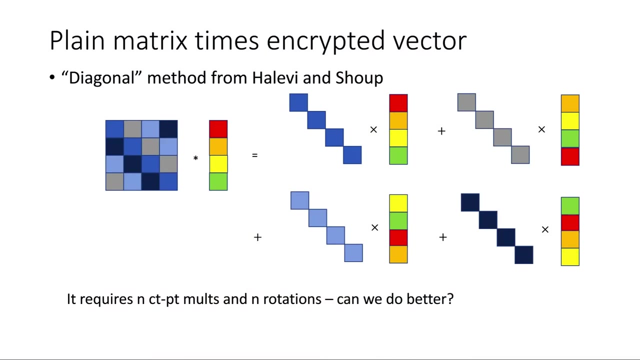 It's a coefficient-wise product. So if you have a four by four matrix times a four by one vector, this naturally just involves n- ciphertext, plaintext multiplications and n rotations, Because we need to rotate the encrypted vectors by the 0,, 1,, 2, and 3.. 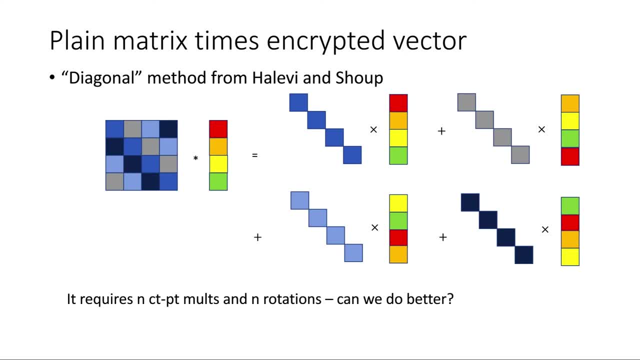 So in this picture you have this vector encrypted, starting with the red, and when you need to rotate it by one, it starts with that orange. So seems like a pretty good algorithm because we didn't even waste any multiplication. But in this case, 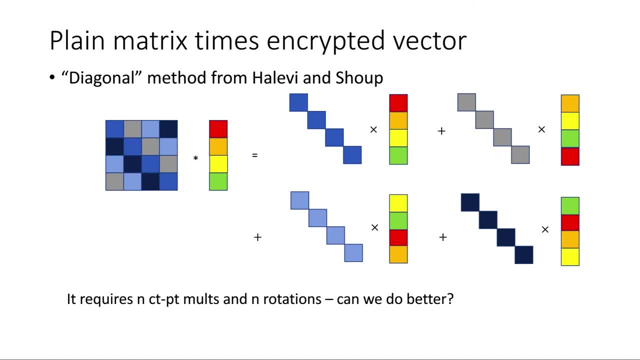 we need to do n rotations, But remember that if you were to implement this algorithm in a plaintext, then you don't need to do any rotation because you just simply do your multiplication and that's it. So kind of of this additional n rotations is. 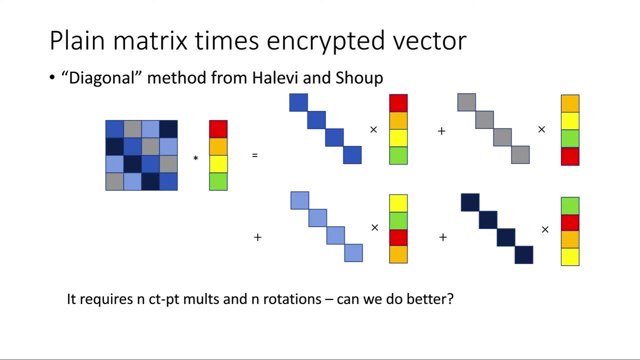 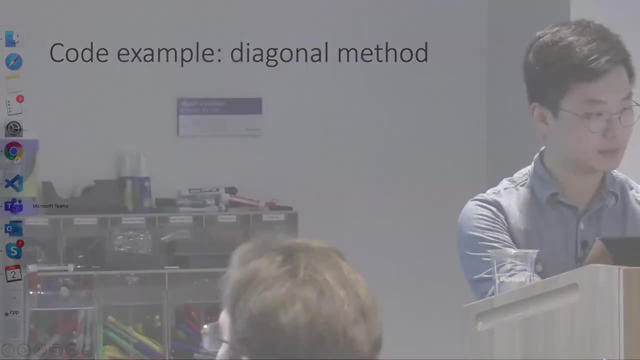 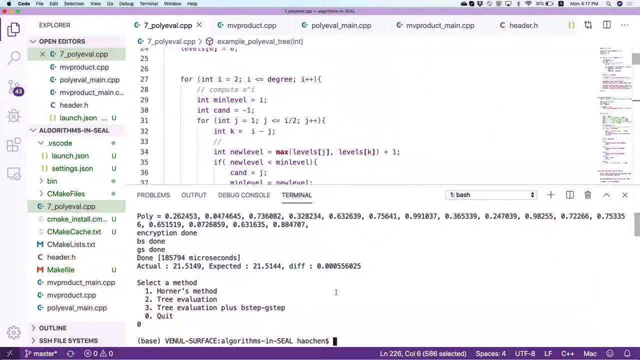 additional overhead that comes from using this he So, and actually we can do better to reduce this number of rotations, And let's talk about that. But before that maybe I'll give an code example of that diagonal method. So it's the same repository. 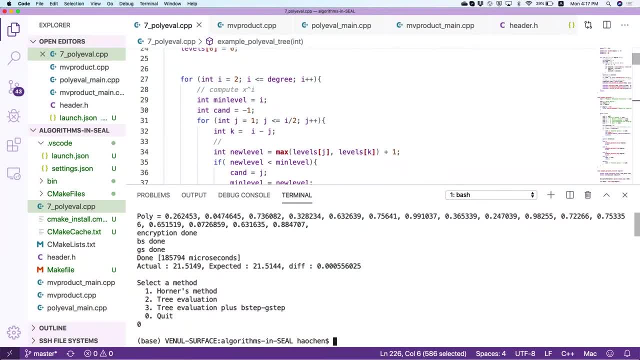 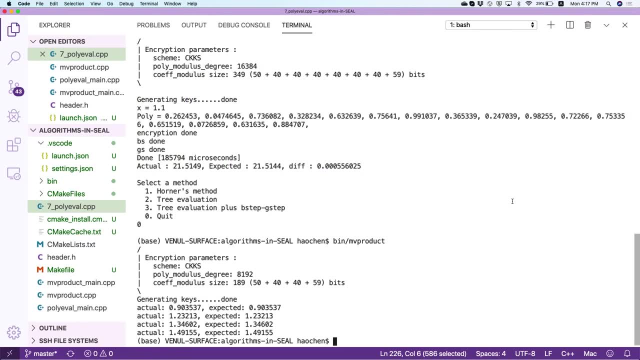 but if you do, I think it's called mvproduct. So what this one does is that it will generate randomly a matrix and a vector and it will encrypt that vector and compute this encrypted version of m times v and it will decrypt that and compare that with the plaintext result. 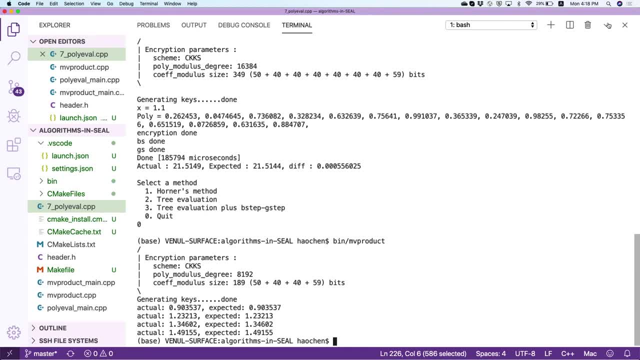 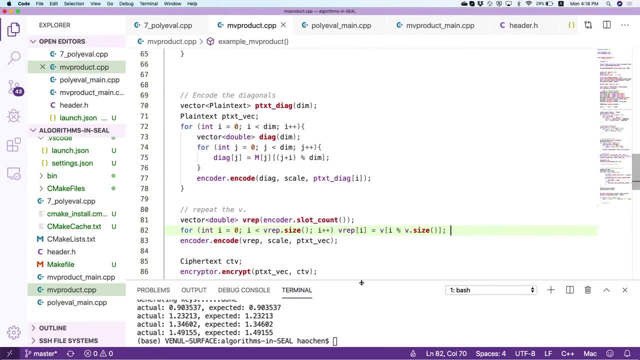 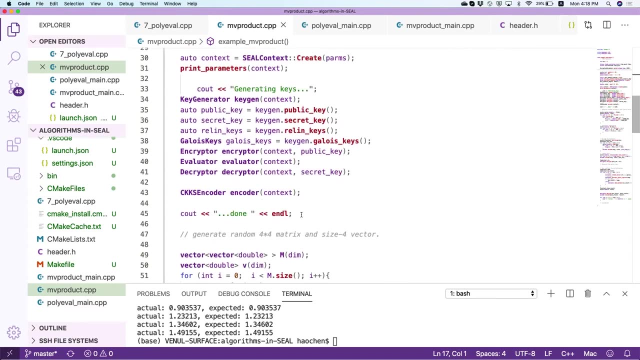 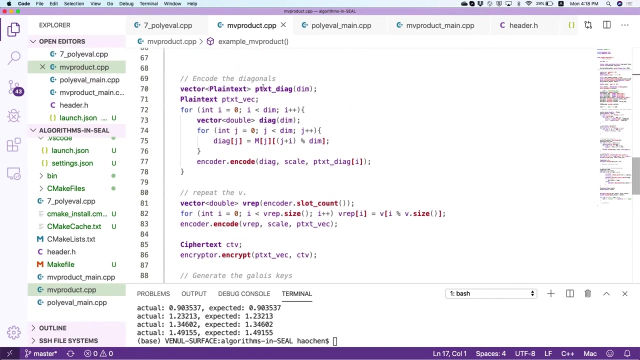 So also I'm going to show you some examples. Also I'll show you that code. So the code starts here. So this one is not super sophisticated, because what you do is basically you set up this plaintext. 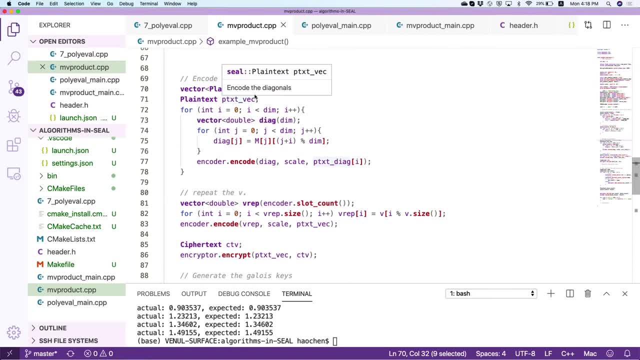 which supposedly encodes the diagonal soft matrix. Yes, what I'm doing here is basically setting the entries of this plaintext to the corresponding diagonal elements and then finally do an encode to encode them into this CKKS plaintexts. Then I encrypted this V vector. 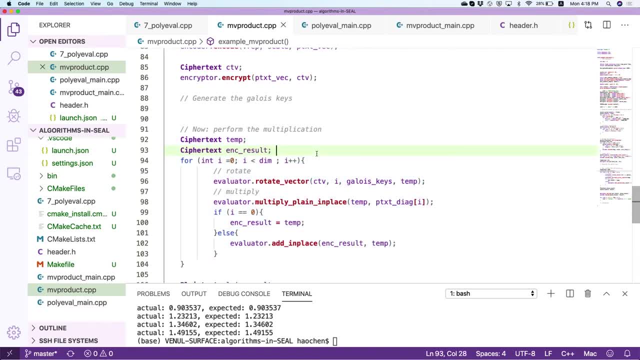 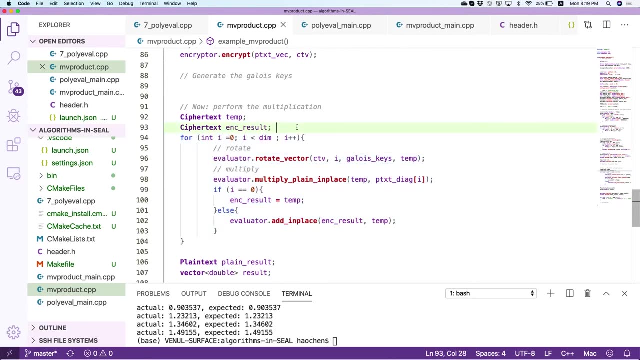 So the action just happens here, where in each step of the iteration I rotate this vector by I steps and then I will multiply that with the corresponding diagonal. There's a song, So this one, I think, is also in the repository so you can check it out. 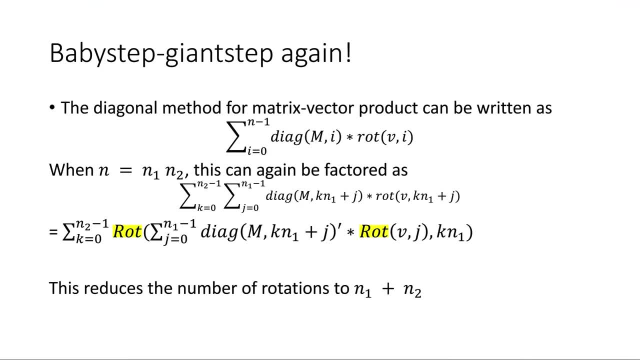 Okay, So now let's talk about the optimization. So it's surprising that we can also use this simple baby step, giant step technique to reduce the complexity of this operation. So remember, what we're doing is that we're computing this sum of different diagonals of the matrix. 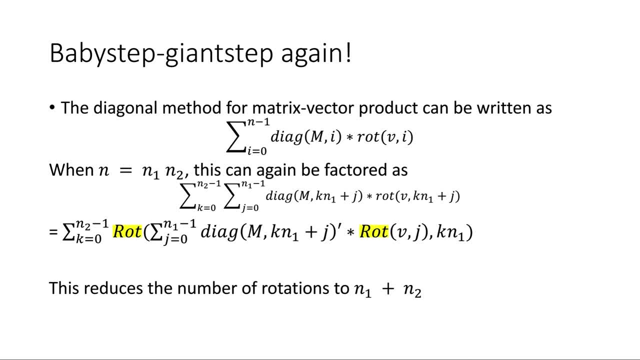 times the different rotations of the vector. So you can also factorize this as a double sum. when the number of entries in the vector can be written as N1 times N2. Then we can actually pull out this rotations to be applied to an inner sum. 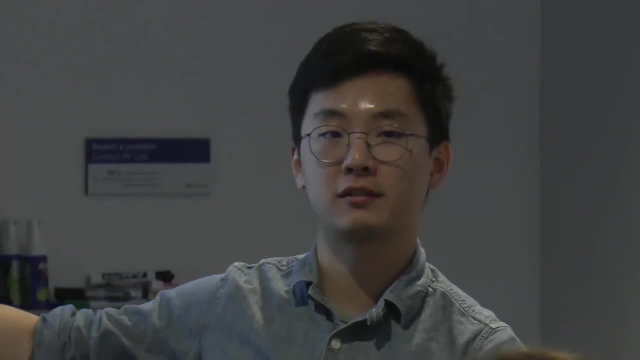 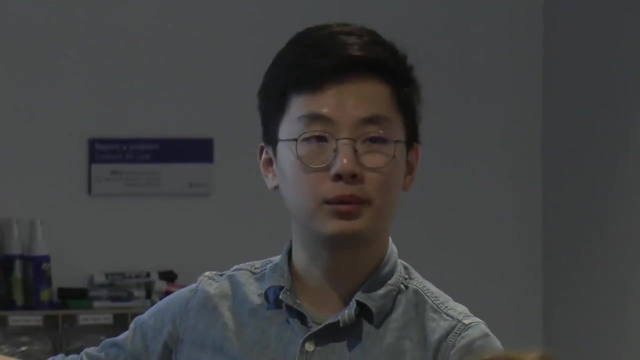 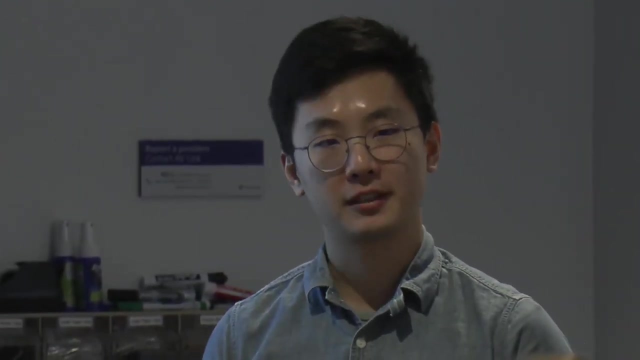 So now this rotation only needs to be done once for each of these items in the inner sum, Which means that we can just use N1 plus N2 rotations to do the whole computation without having to use N rotations, and that actually saves a lot. 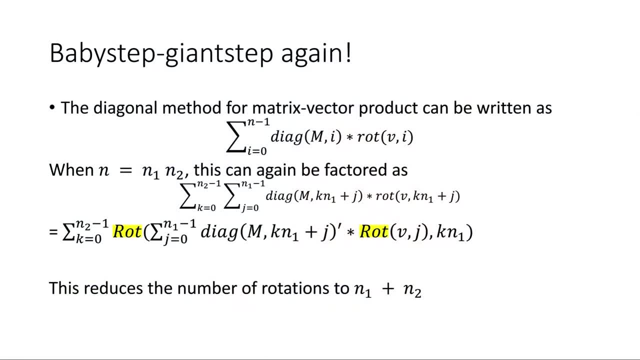 So I don't have a concrete code example for this, but I think it's a nice exercise to try to code this up. I think it's another example to illustrate that with a lot of these H-sheet computations it comes with some overhead, but it's possible that by some interesting arrangements. 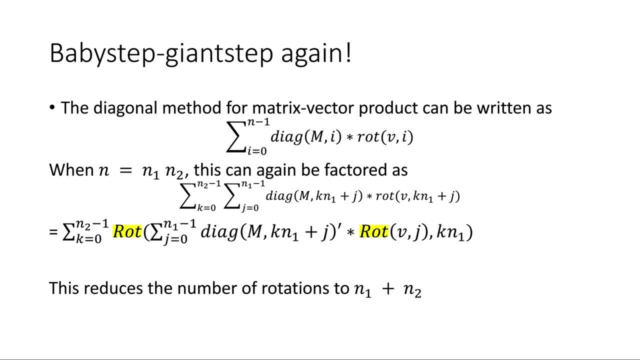 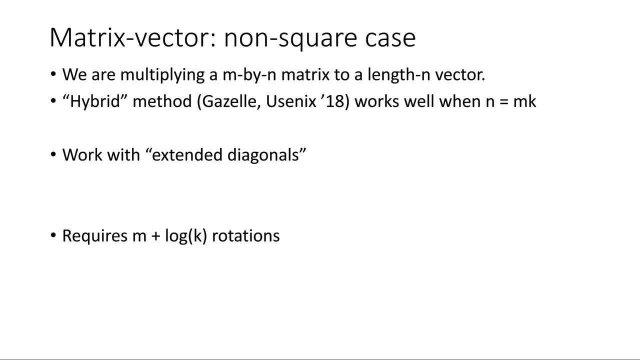 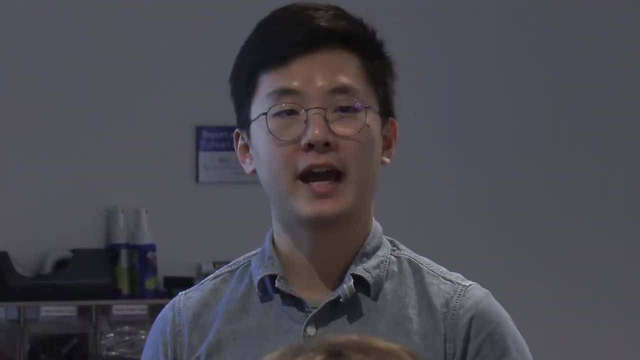 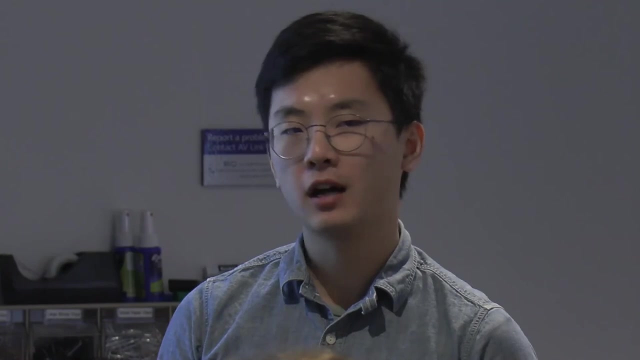 we can remove this or at least reduce the overhead. Okay, So the previous method works when the matrix is square. So you may want to ask that what happens if I have a general rectangle matrix? So I think right now the situation is complex because there 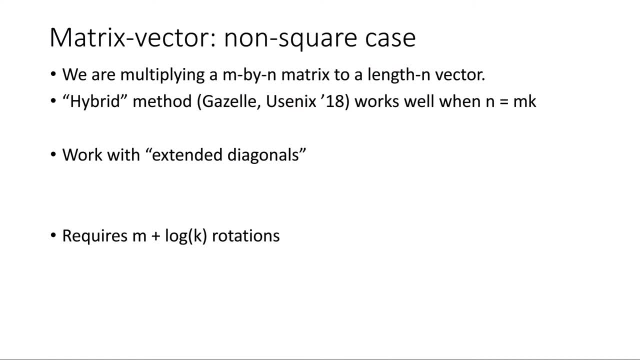 isn't one algorithm that works and it's the optimal for all the possible matrix sizes that you can come up with. This is also partially due to the limitations that also the CKKS scheme, for example, and the particular parameter choices in SEAL gives you only powers of two vector length. 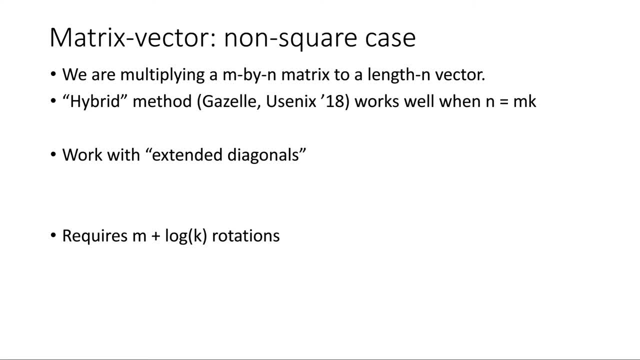 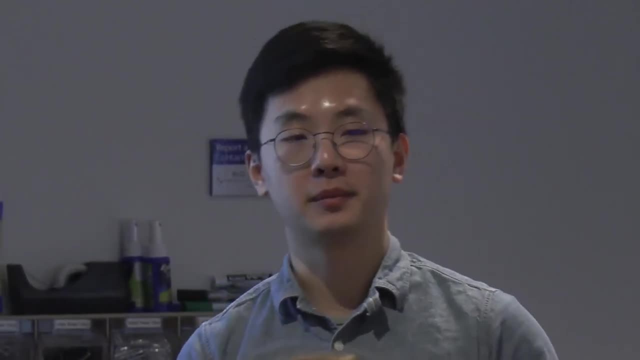 But fortunately, I think, in the special case where you have a matrix which has more columns than rows and suppose that the number of columns is a multiple of the number of rows, then there's a hybrid method which uses this diagonal method a little bit and gives you good efficiency. 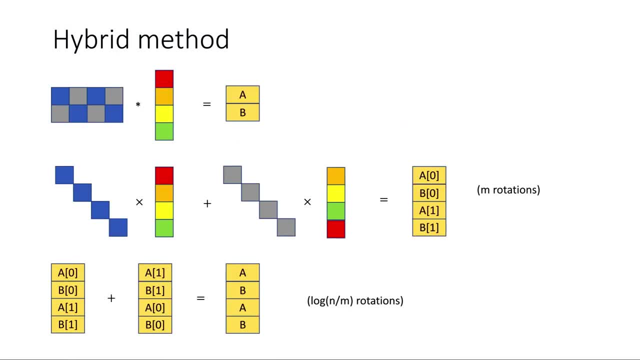 So let's look at that. So now suppose you have a matrix times a vector and instead of a four by four matrix you have a two by four, Then what we could do is to extend the notion of diagonals and encrypt four entries inside one of the 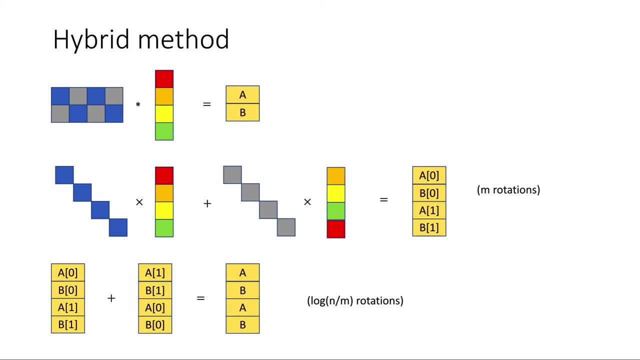 sorry, not encrypt. encode four entries in this one vector and then we're still not wasting any of the multiplications. by just doing one rotation I can compute all the necessary products. But now the problem is that I got this intermediate results, which is some kind of partial sums. 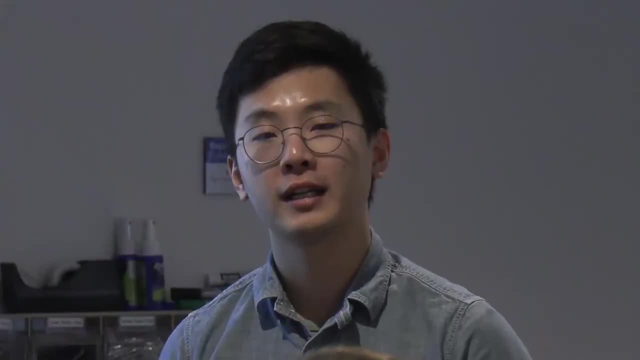 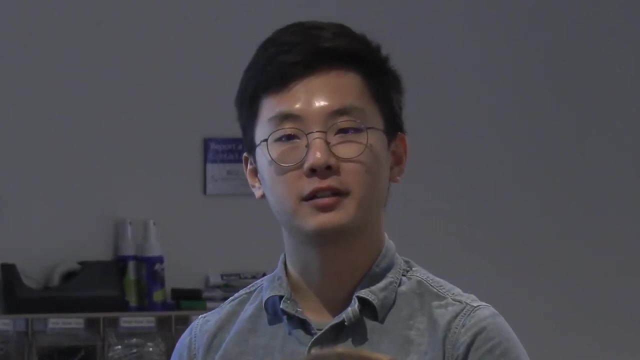 and then these partial sums needs to be aggregated further in between the slots in order to get the final result. So the difference here is that now the result is only a vector of size two. Here it's represented by the two numbers a and b. 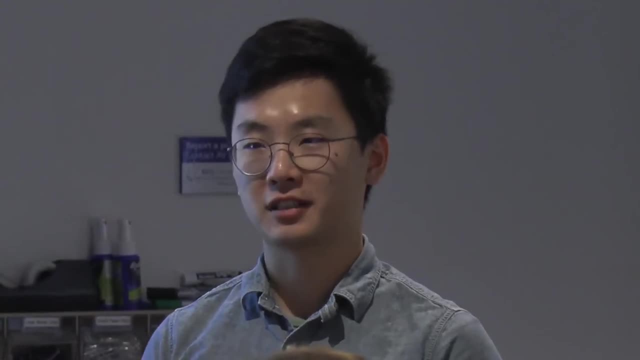 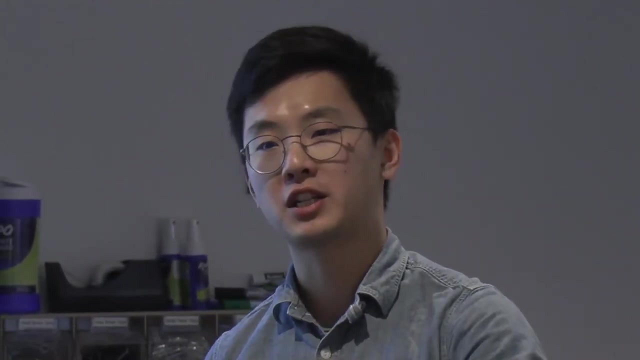 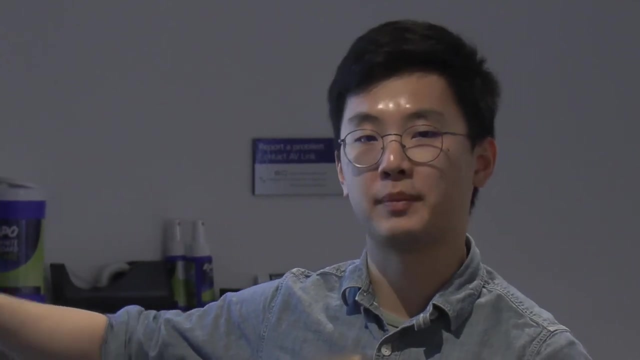 But now I have four slots, So each of this slot contains some partial sum about this a and b. So what I need to do further is to do a rotation and summation. Fortunately, because you have this power of two structure, you can do this summation of all slots in log, number of rotations. 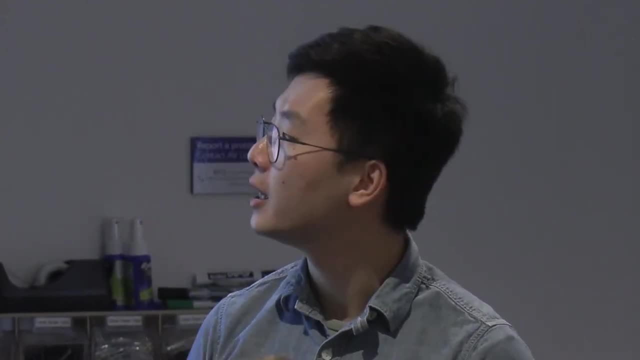 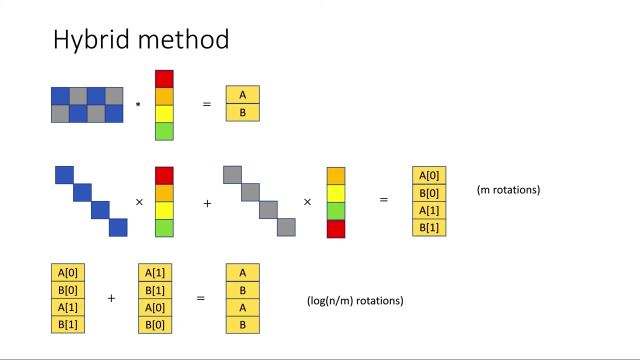 So it will be interesting to work out the details, but this is actually much better than the naive implementation of a matrix vector product. Notice that in all these cases, the primary goal is to reduce the number of rotations, which is supposedly complex. 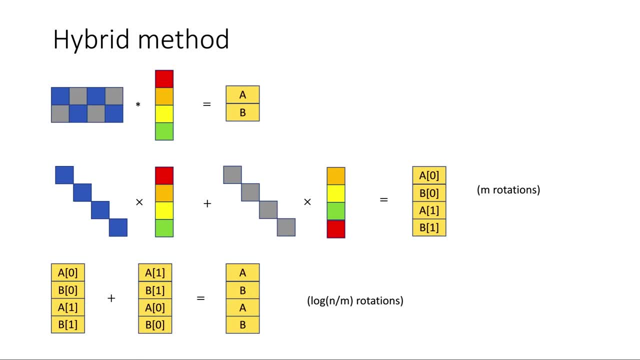 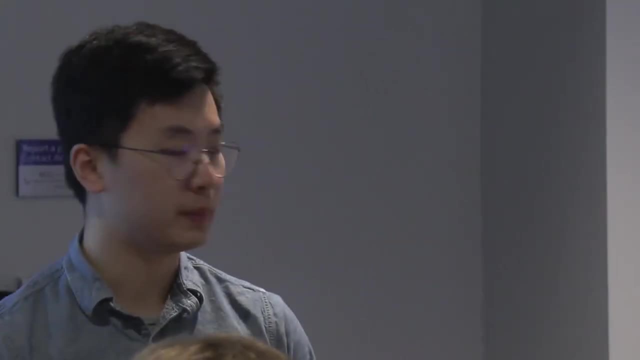 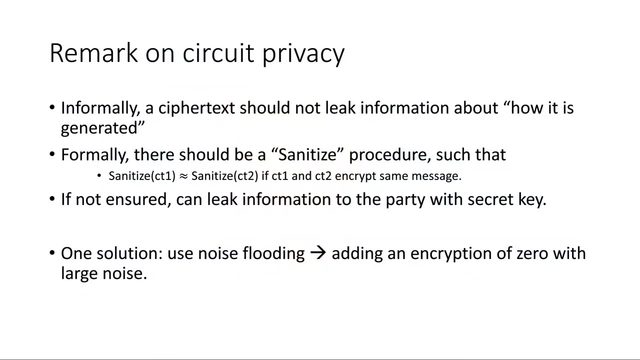 So I think these are all of the algorithms that I wanted to cover, and I wanted to use the final few minutes to talk a little bit about some side comments. So first of all is the remark on the circuit privacy. So this is not a meaningful notion if you're only using 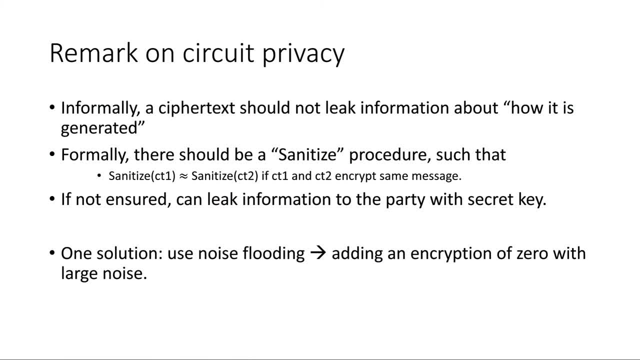 the homomorphic encryption for outsource computation, because then the computation is known to the secret key owner already. So for example, if I'm the only data owner, I just want to offload my machine learning computation to some server and not doing that computation myself. 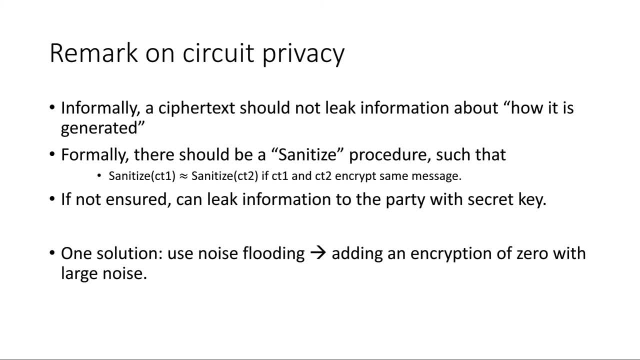 then it's okay because the function that I supposedly want to evaluate is known to me. So, even though in the end it's leaked, it's perfectly fine. But it could potentially be a problem if you're designing applications using homomorphic encryption that involves 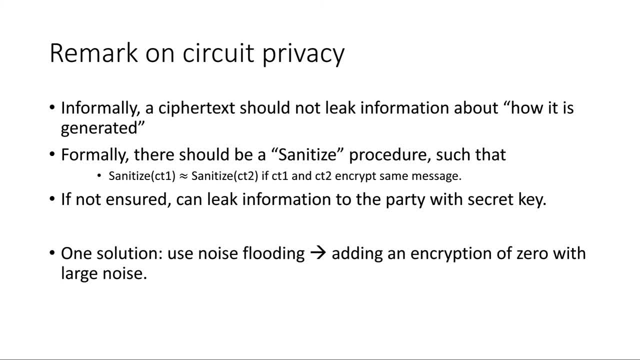 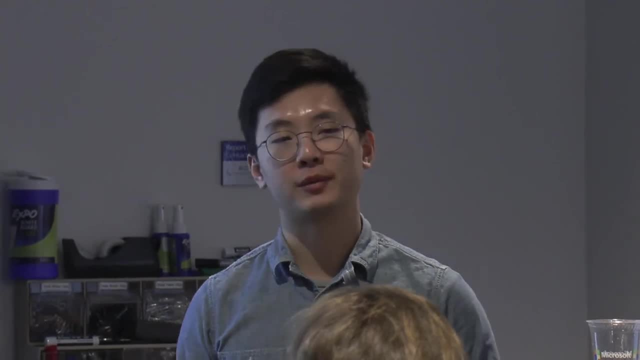 sensitive data from two different parties, for example. In that case you might be thinking that it's possible to just let the other party perform this plain-text ciphertext computation, But then the resulting ciphertext might contain some information about the plaintext even beyond what you are supposedly learning. 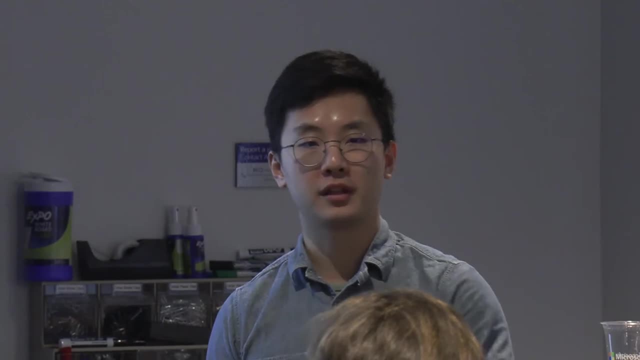 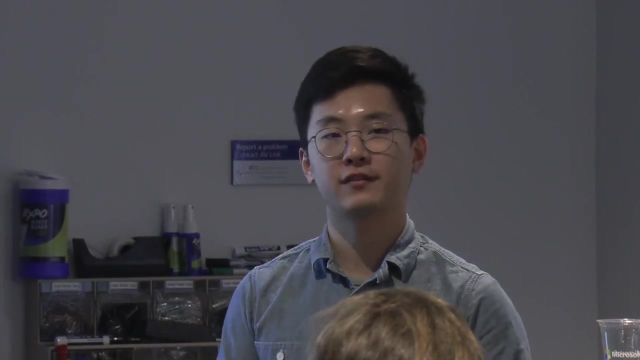 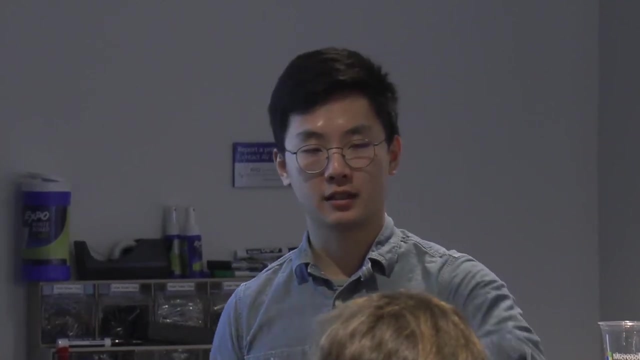 So this is interesting problem, both in theory and in practice, and I think there are no very satisfactory solutions to this. There is kind of like an efficient solution of just adding some noise. If you add a large enough noise, then you can prove that. 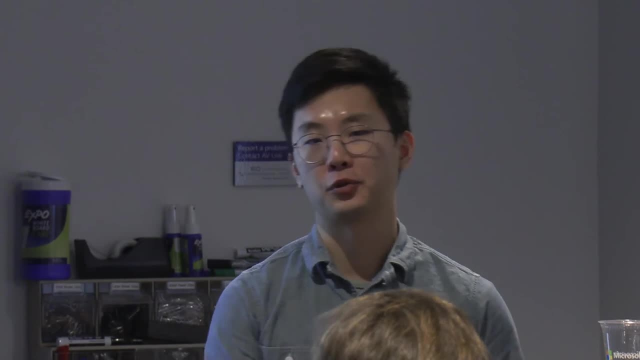 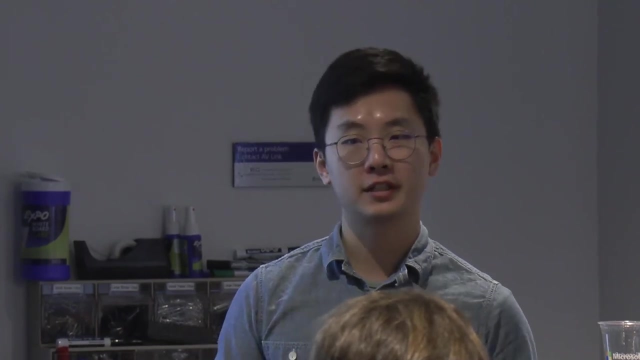 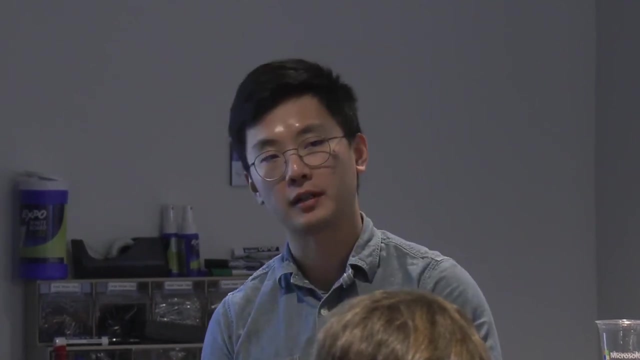 this other party's sensitive data isn't leaking through this additional noise, But it's kind of a weaker guarantee, only statistical, so that in the future, if we want to use this for two-party kind of applications, we may want to think about how to manage this issue. 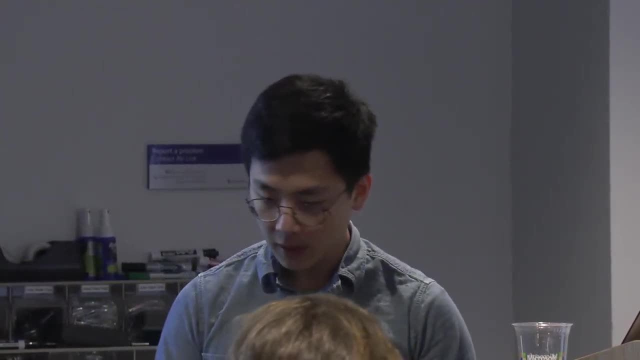 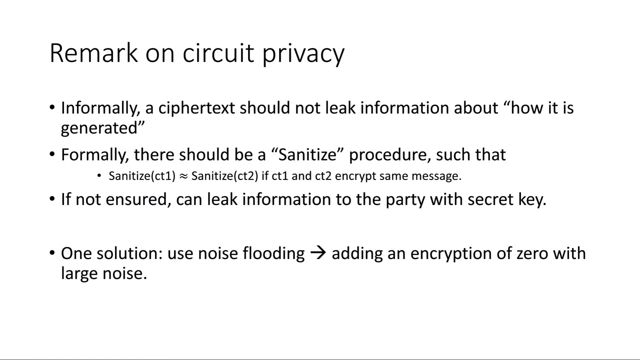 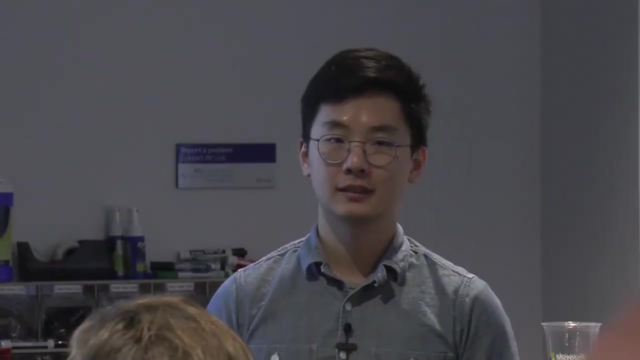 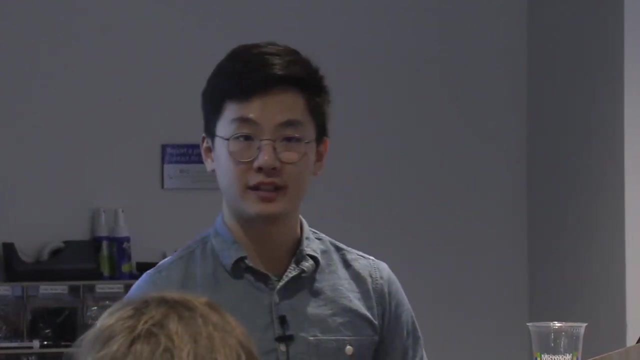 Then I think I can conclude by identifying some of the yes For the previous case. if we transform the whole computation to be oblivious, we still have the same problem. So the question is that if your computation is oblivious, would you have the problem? 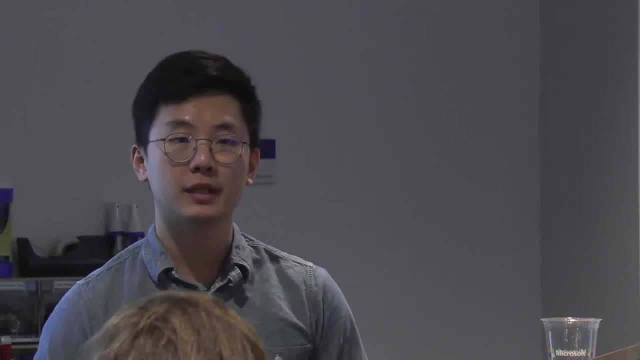 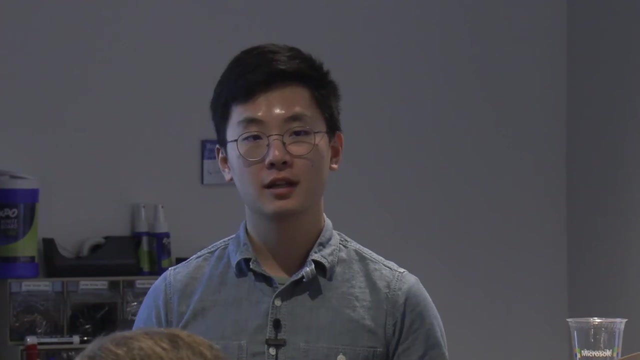 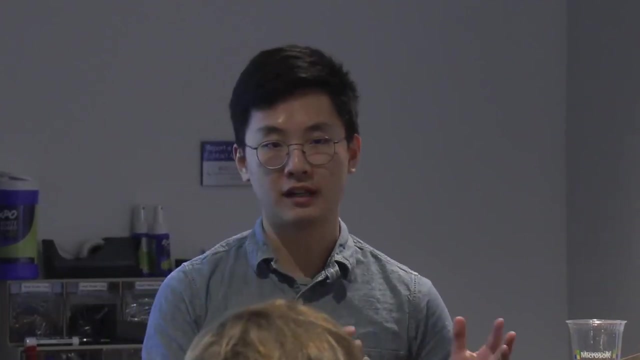 So yes, in some cases, because even though you can say structure your computation as a circuit, sometimes the circuit comes with certain constants and those constants can be sensitive data of the other party. So it's important that the final ciphertext of the evaluation result doesn't leak anything about. 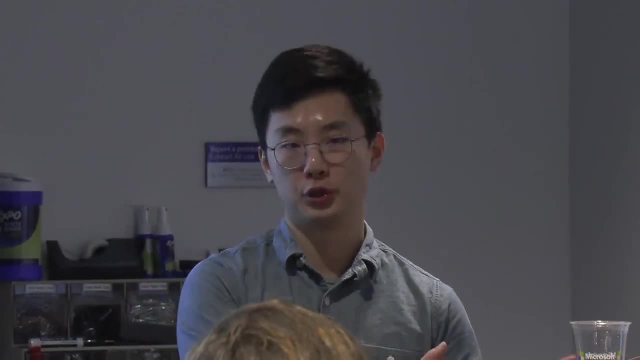 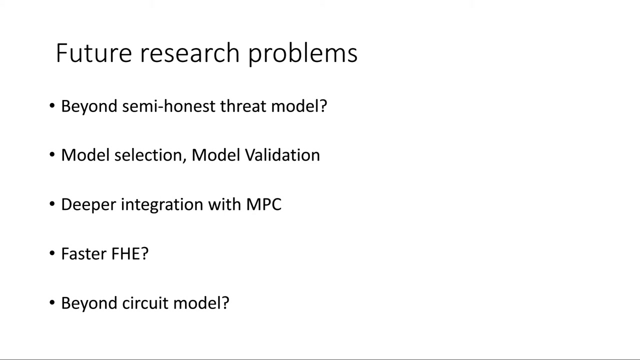 these constants other than the output of that circuit? Okay, So I wanted to identify also some some further research problems of HE. So some of these questions are kind of far-reaching goals, but because I know also there's a lot of people working in this area. 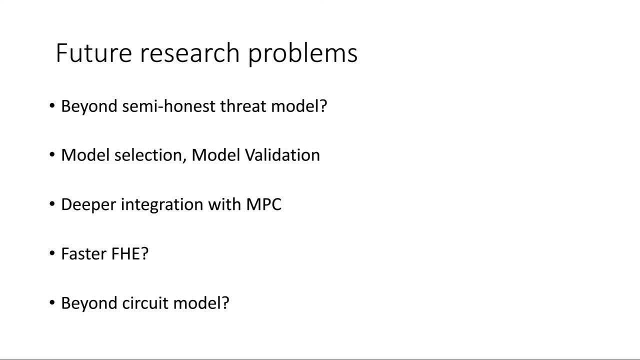 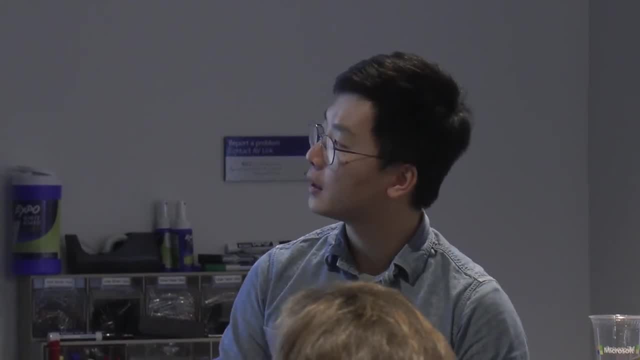 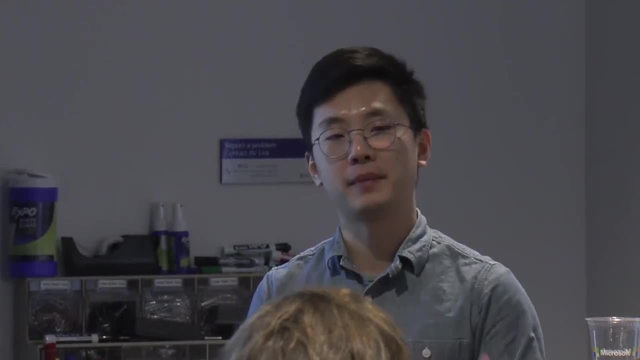 so I wanted to just single them out. So first of all is that: is it possible to have HE beyond the semi-honest model? For example, we could think about adding some guarantee where even you have a malicious evaluator you can still make some guarantee about. 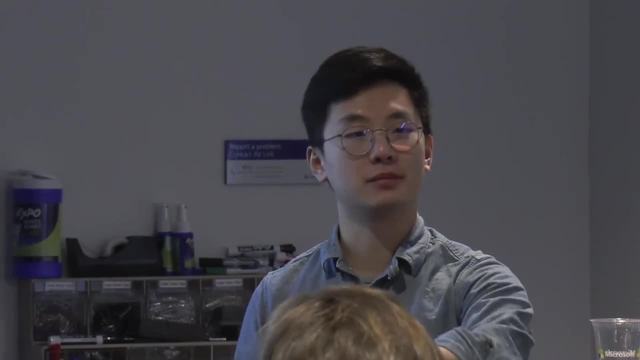 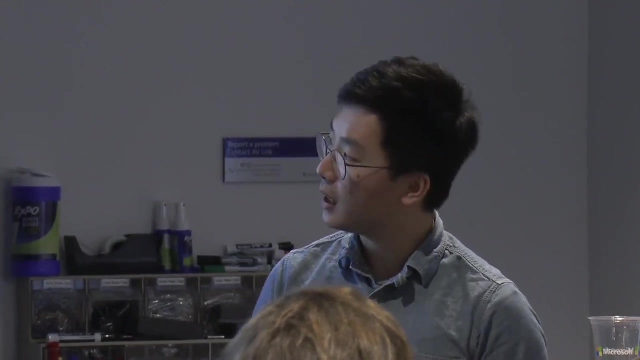 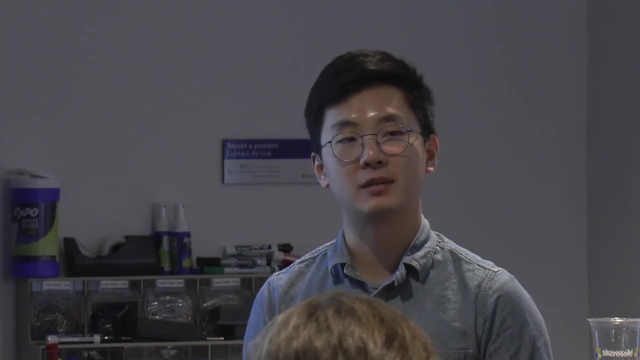 the final ciphertext doing kind of reasonable computation. Second one is that in the case of privacy-preserving machine learning, usually in the machine learnings, there will be some kind of preliminary steps where you decide which model to use and after the training. 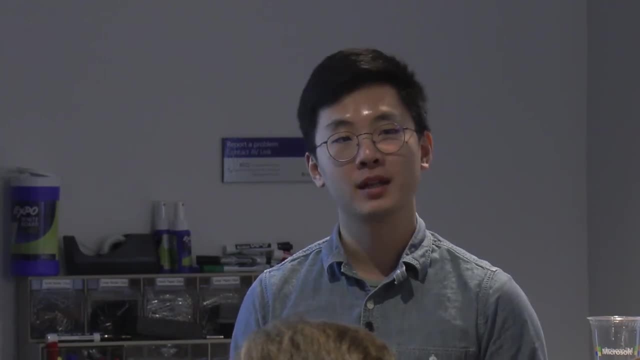 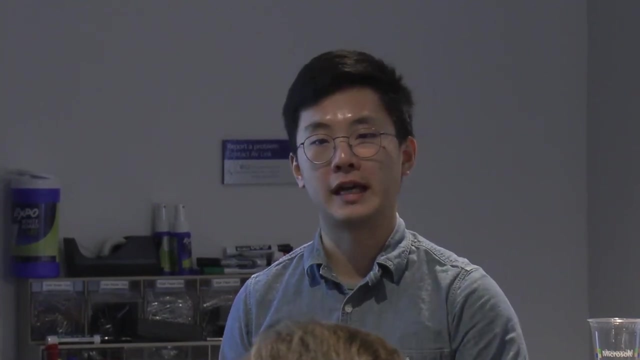 you will try to validate the model using some of the test data, But this is not clear- at least a 100 percent- how to integrate these into the HE framework. So I think this was also briefly mentioned in Arun's talk- that if you want to do some kind of retraining, 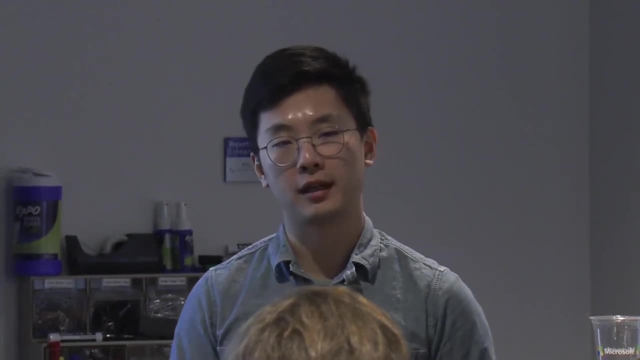 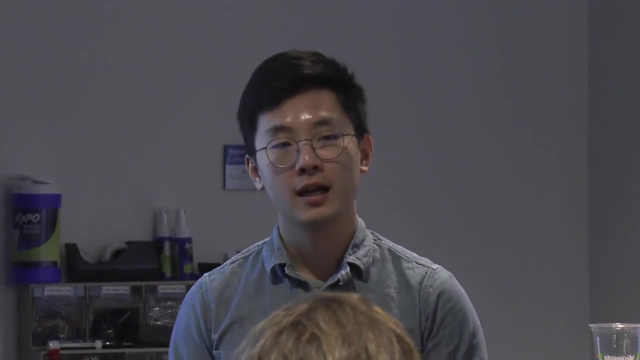 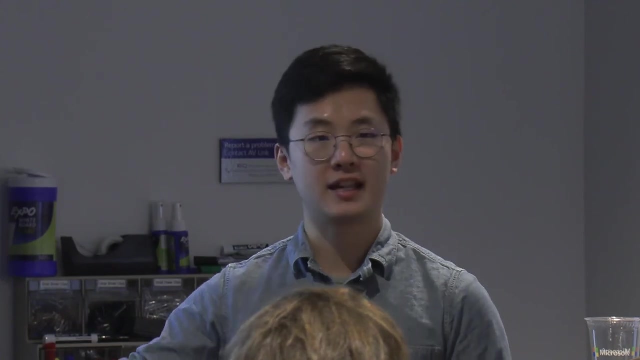 it's not entirely clear that how you would go about doing that using the HE, Because HE is kind of you have- you need to specify the computation in the beginning. So if you're doing some training, then you need to specify the step size and how many steps you're taking. 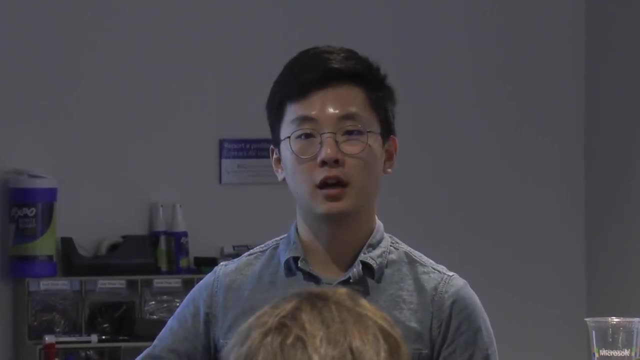 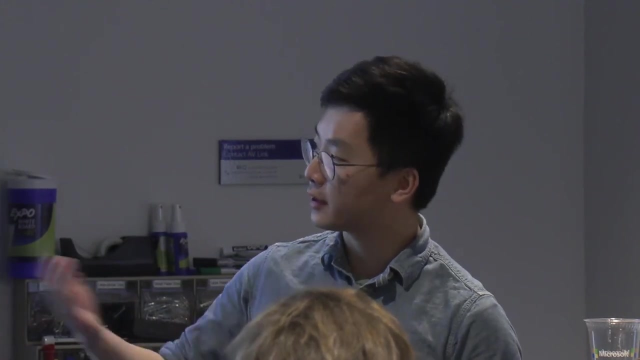 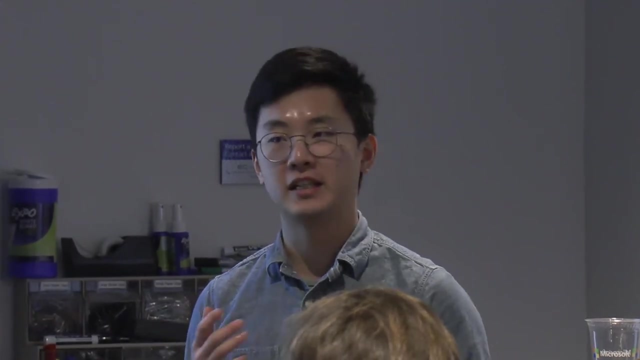 and these things are often decided, at least in the plain text case- you decide that after you have taken some look at the data. Another question is whether we can have a deeper integration with MPC. So I think there are some words in combining HE with MPC to design fast end-to-end solutions. 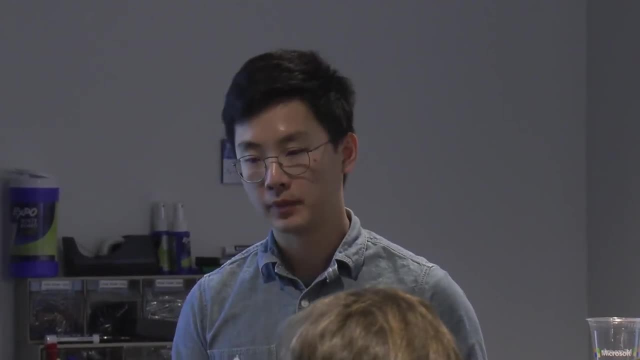 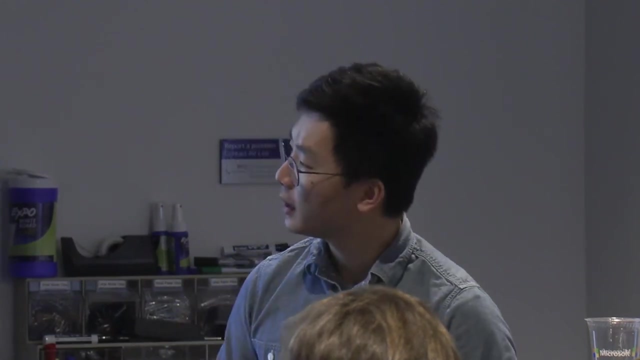 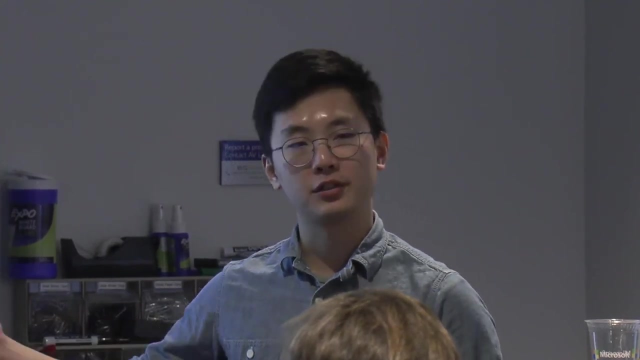 But I think there could be some more efficient ways of integrating them, like providing the good connectors of these two primitives, and I'll skip that faster FHE part. and the last one is what I wanted to talk about more, which is right now all the HE and MPC. 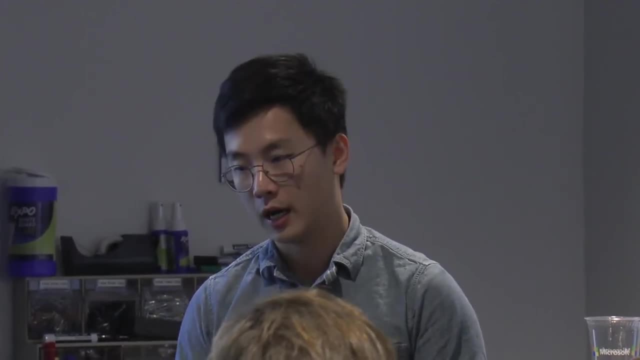 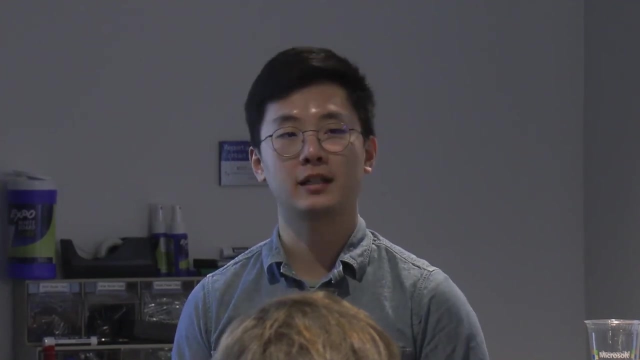 and I think even some of the zero-knowledge proof primitives- deals with the circuit model, which means that we have to structure our computation as a circuit, whether it's binary or it's arithmetic. So that's great, But I think also a lot of 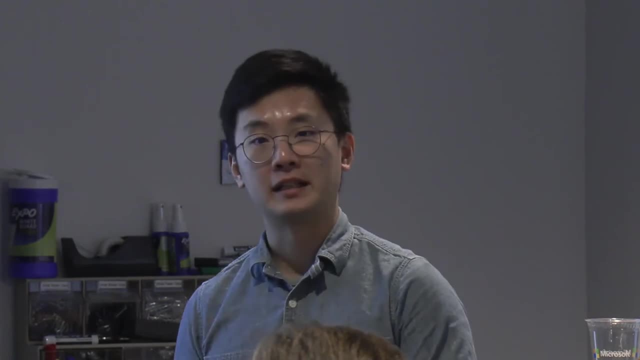 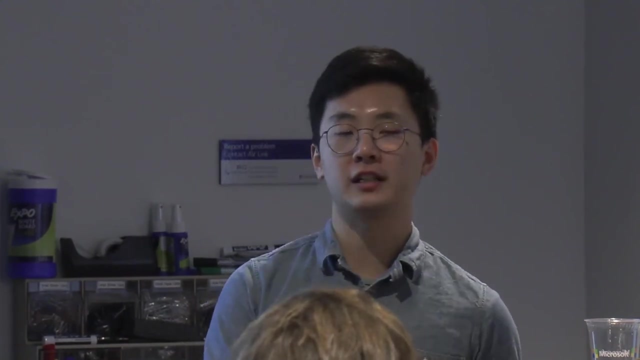 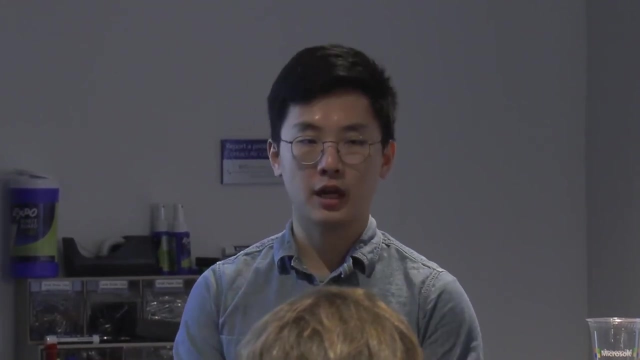 the computations that people actually do in ML. at least it's not so much of a fit into the circuit model. or if you fit it in a circuit model maybe there's a big expansion of the cost. So I'll say one example. 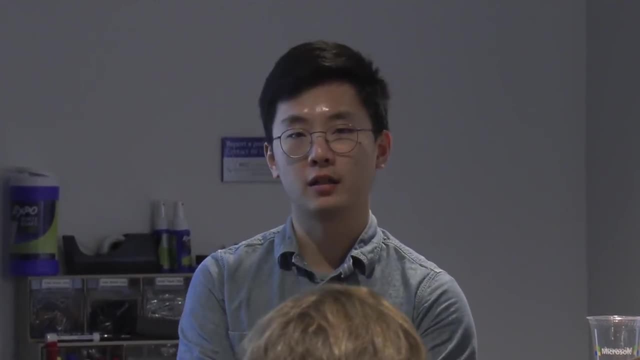 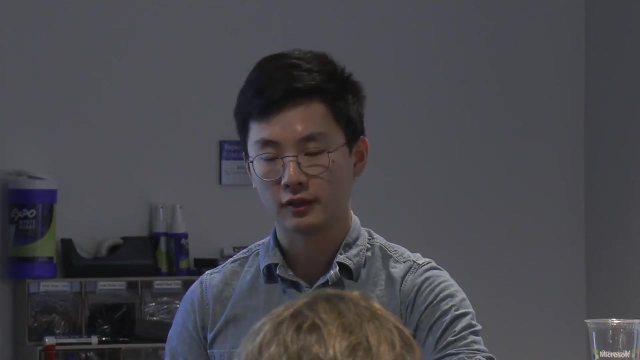 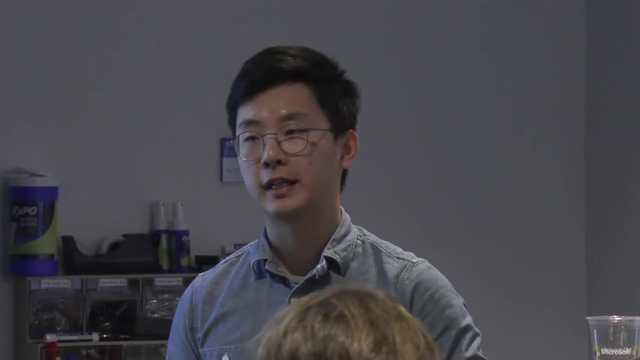 So there could be a lot of algorithms that train decision tree or a random forest where there could be a lot of training algorithms in ML which has a stopping criterion. So the stopping criterion usually can be expressed as you have a model after several steps of training. 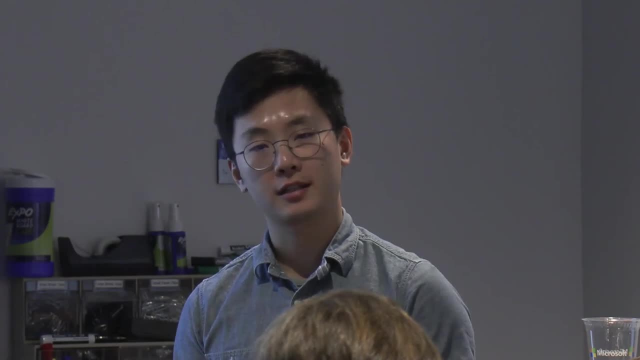 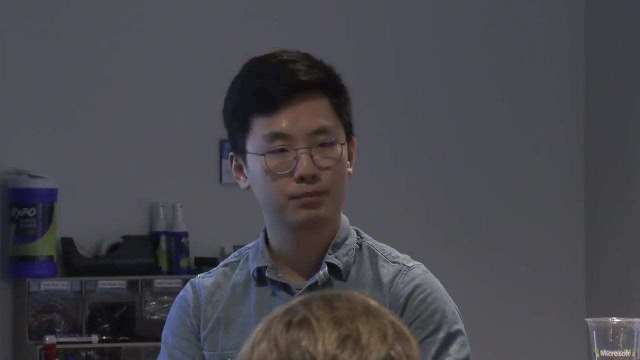 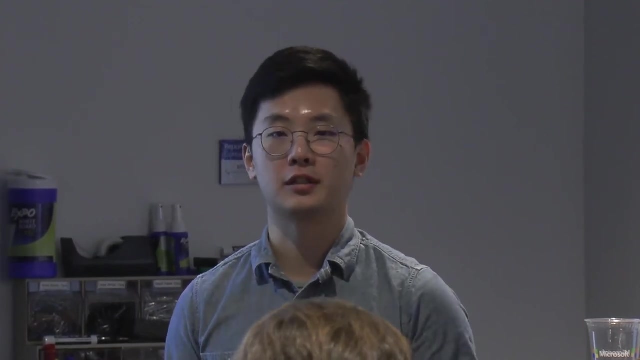 and you check some criterion holds or not? If it holds then you will stop the training and if it's not hold, then you will keep going, possibly modifying some of the parameters or not. But doing this branching is hard to do in a circuit, as we might know. 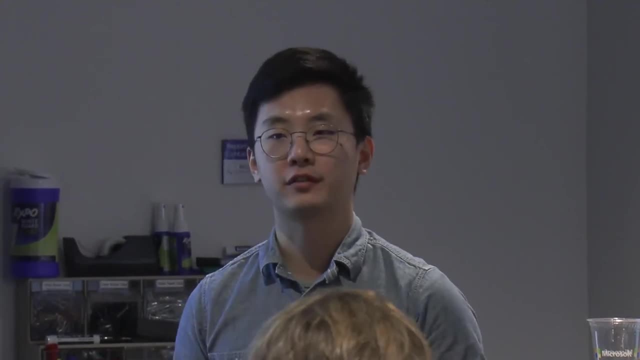 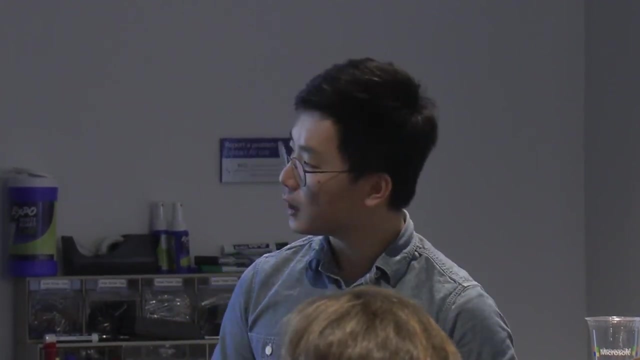 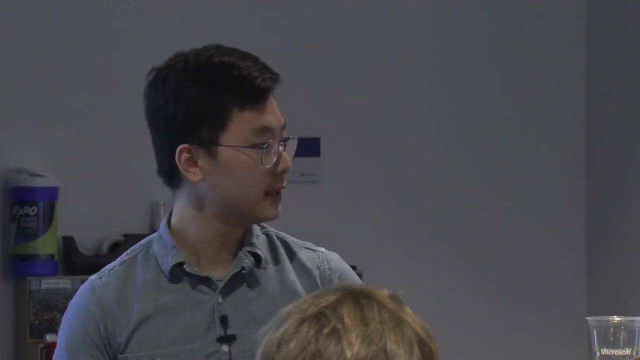 So if you want to preserve the full privacy of the data, it doesn't actually save you anything because you have to evaluate the both branch. So this one, I think it's an interesting question to think about also. So I will stop here and have this slide up. 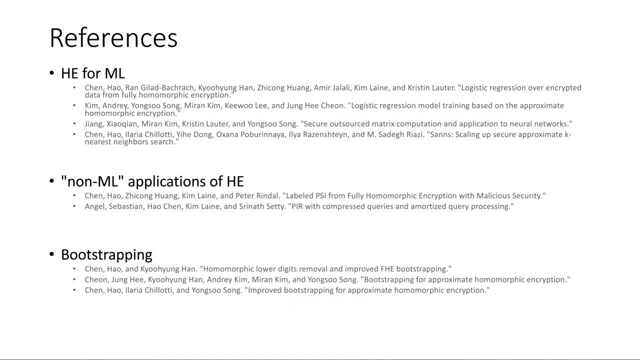 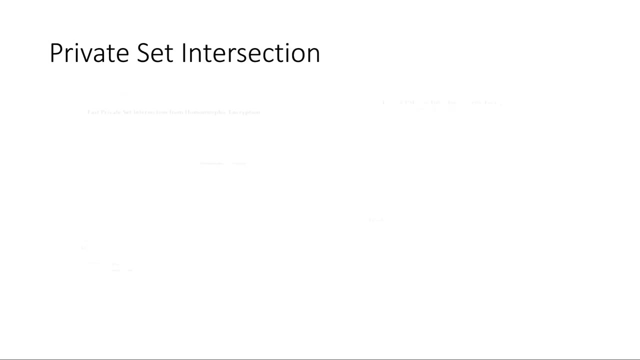 for some references to a certain paper And some links, and I'm happy to take questions. We'll publish the slides online anyway, so you don't really have to take the pictures. Those are in small fonts anyway. Do you have any questions? 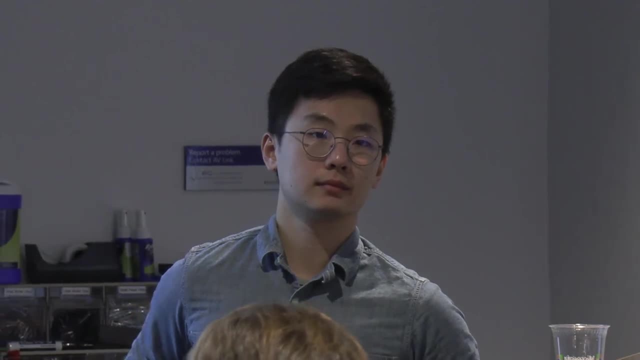 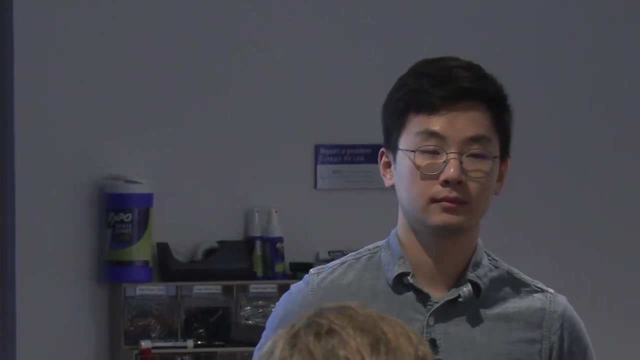 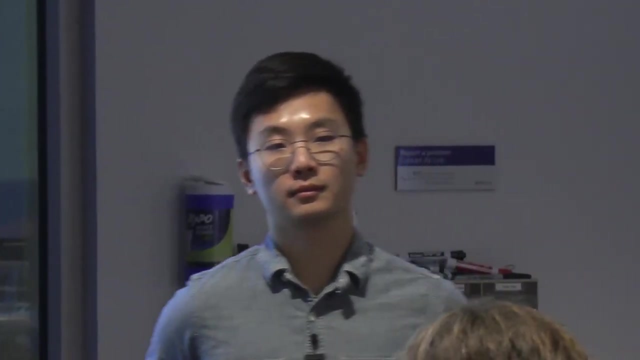 So this semi-honest threat model, it seems like a bit weird, to me at least, because how would you distinguish between, say, the server, for example, how would you distinguish between a server that uses a good model versus a server who simply like, oh sorry. 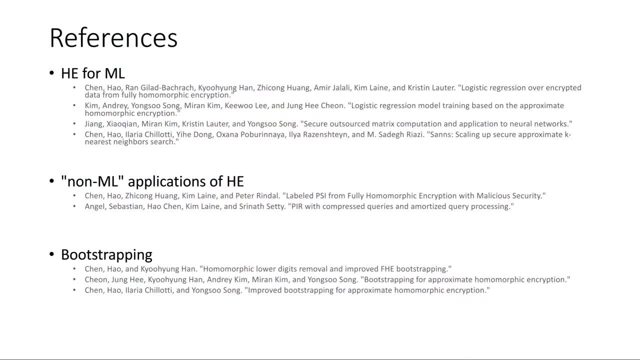 How would you distinguish between a server that simply uses a bad model and a server that deliberately uses a bad model? Yeah, So that's a good question. I think at least that's not a question specifically for HG, It's kind of an issue also for MPC as well. 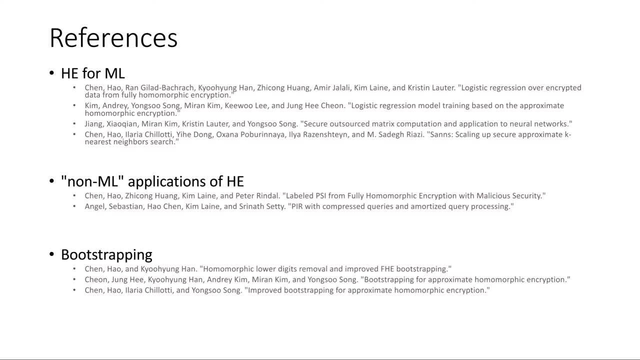 where you can check that input data is valid, which means that it's between certain range, But you can't check if that is a valid model or it's some random data, Right, Sorry? So, for example, like in MPC, at least, 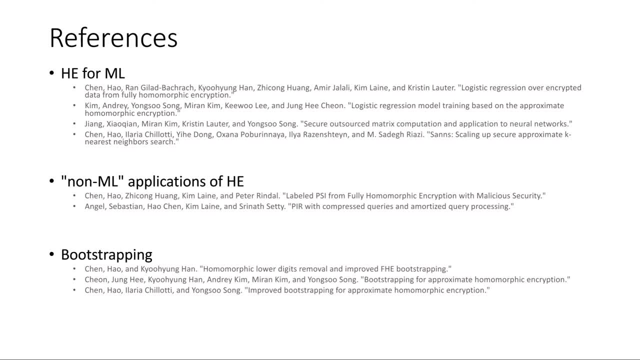 you don't really deal with input substitution, which is like it seems like that's the only attack you can do, as, like a malicious evaluator say, in the FHG- Yeah, Yeah, FHG- setting. So I think we can separate two cases. 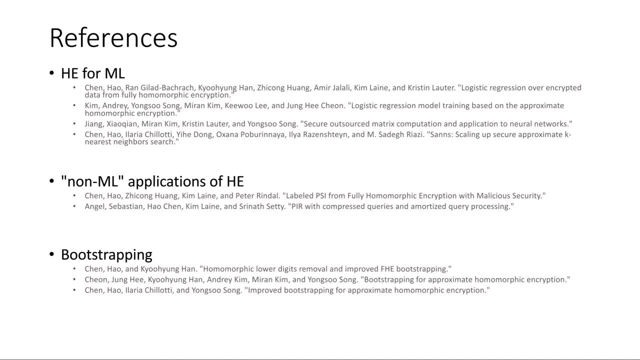 One case is the attack that you mentioned by just I can just input random data to the computation. The other one is that suppose the computation is kind of expensive, then the malicious server can just not do any computation. So by doing this, 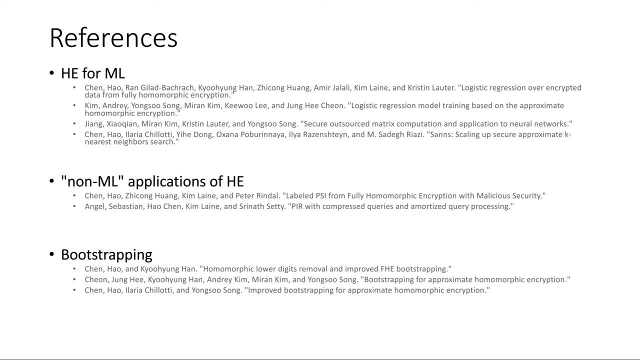 it has motivation to do this because it saves some cost, Right? Okay, So you're saying like: just encrypt this is a cat or something and then send this back, Yeah, Where you can just like not do any evaluation but encrypt zero, or 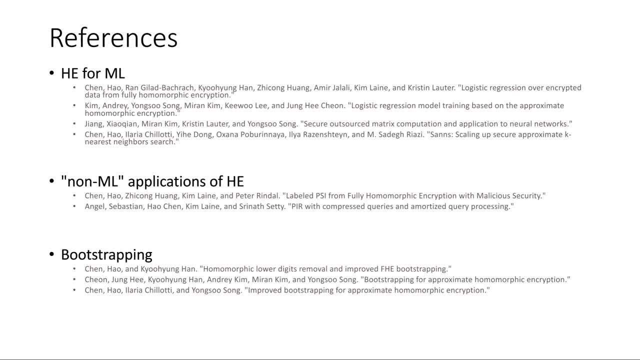 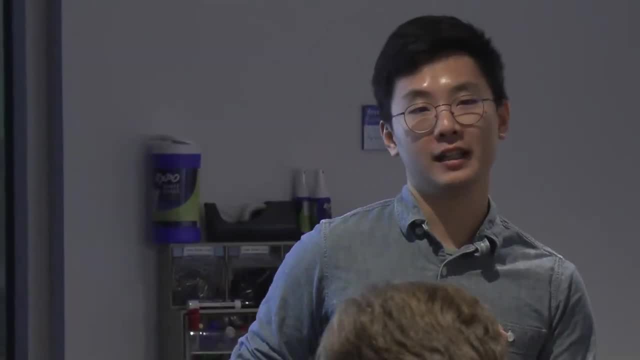 Right. But that seems to be like sort of the same thing, right, Because I could have a model that is just like terrible and just says, like this is a cat to everything. Yeah, That's true. So I think what could be done is that, after you get the result, 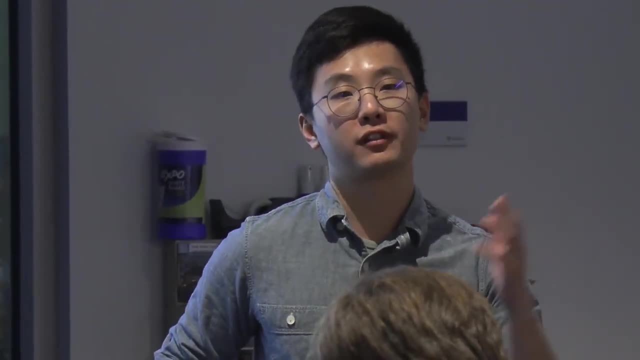 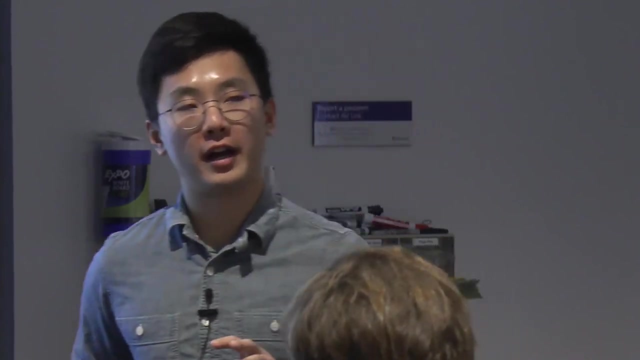 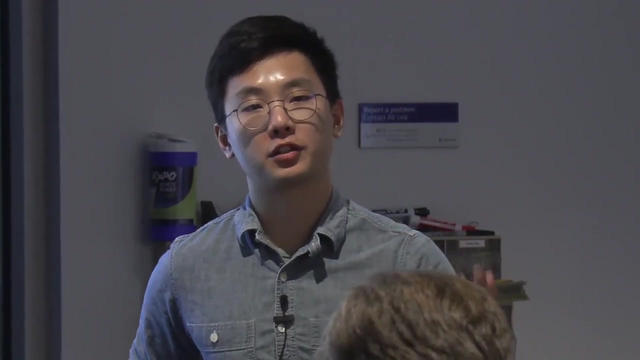 if there are some way to use a different channel to validate the result, then it kind of kind of can help with that. But first of all I think we should have a way to ensure that the server is evaluating, kind of executing certain given computation. 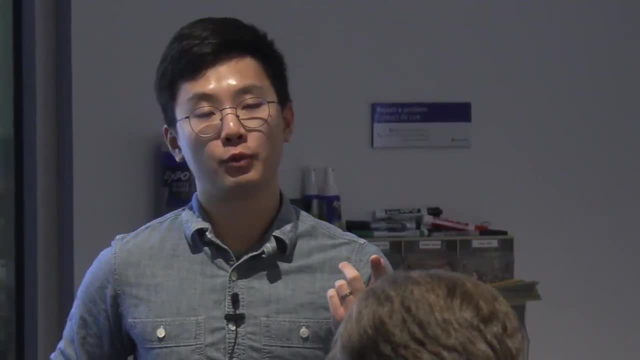 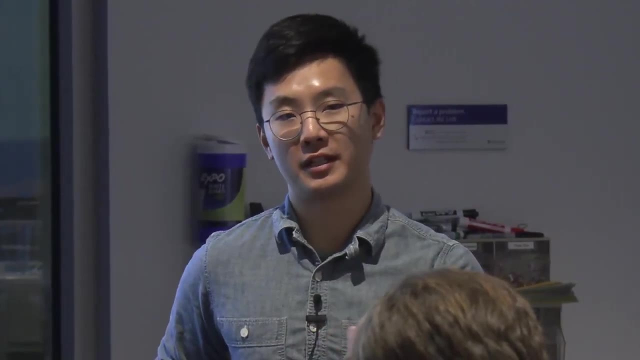 So this makes sense, for example in the outsource scenario, where the server doesn't have like a private model as input. So suppose I just have like a huge computation that I wanted to outsource. then I want the server to be able to verify to. 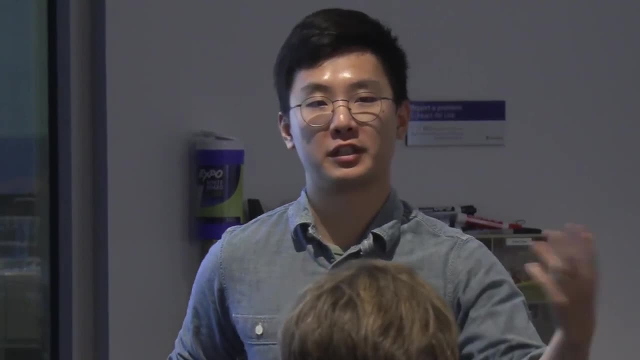 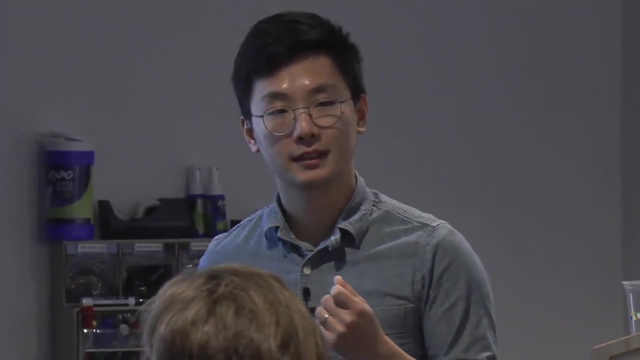 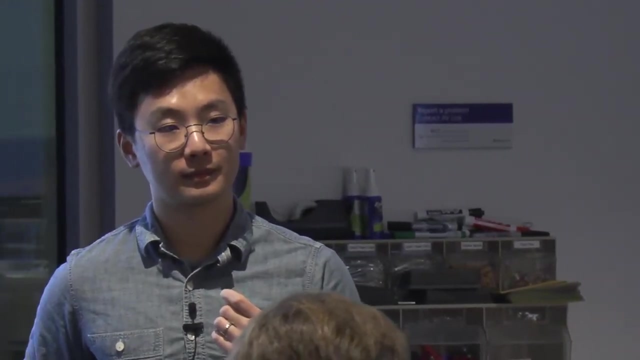 me that it actually does that computation instead of just returning some kind of garbage data. Right? Isn't there also a setting talking about threat models where, if you have a lot of interactivity, an actively malicious server could recover the key? 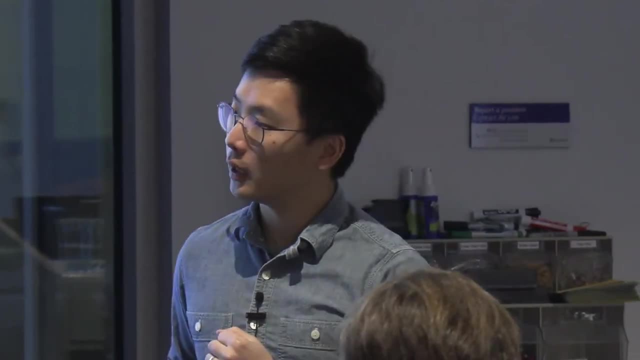 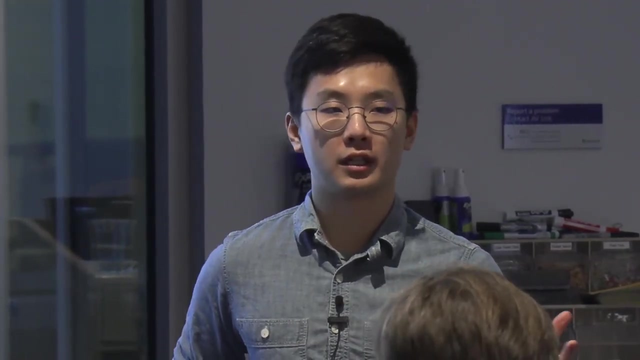 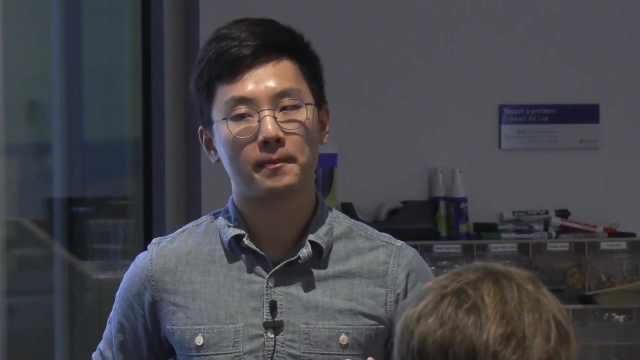 I remember something of that nature, right, Yeah, So, yes, So in the case where you have a lot of interaction and those interaction involve some client decrypting and sending back stuff, then if the server is malicious it could possibly try to kind of forge some ciphertext. 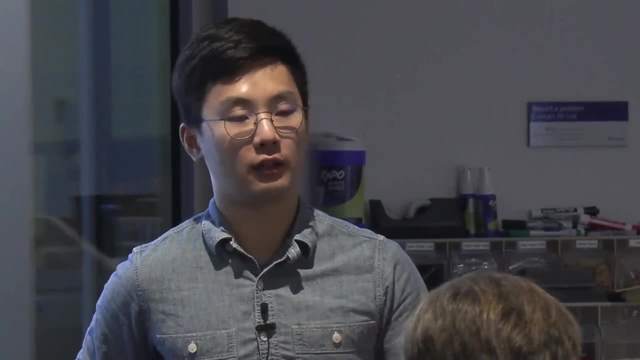 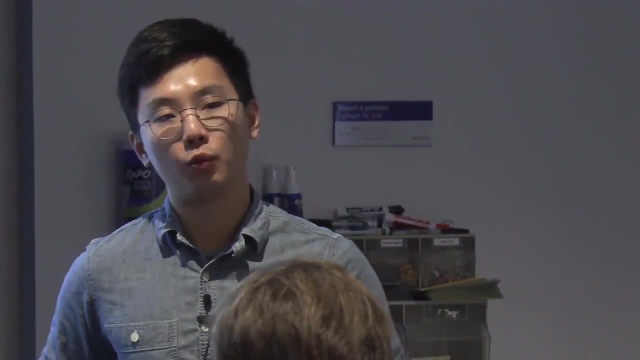 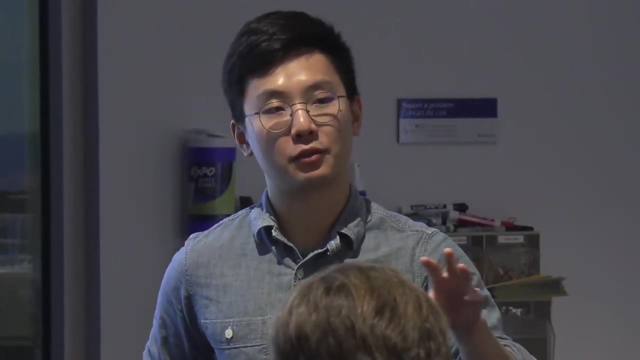 where it can learn about the key through the decryption. So yeah, So I think that's another valid point where we also need this kind of defend against the malicious servers. So if you can prove that the ciphertext you send to this secret key owner is generated through,